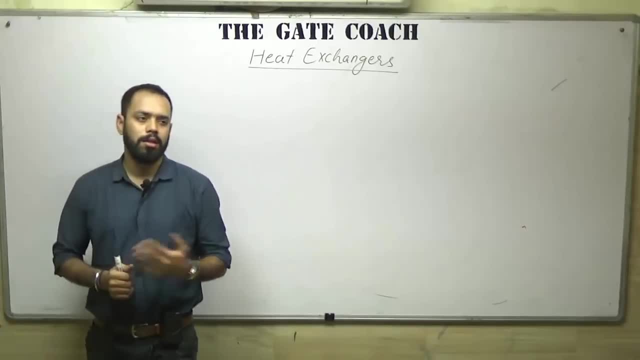 other PSU interviews are going to be held in this month or in the next month. So most of the students- as per our discussion with most of the students, because we are daily conducting some mock interviews- and we found that they are uncomfortable with this particular 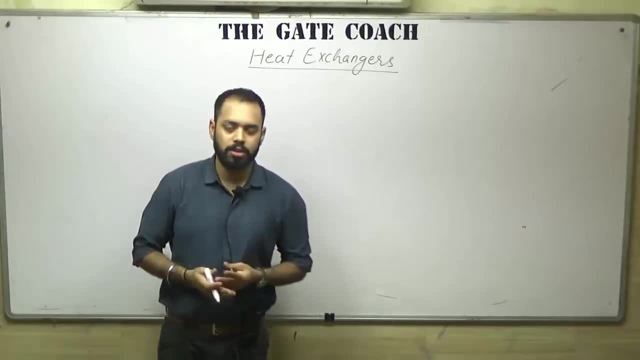 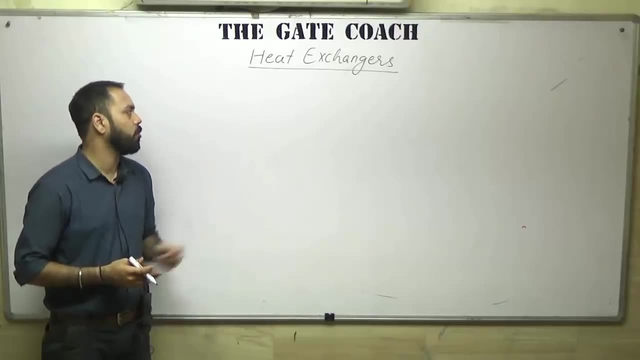 topic: heat exchanges. So, as per the request of all those students, we, the Gatecoach, are here with the most important topics for PSU interviews or for BARC interviews, that is, the heat exchanges. So let me make it clear that whatever I am discussing here about the 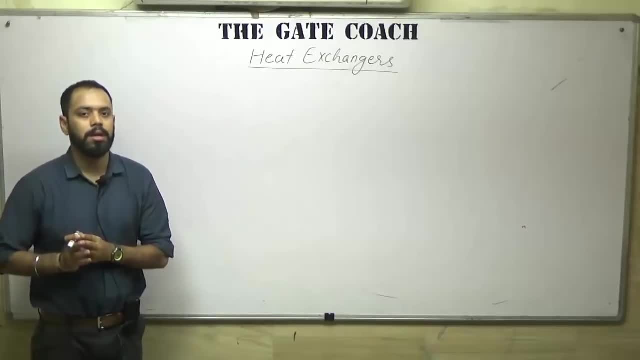 heat exchanger is specifically for interviews, This is not for gate examination, this is not for clearing gate examination or because I am not going to discuss the various formulas and various methods of calculation of areas. So in PSUs, when they are going to ask you, 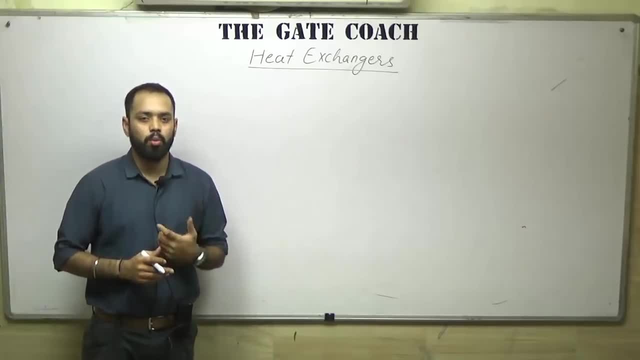 regarding heat exchanger, the questions will be based that what are the types of heat exchangers, In which condition we are going to use which type of heat exchangers? Let us suppose we are having the double pipe heat exchanger and the shell and tube heat exchanger. So 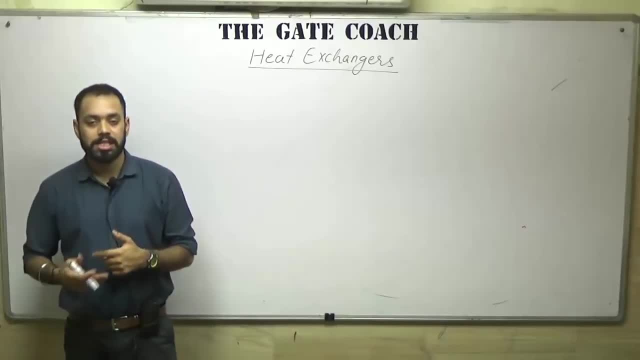 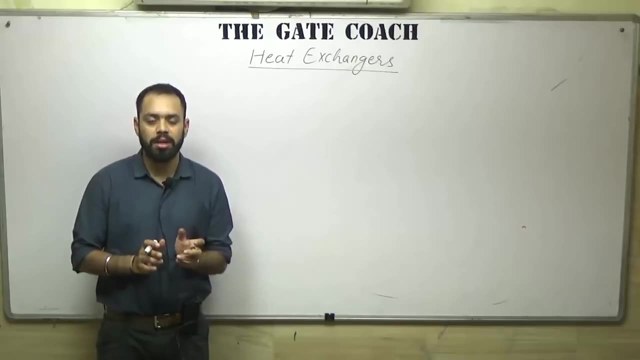 which exchanger is suitable for which purpose. We will use the exchanger in a counter current configuration or in a co-current configuration. How the number of tubes is calculated. What is the approximate diameter of the tube? What is theчеal of the board for each pipe Is? 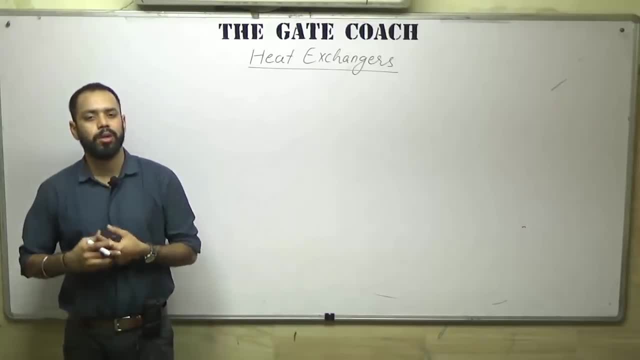 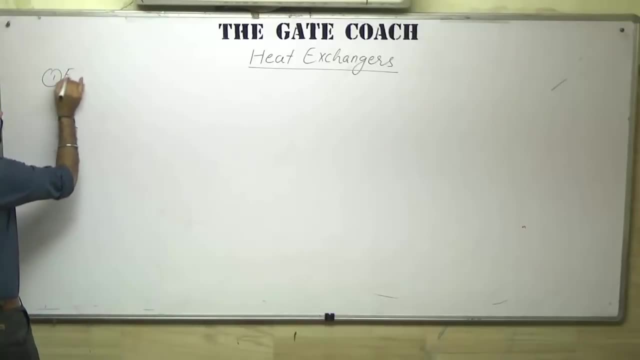 there a number of tubes in this tube. How many of the tubes are in that tube? How many of the tubes? So these kind of questions will be asked during the interviews. So, one by one, I am going to discuss these things. First is so, what is a exchanger or a heat exchanger? Why it is used. 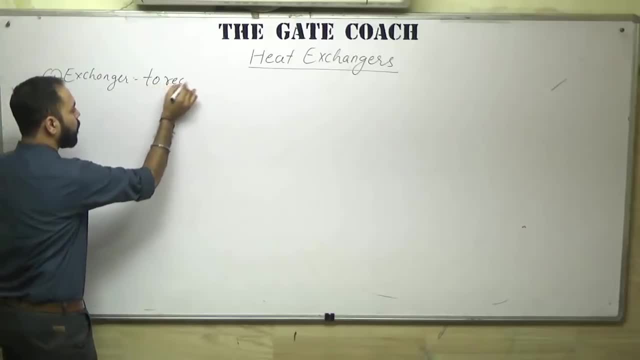 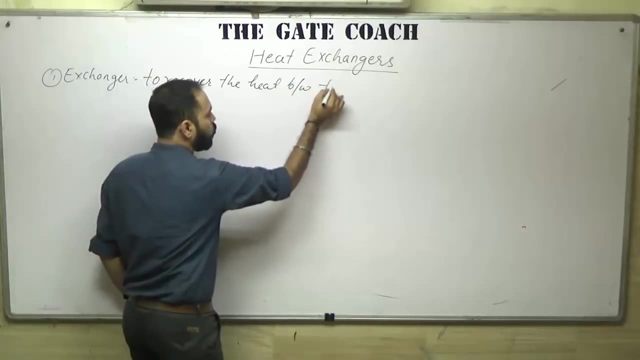 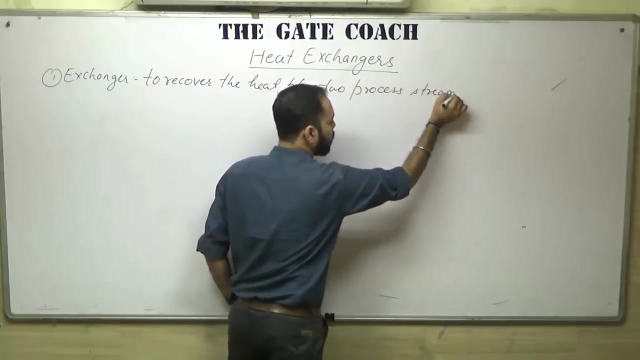 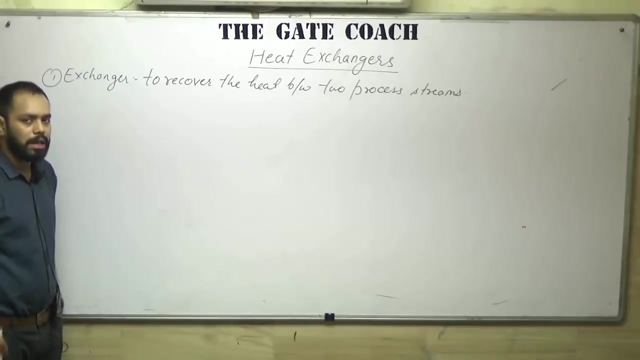 A heat exchanger is used to recover the heat between two process streams, to recover the heat between two process streams in any process. So there are different terms which are used or there are different types of heat exchanger. We have different names. Another term is a heater, So when we say a heater, 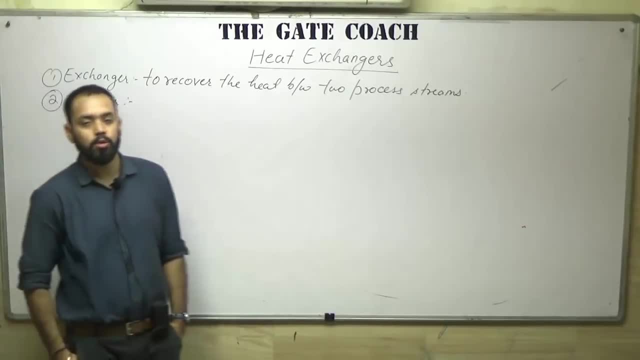 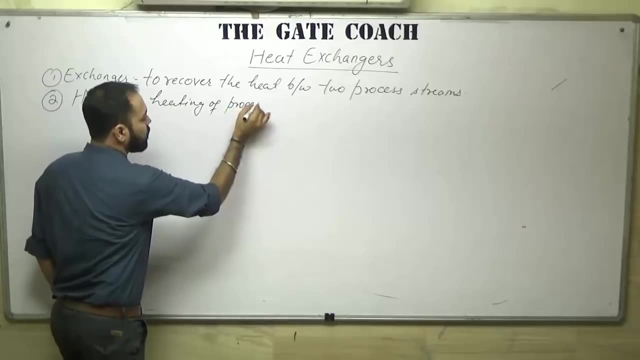 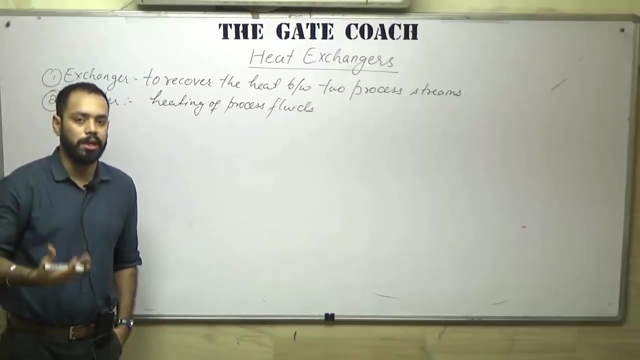 it is a heat exchanger, but a heater is specifically used for heating of process fluids. Heating of process fluids. What is the meaning of process fluid? Process fluid is that stream which we want to heat, And when you want to heat a process stream, we should have a heating medium. 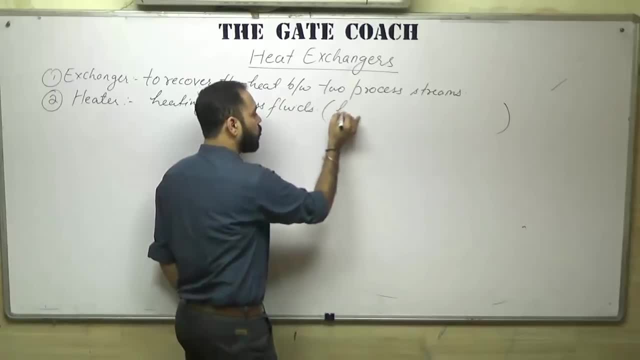 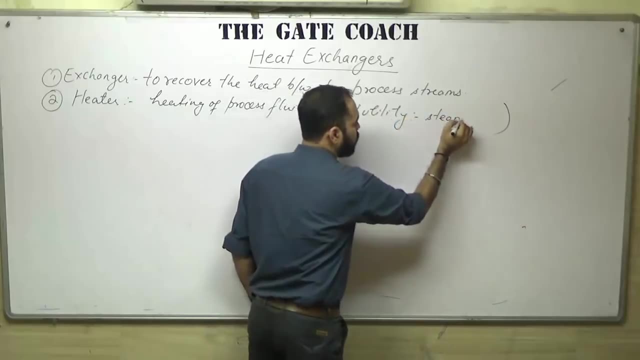 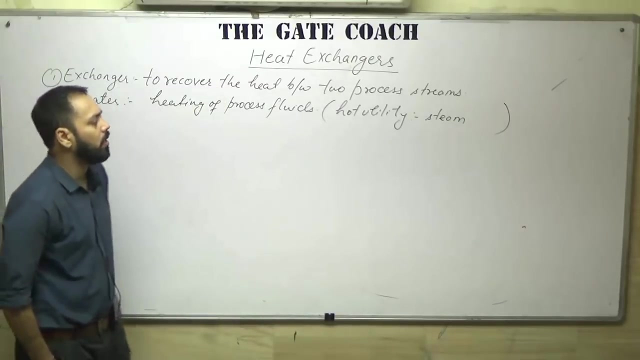 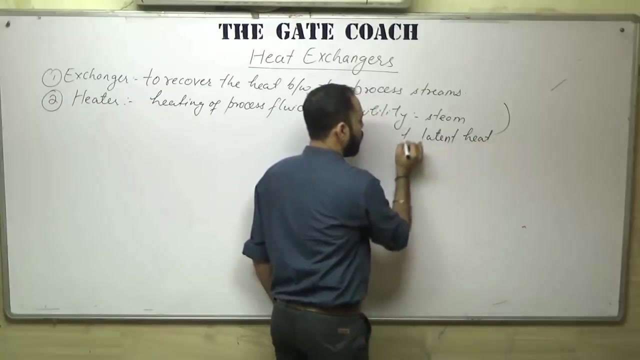 That heating medium is also called hot utility, And generally this hot utility is steam. Generally we use steam as the heating medium. okay, so steam has a very high latent heat content. actually, it has very high latent heat content, very high latent heat content, and therefore it is suitable for heating of. 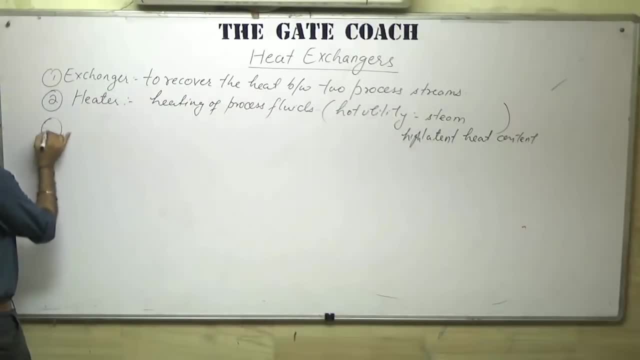 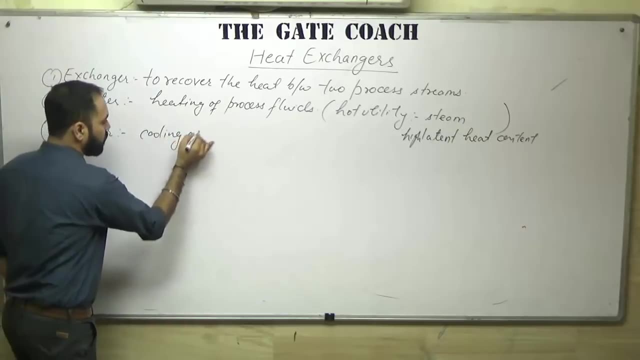 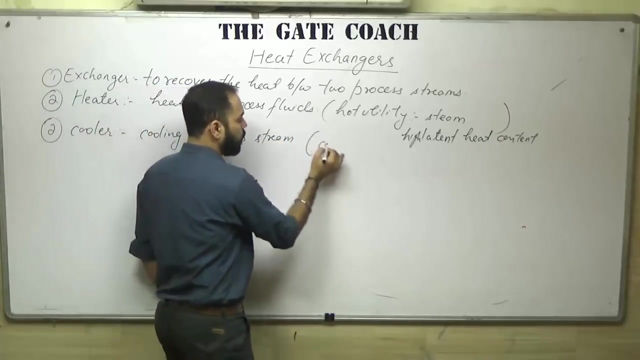 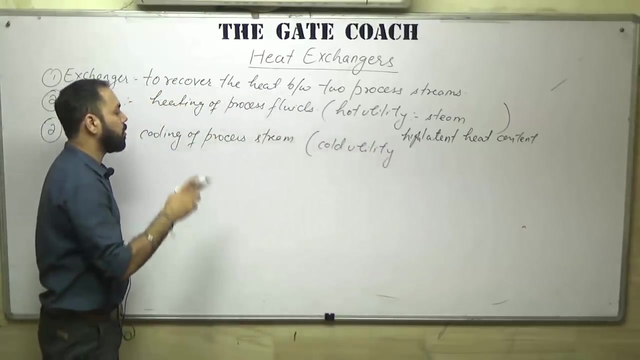 process streams. another term that is used in process industries is a cooler. so what is a cooler? cooler is used for cooling of process stream, and when you are cooling a process stream, there should be a cold utility. what is the meaning of cold utility? the stream, which stream means the 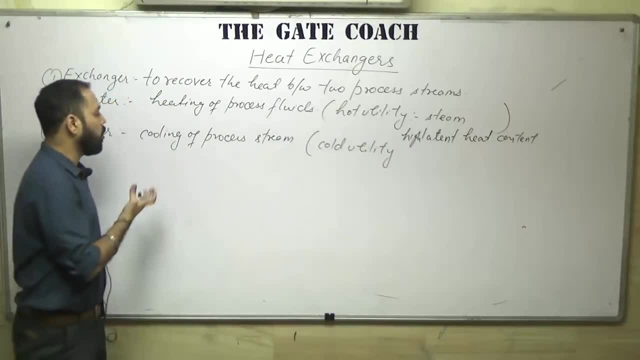 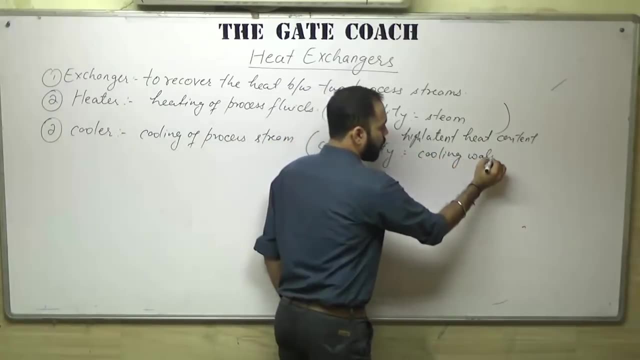 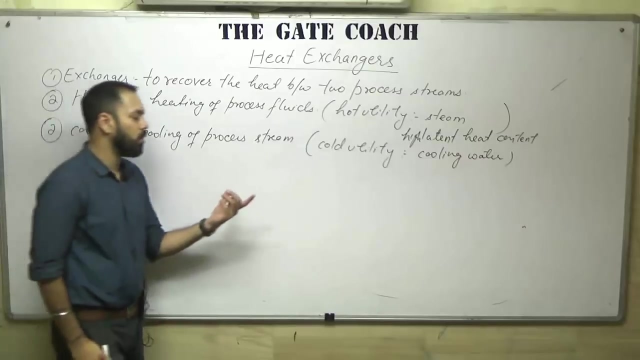 other stream apart from the process stream which i am using to cool this process stream, that cold utility is the cooling motor. so so now, sometimes the interviewer will ask you that cooling water which i am using here. generally this cooling water is present at the room temperature, let us say, 25 degree celsius or 30. 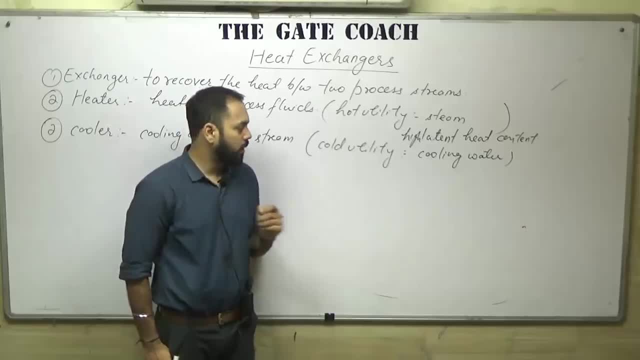 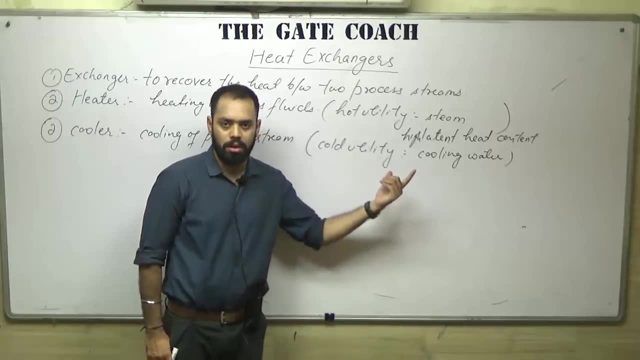 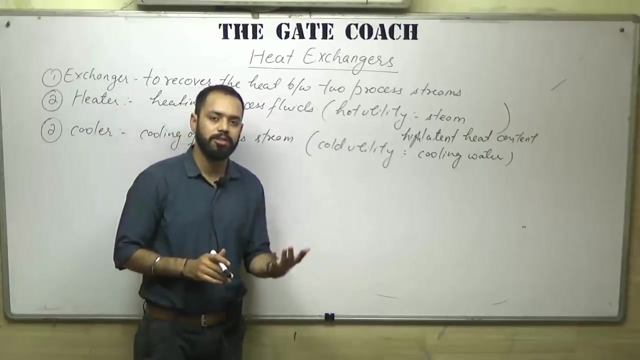 degree celsius. so if the interviewer asked that, can we use atmospheric air for cooling purpose instead of cooling water? so what should be the answer? see, first thing is, if you want heat transfer to take the air out of the process stream, then you have to take the air out of the process stream. 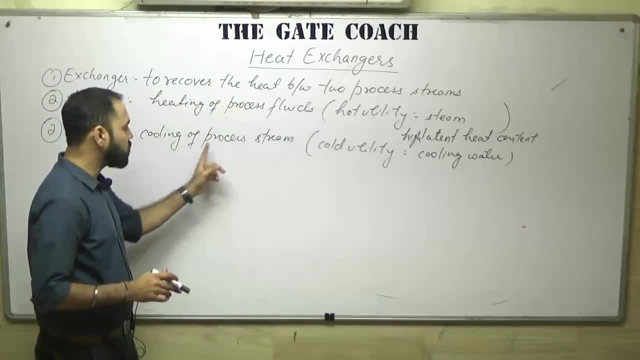 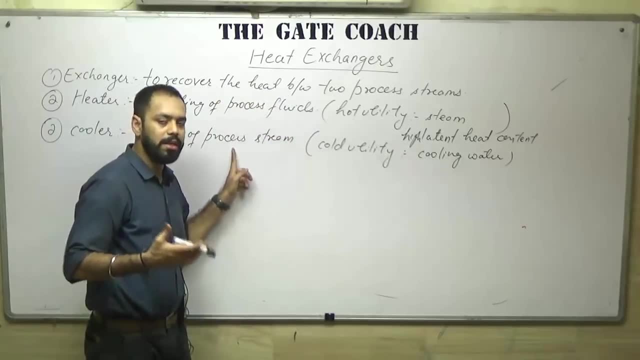 and you have to take the air out of the process stream and you have to take the air out of the process stream. let us suppose i am cooling a fluid, so the process stream is a hot fluid and the cooling water is the cold fluid. if a process stream is at a temperature of, let us say, 80 degree celsius and you want heat transfer to, 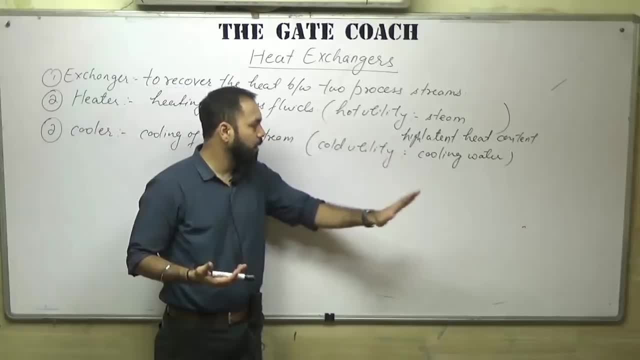 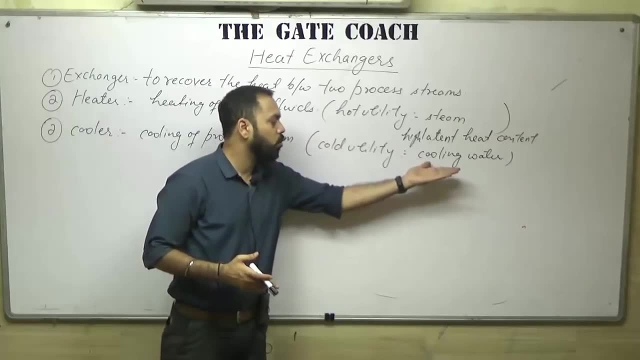 take place from the process stream to the cooling water, then definitely cooling water should be below 80 degree celsius. then only heat transfer can take place. so i can use atmospheric cooling water- let us suppose 25 or 30 degree celsius cooling water- to cool this hot process stream. 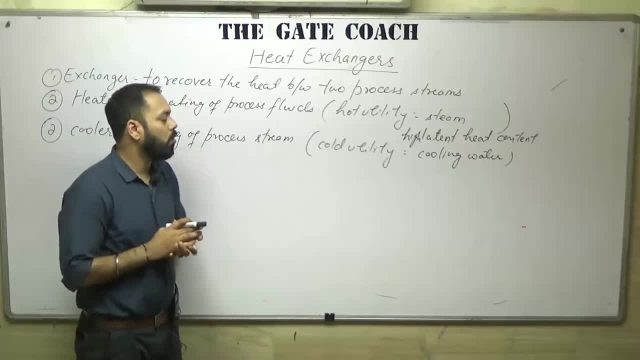 so there must be a temperature difference. okay. now if the question is: can we use atmospheric air to use this stream? of course you can use. okay, atmospheric air should be can be used provided the temperature of the atmospheric air should be less than the temperature of the process stream. 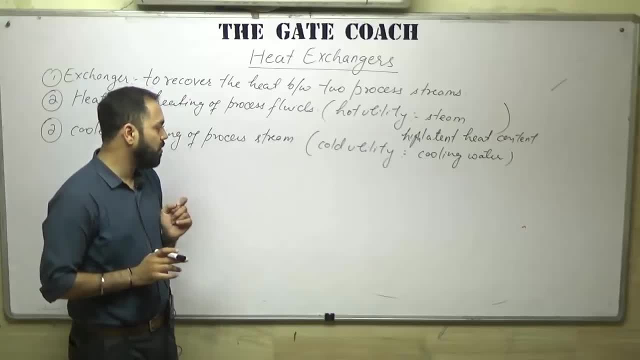 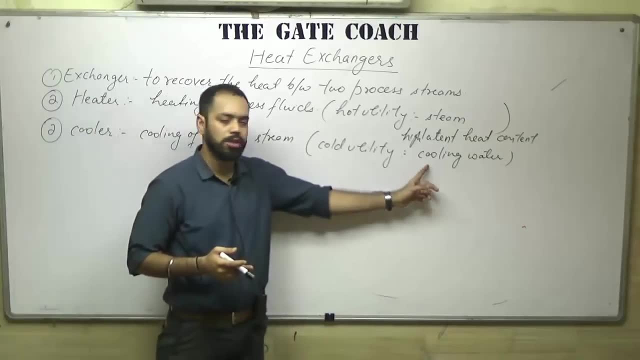 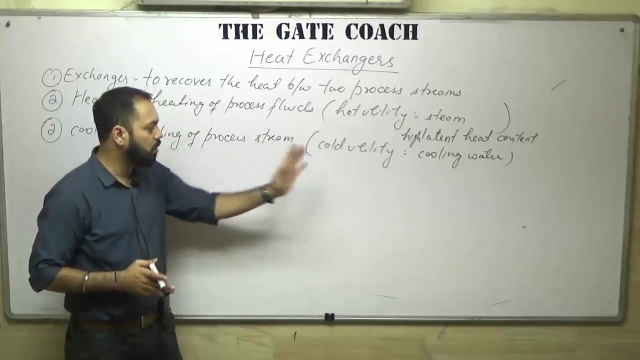 but then there will be a problem. what is the problem? the problem is the heat transfer coefficient of atmospheric air is lesser, much less than the heat transfer coefficient of cooling water. and if the heat transfer coefficient is less for the same heat duty, if you are using cooling air. 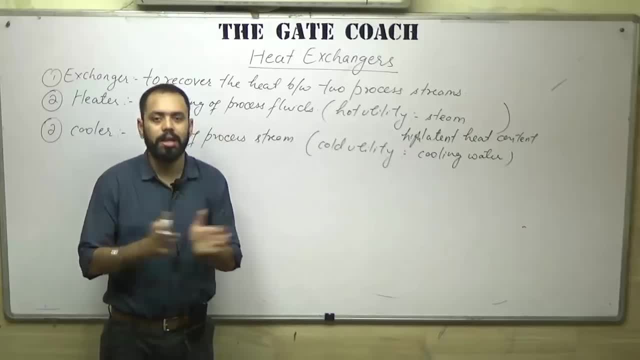 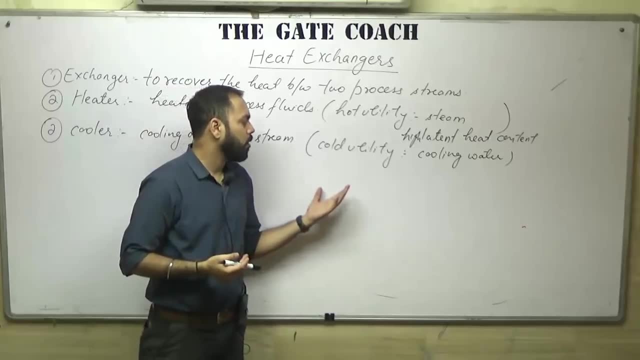 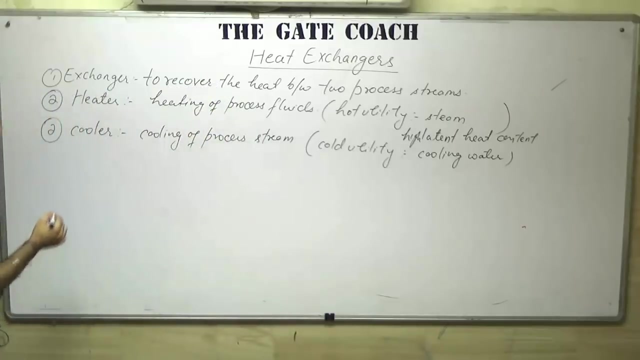 instead of cooling water. the heat transfer area will be very large and therefore the size of the heat exchanger required will be very large. so therefore, most of the time to save the cost, we use cooling water instead of cooling air in any cooler. okay, next is: this is third. fourth is condenser. 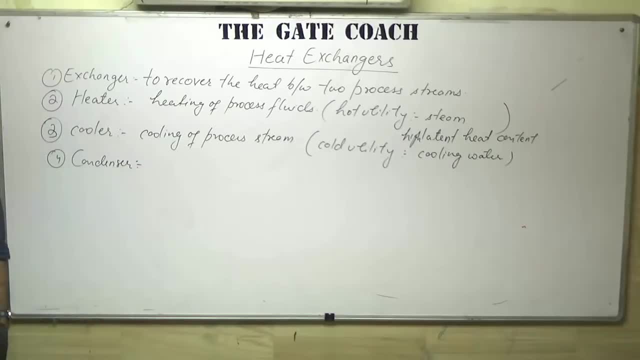 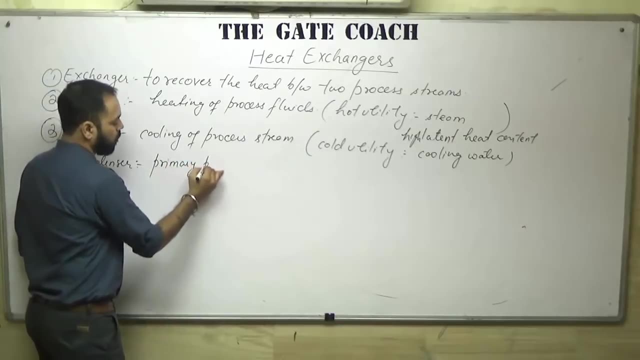 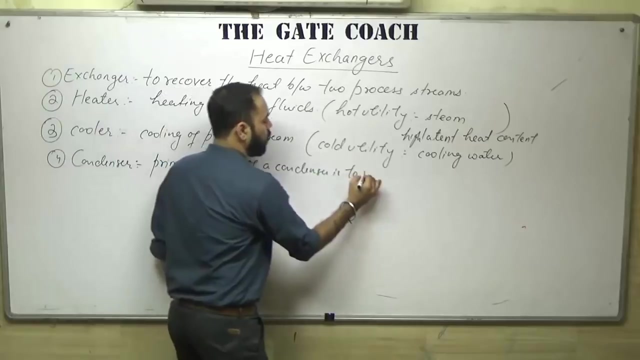 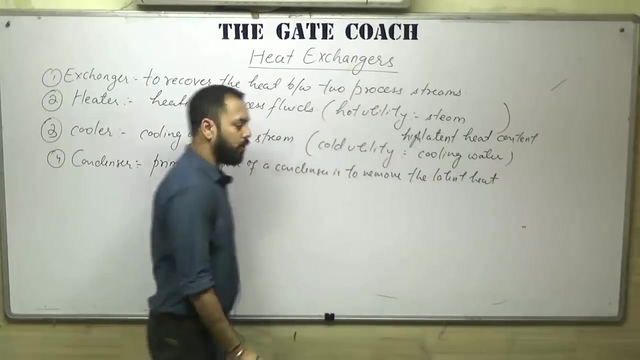 so what is a condenser? there is a difference between cooler and a condenser. what is a condenser? its primary purpose, the primary purpose of a condenser is to remove the latent heat. it means when a process stream enters the condenser. if it is present in the vapor form, it 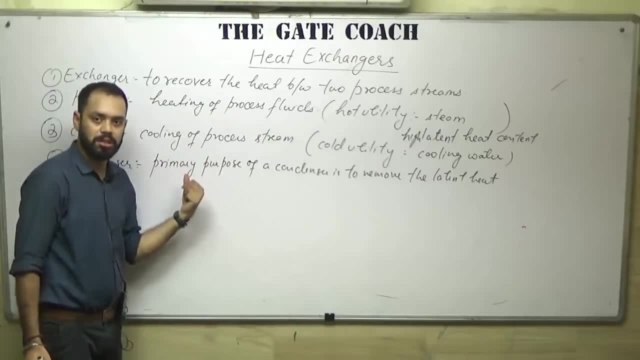 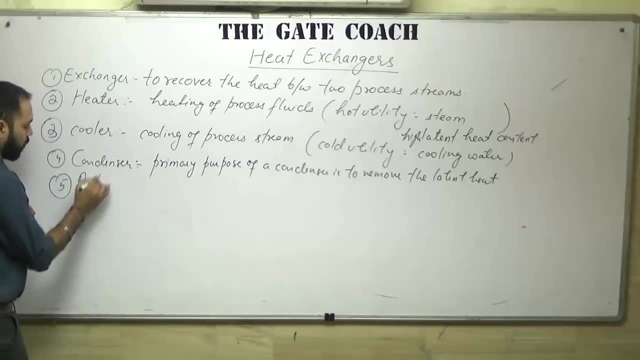 will be condensed once it enters the vector form. then when it enters the vapor form, it becomes condenser. So the phase of the process stream will change, while in case of cooler, only sensible heat change is there. similarly, there is a reboiler. so what is the purpose of a reboiler? the primary 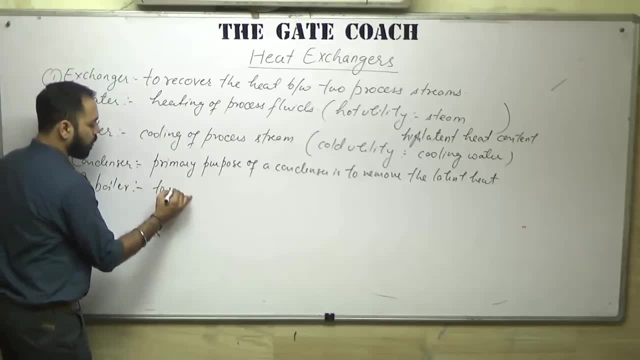 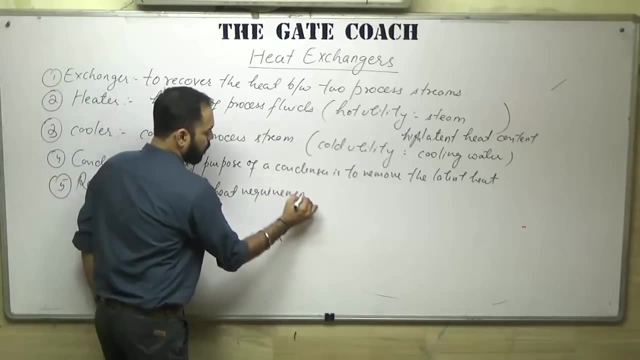 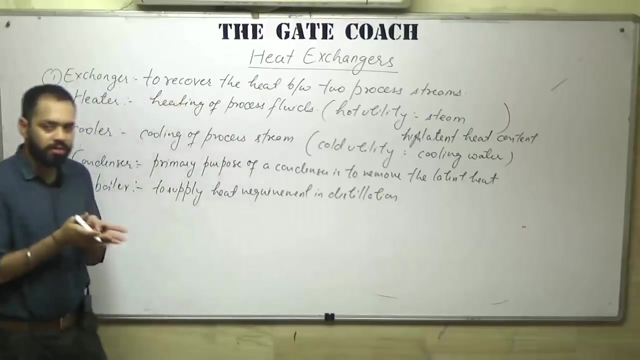 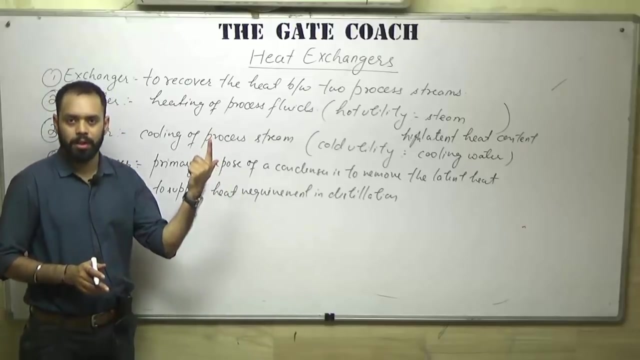 purpose of a reboiler is to supply heat requirements in distillation. what reboiler does? from the bottoms of the distillation column, the liquid is fed to the reboiler. okay, now that reboiler evaporates the liquid and most of the time that reboiler is a partial 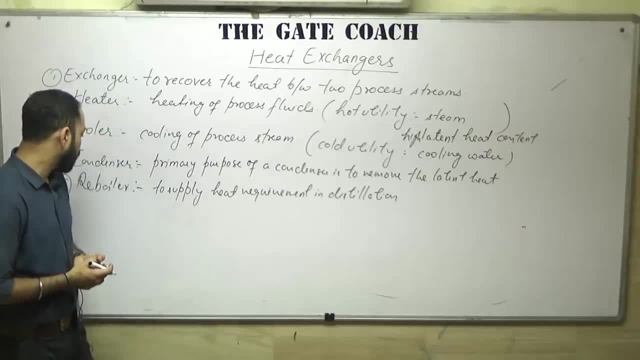 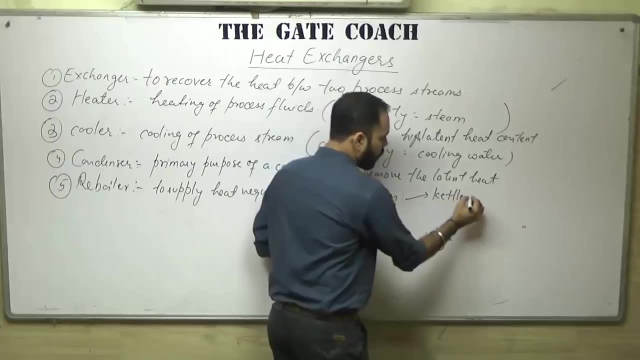 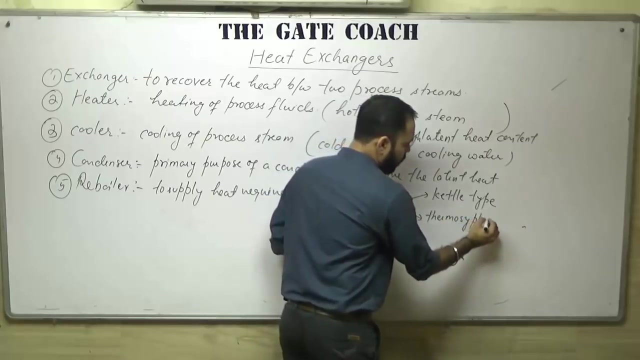 reboiler, so partial evaporation takes place in that. Okay, now for the point of interviews. I am telling you that there are two types of reboiler: the kettle type and the thermosyphon type. so you must have studied that there are two. 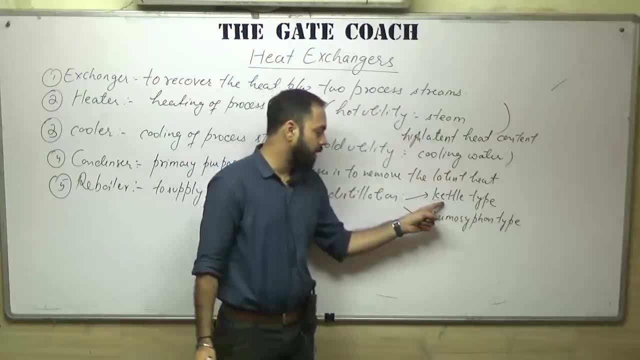 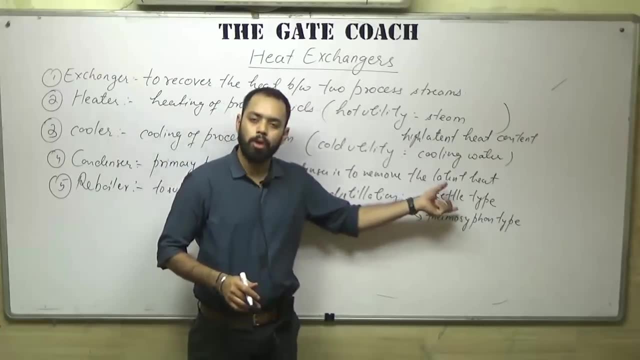 types of reboiler. so go through the details of kettle type and thermosyphon type reboiler. what is the detail? detail means in which configuration kettle type reboiler is used, horizontal or vertical. In which configuration thermosyphon reboiler is used, horizontal and vertical or vertical. 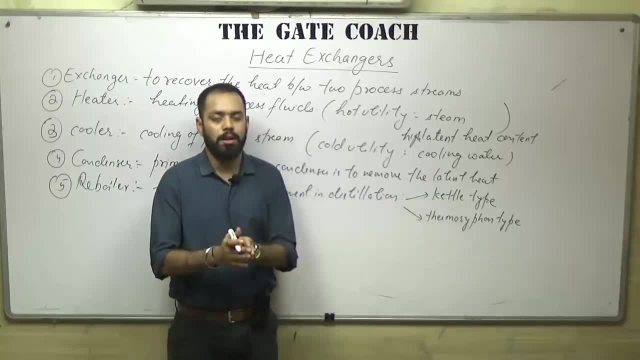 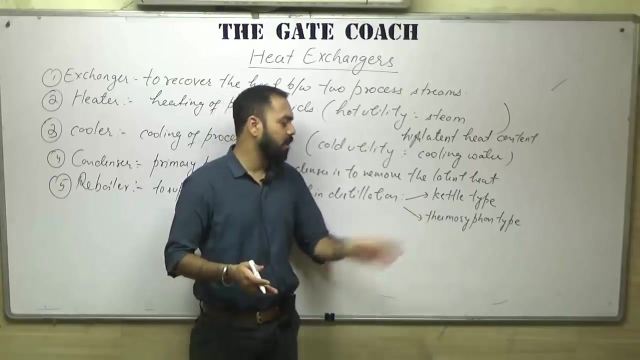 okay, what is the basic difference between the principle of functioning of kettle and the thermosyphon reboiler? so if I ask this question to students, they say that, sir, we consider kettle type as a partial reboiler and therefore it will be considered as a stage, while a thermosyphon type 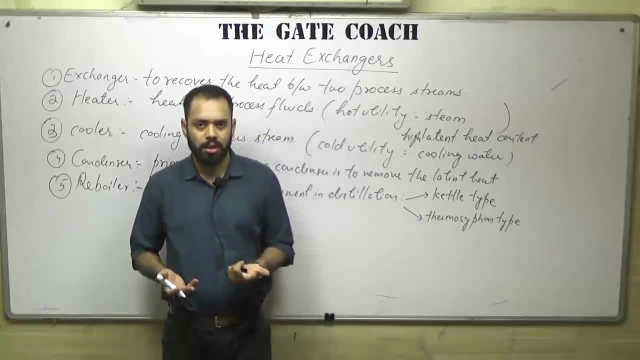 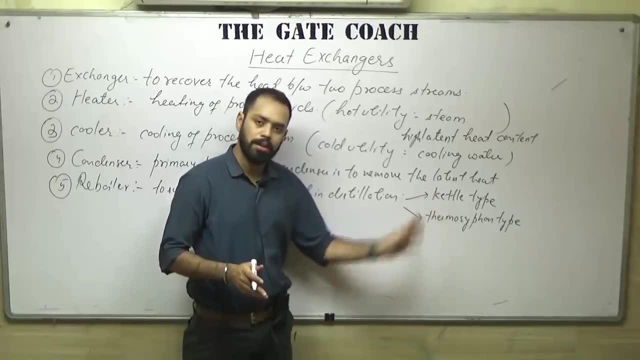 reboiler is a total reboiler, so it will not be considered as a stage. okay, that's true, but I'm talking about the basic difference between the function of kettle and the thermosyphon reboiler. okay, so you can go through standard books like Richardson and Coulson and you. 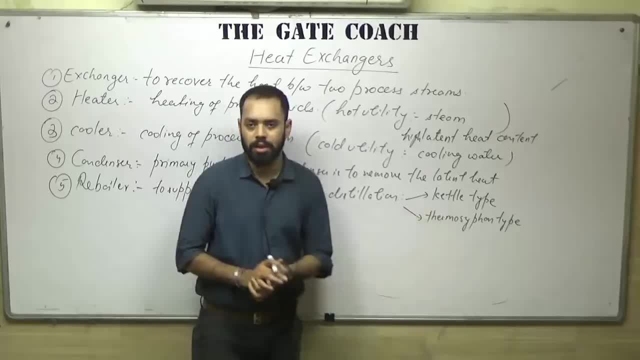 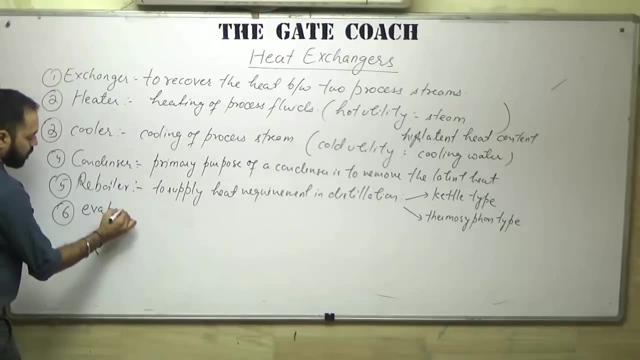 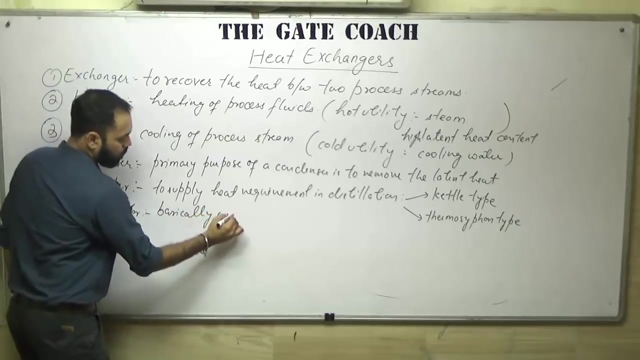 can read a paragraph or two paragraph about the kettle or the thermosyphon type of reboiler. okay, the next thing where a heat transfer process takes place is called evaporator. so what is the function of a evaporator? evaporator is basically used to concentrate the heat. 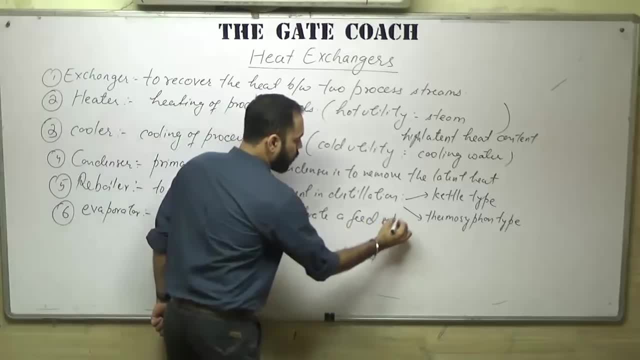 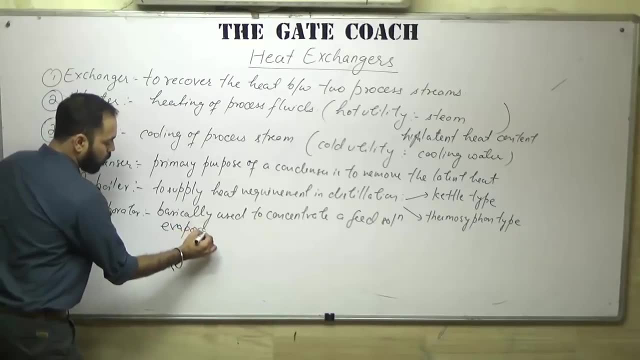 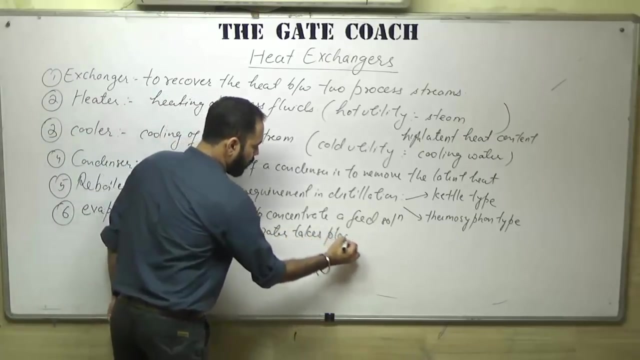 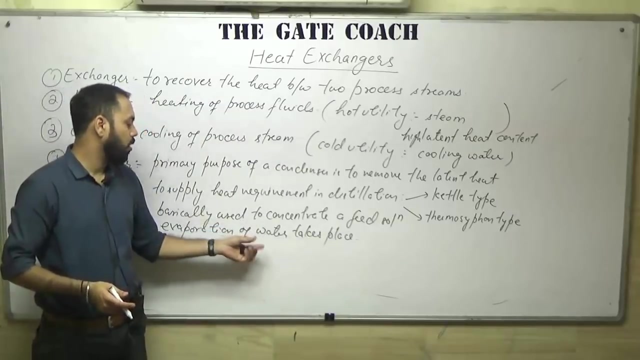 into a feed solution and therefore, in case of evaporator, evaporation of water takes place. evaporation of water takes place, okay, if any other fluid, let us suppose, apart from water, if you have any different kind of fluid which is getting evaporated, So that is the type of liquid that can be evaporated. 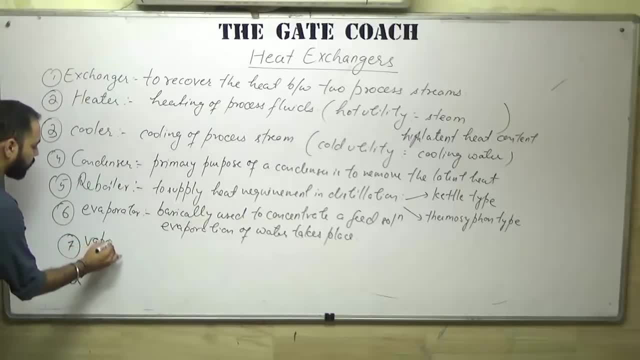 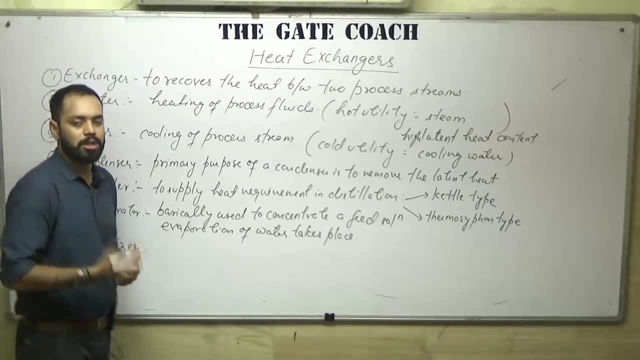 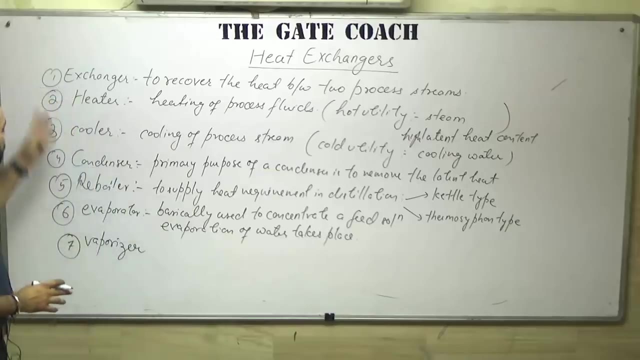 Okay, Yeah, known as a vaporizer. so what is the difference between then evaporator and a vaporizer? the difference is: in case of evaporator, the evaporation of water takes place. in case of vaporizer, evaporation of any other liquid takes place. ok, so these are some terms, some devices which 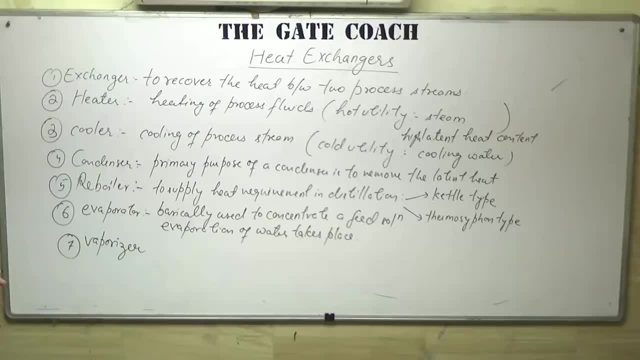 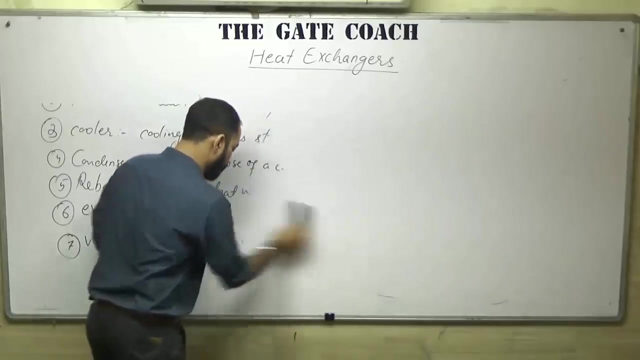 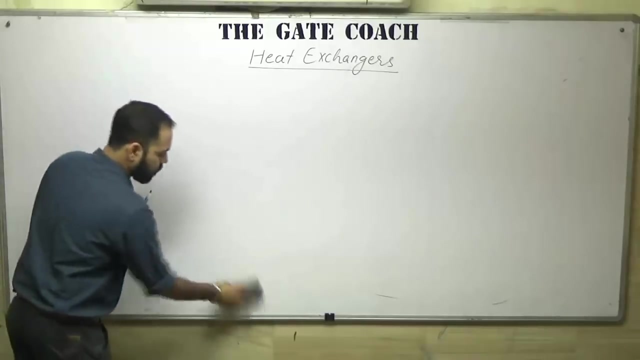 are used in process chemical industries. ok, so we should have the knowledge that how these terms are different from each other. these things are asked in the interviews, ok, so i think this is clear to you. ok, now the next part is: what are the types of heat exchangers? 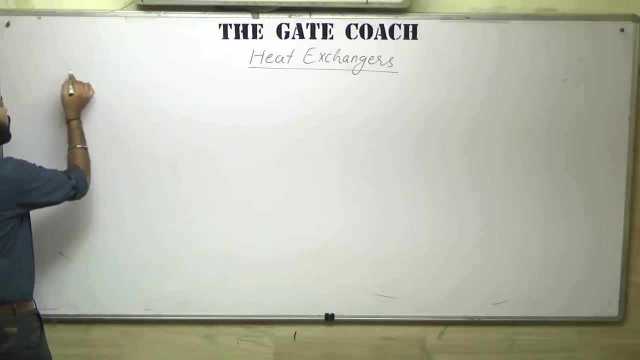 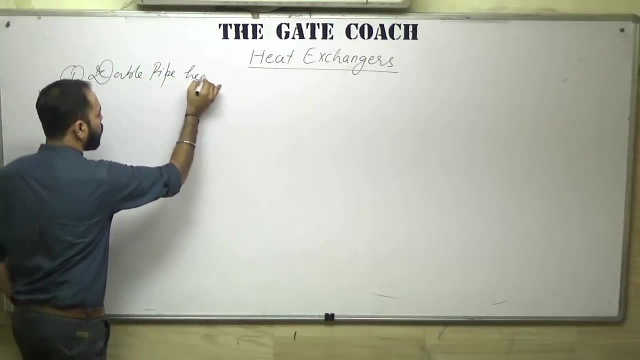 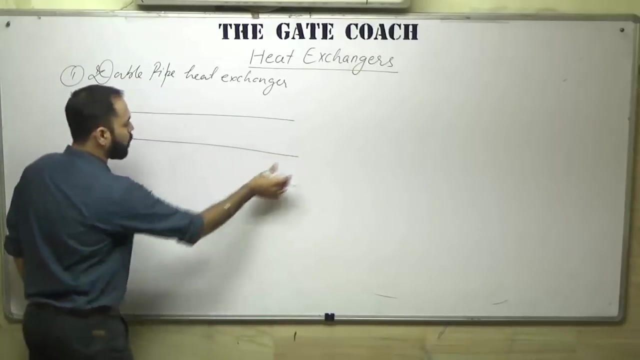 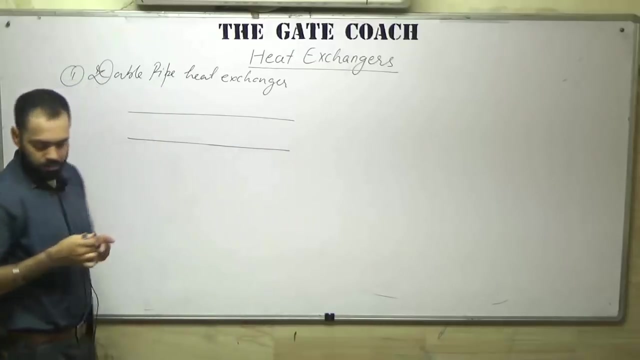 so the major types of heat exchanger. so the major types of heat exchanger. the first one is the double pipe heat exchanger. what is the double pipe heat exchanger? it's a very simple kind of heat exchanger. there are a set of concentric pipes. so this is the outer pipe. ok, there is a inner pipe. 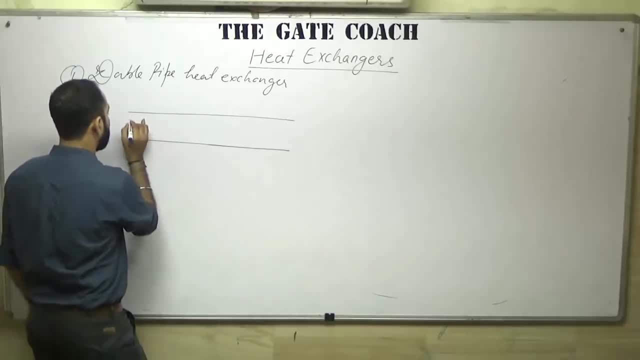 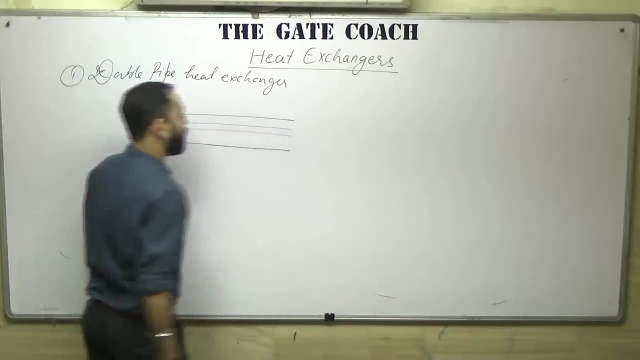 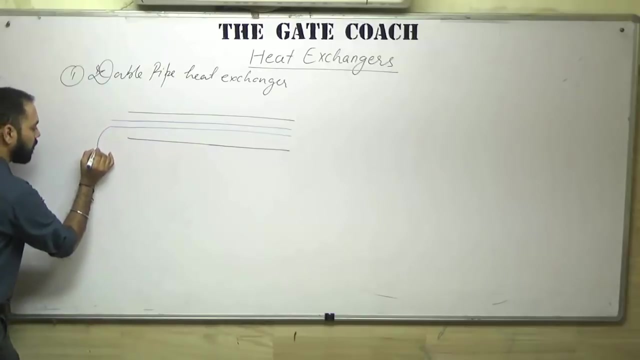 the outer pipe and there will be an inner pipe right. so this pipe extends from the main region. then there is a bend like this, which is called the u bend, and then it goes into another bigger diameter pipe. so this is the inner pipe, right? so this is the inner pipe. 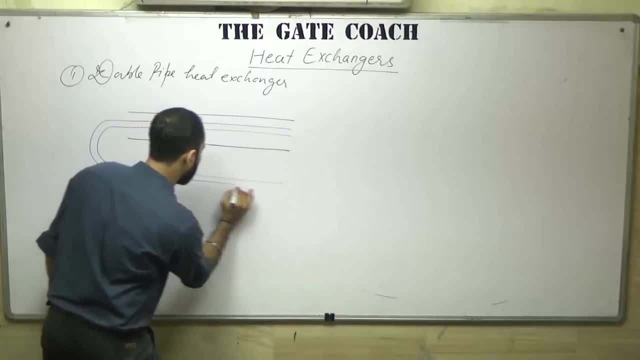 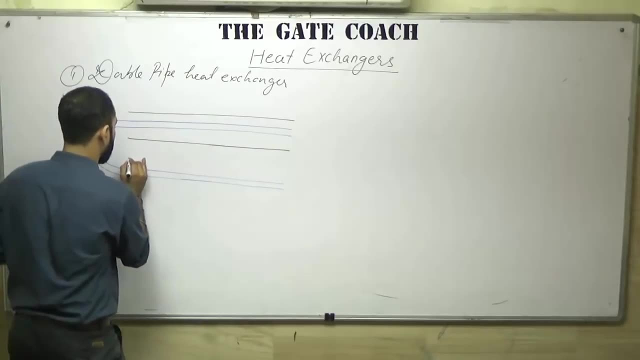 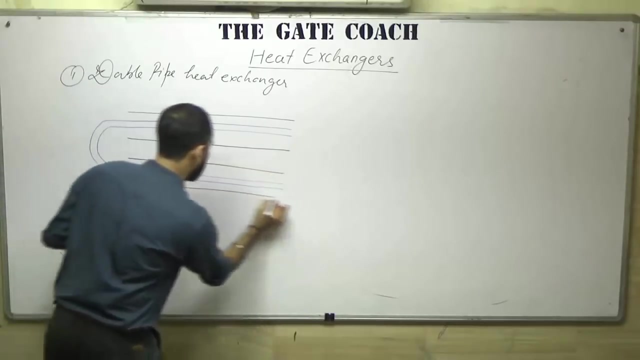 right… ok, so the outer pipe… so this is the outer pipe, right… and the inner pipe… so the inner pipe. now, if you just consider the space around the inner pipe, of example, if you consider the space around it, this will be 2 Baby ну and it will be 9 Baby Yo. 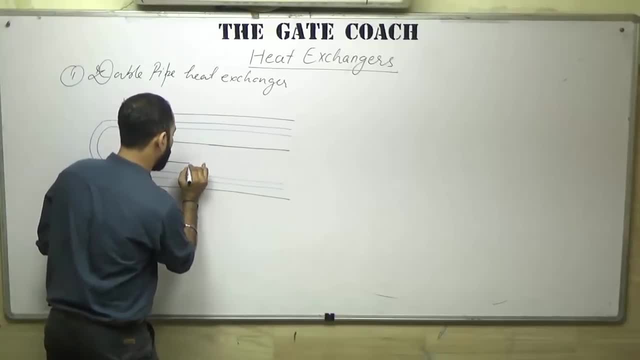 so this is the other and the inner pipe. this is the same constructionine used for internal pipe. sayzai, you can look at the typical pedals. OK, so this is the other vibrate syrup is. Спасибо, massagearis beam, it will be right here easily. ok, then you will, being to ends of the pipe. 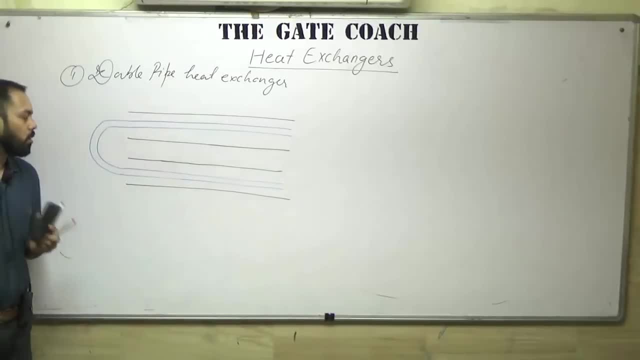 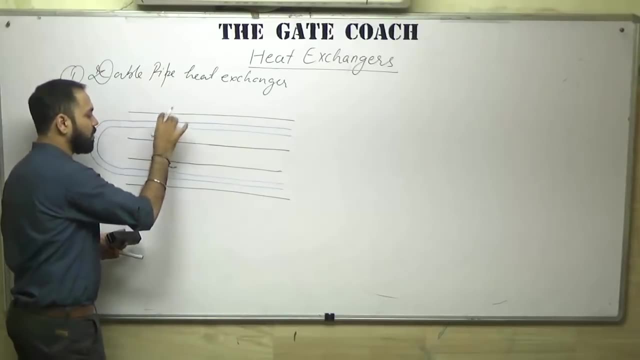 so much is needed here, even during the process of electrical inverse, the installation of a double pipe heat exchangers. I am not showing all the components. There are a lot of joints. This inner pipe, if you want to hold this inner pipe inside this outer pipe. 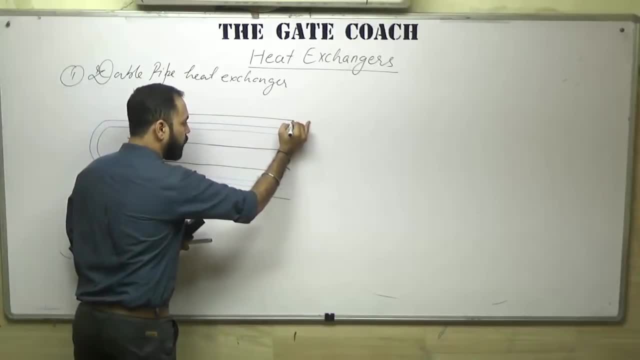 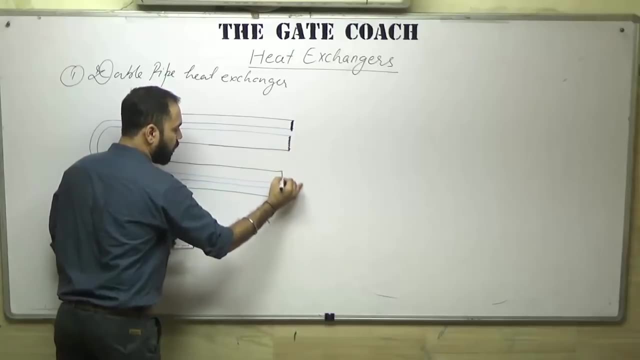 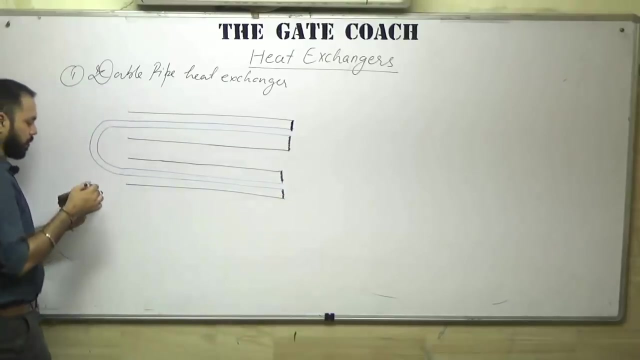 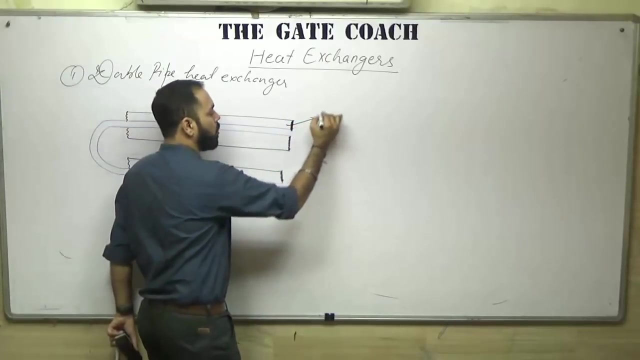 then at this point there must be some arrangements made so that this inner pipe will remain like this. So I am not considering those detailed construction that is not required for the purpose of interview. So the region, this particular region, this region is called the. 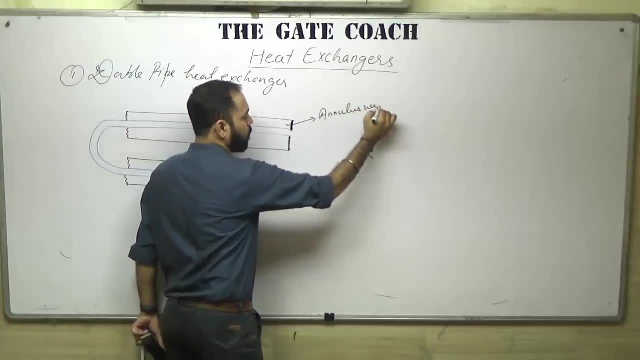 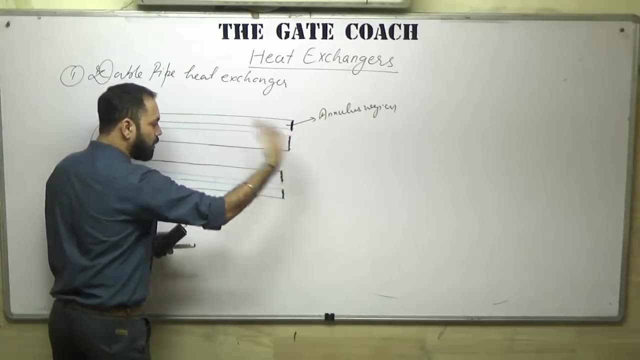 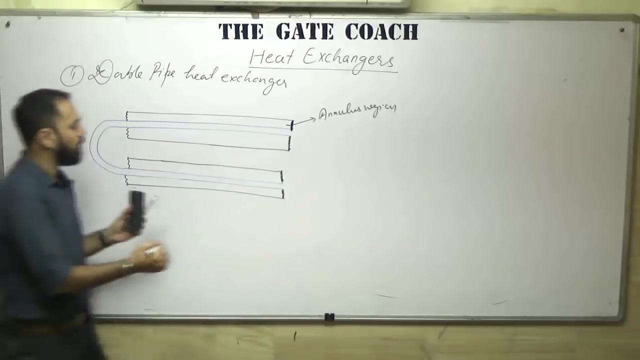 annulus region. So there are two process streams. One of the process stream will travel in this annulus, while the other process stream will travel in this inner tube. This set is known as one hair, So in a double pipe heat exchanger we use this term: hairpin. What is the meaning of? 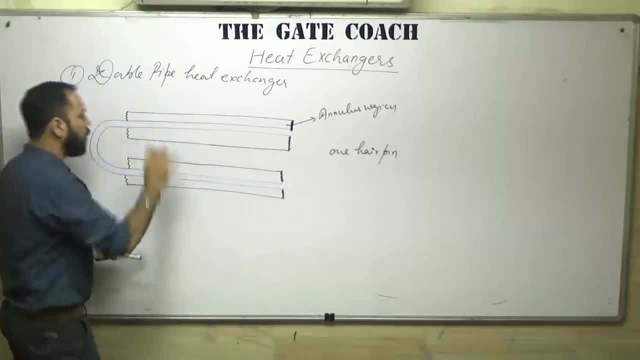 a hairpin. This one set is known as hairpin. This set is known as one leg of the hairpin. This one is the other leg of the hairpin. So what is so special about the double pipe heat exchangers? If the question is in which? 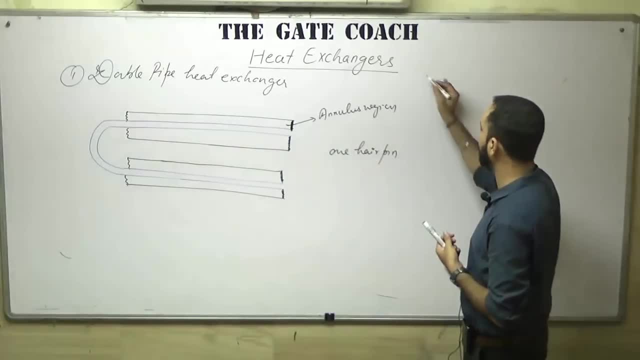 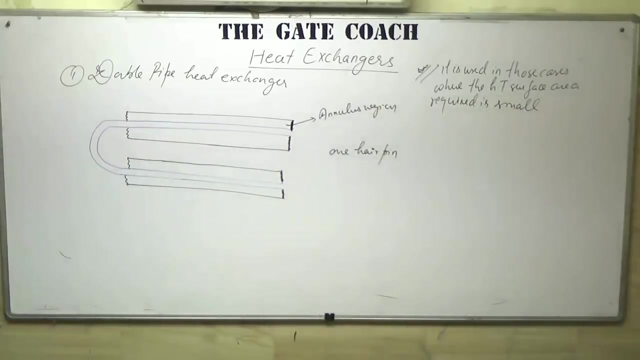 case, double pipe heat exchangers will be used. So let us write few points regarding double pipe heat exchanger. The first point is it is used in those cases where the heat transfer surface area required is small. So that is the use, and that is also the limitation, of this type of heat exchanger. 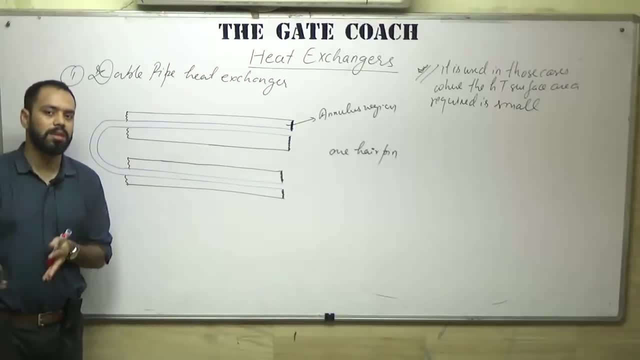 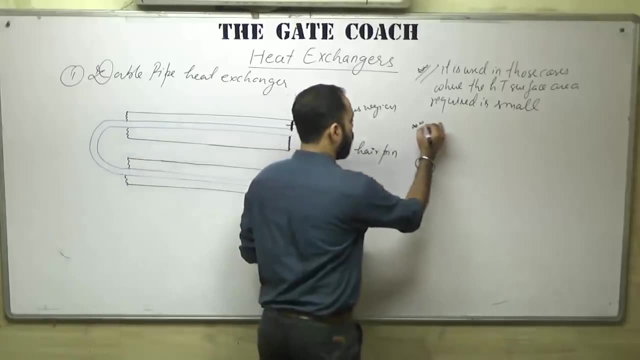 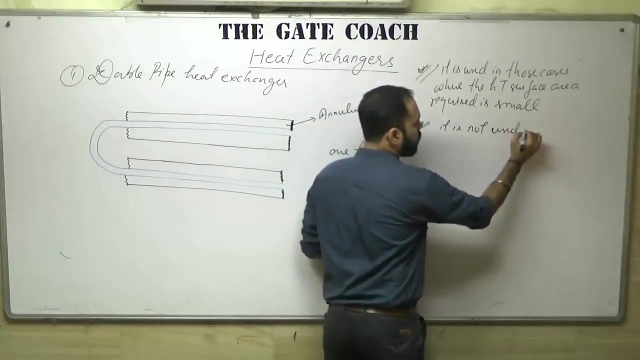 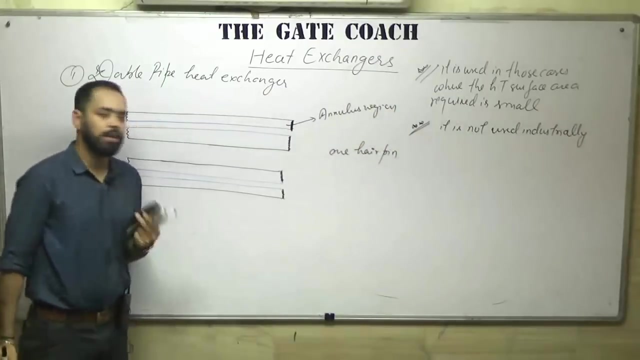 We cannot use this double pipe heat exchangers in those cases where the area required for heat transfer is very large, Because in that case it is not used industrially. It is not used industrially why? Because generally in industries the heat transfer surface area required is very large. 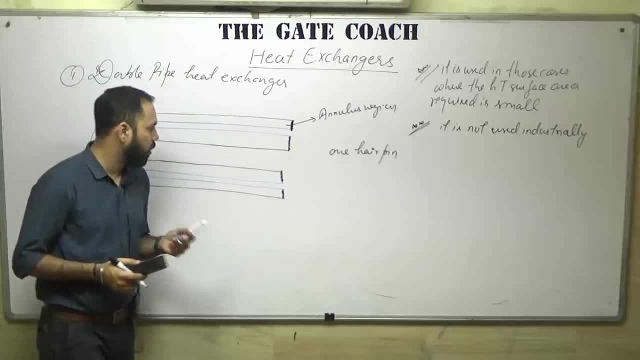 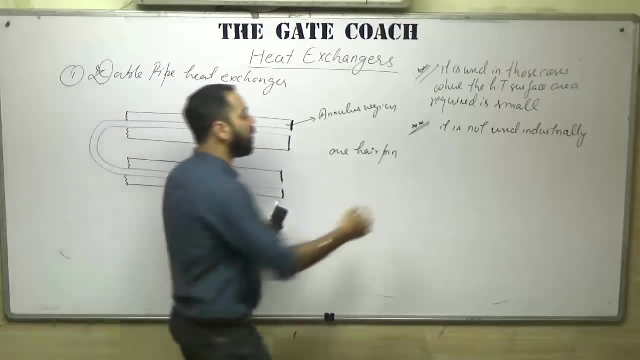 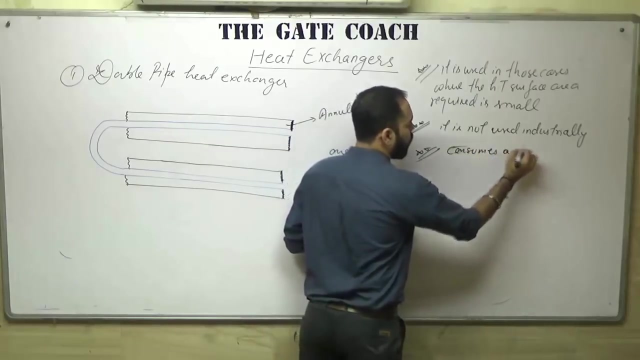 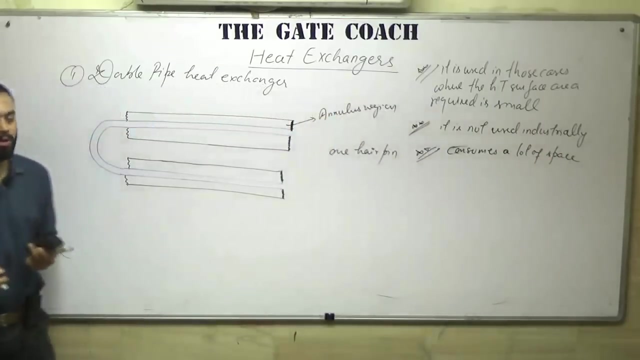 And if you want to provide that much of heat transfer, The number of hairpins will increase, And to accommodate that number of hairpins we will need a lot of ground space. So it consumes a lot of space. It consumes a lot of space. 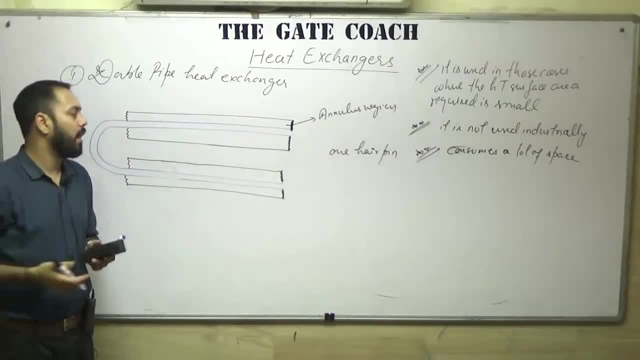 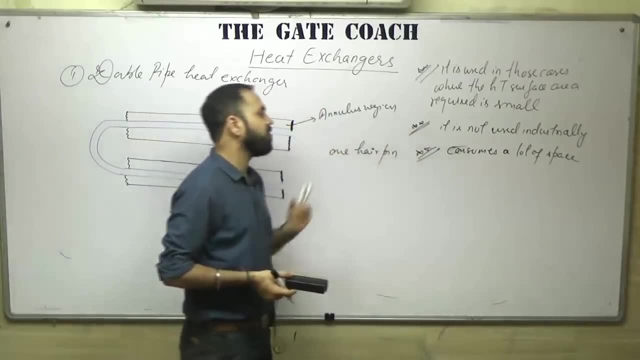 Because if you are going to use this for industrial purpose, in that case usually what happens in industries: The value of heat duty is very small, So it consumes a lot of space, But in that case the number of hairpins is very high, due to which the heat transfer surface. 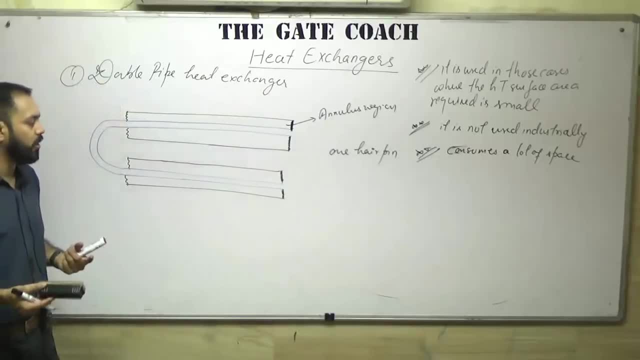 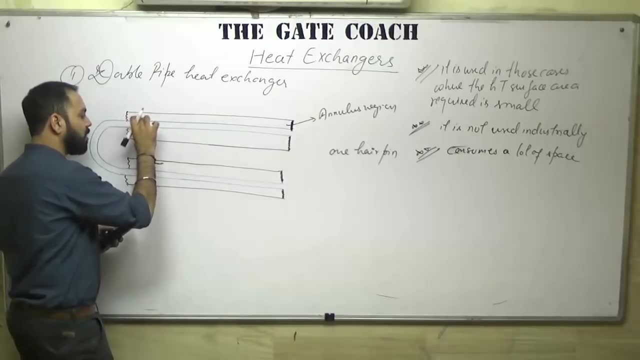 area required is very high And if you want to provide that much of heat transfer surface area, What is the heat transfer surface area In one leg of this hairpin? this is the surface area, The surface area of this inner tube right. This upper surface area of this inner tube is the surface area where heat transfer is. 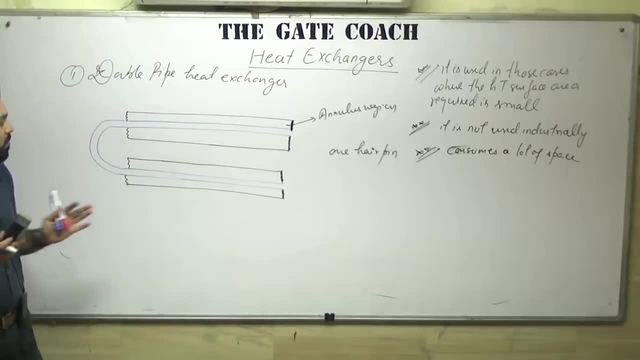 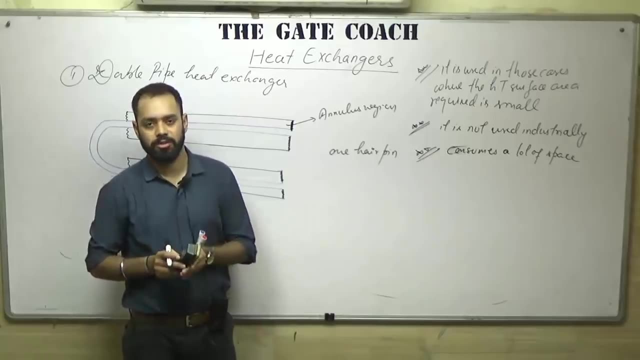 taking place And if you want to provide very high surface area, in that case you will have to increase the number of hairpins, which is going to consume a lot of space. So that is not economically feasible for us. so they are not used industrially. what are the advantage of these double? 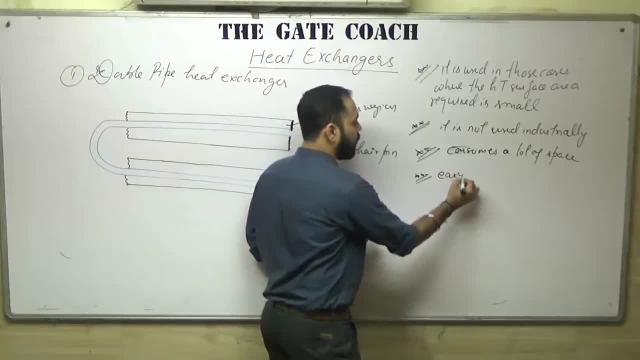 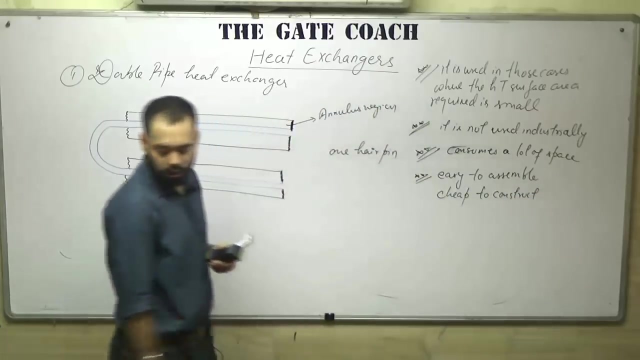 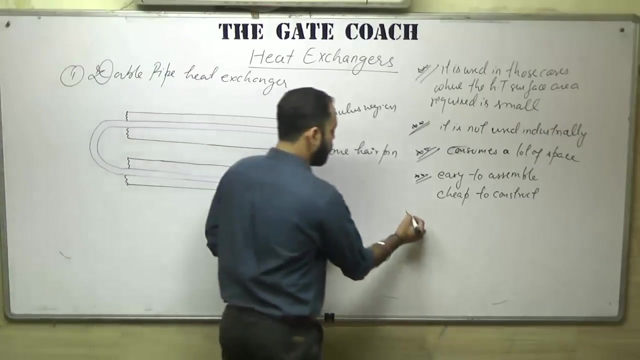 pipe heat exchanger. the advantages: it is easy to assemble- okay. secondly, it is cheapest. or you can say it is cheap to construct. this is the advantage of this type of heat exchanger, okay. another problem with this type of heat exchanger is- let us suppose you are saying that I am increasing the number- 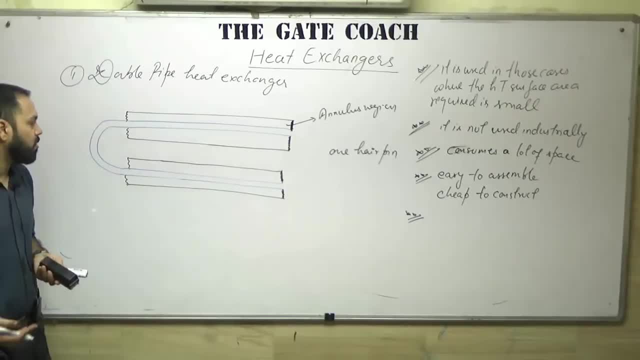 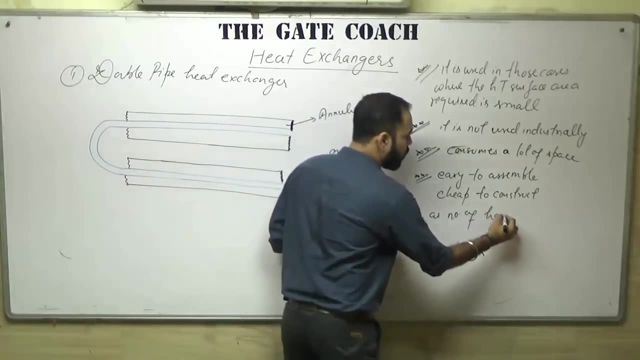 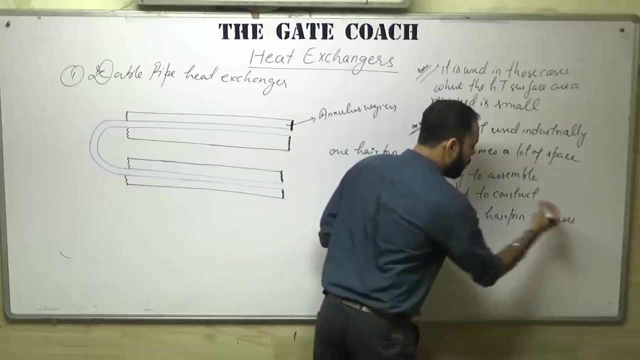 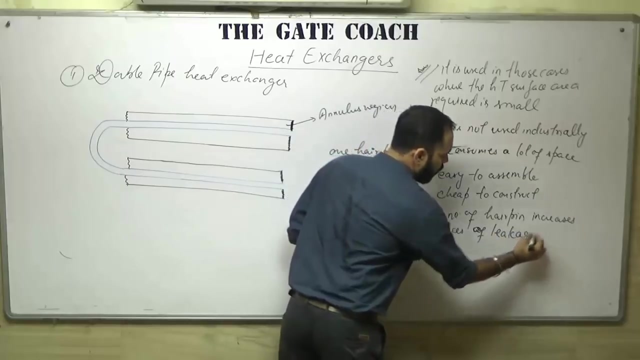 of hair pains. as you increase the number of hair pains, the chances of leakage will increase as number of hair pin increases. why the number of hair pin will increase? because I want to provide more surface area for heat transfer. as the number of hair pin increases, increases, chances of leakage will increase. chances of leakage increases. why there will 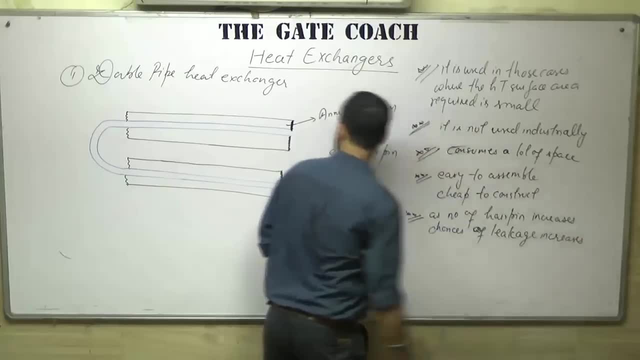 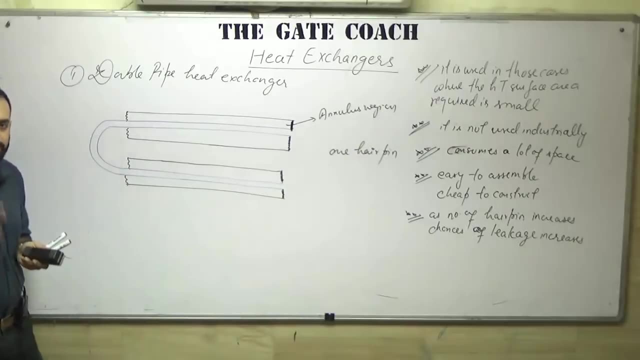 be leakage because in a double pipe heat exchanger there are a lot of bolts and lot of joints and if you see, in one hairpin there will be approximate 10 to 12 bolts or joints. so as the number of hairpin increases, okay the chances of leakage, the loss of heat, heat will be there. 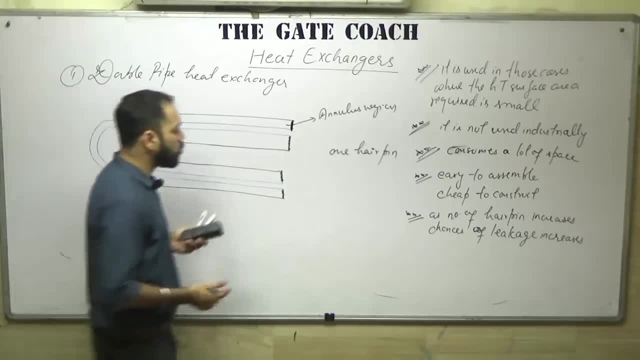 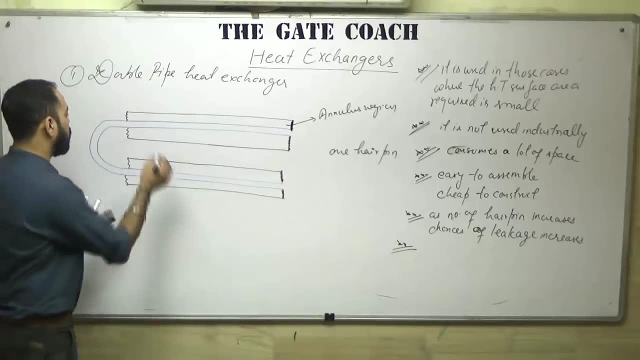 again, which is not economical for us. okay. another issue with this type of heat exchanger is usually what happens in one hairpin: the length of this leg. this is the leg. okay, this is the leg, the length of this leg where the heat transfer is taking place. this is also. 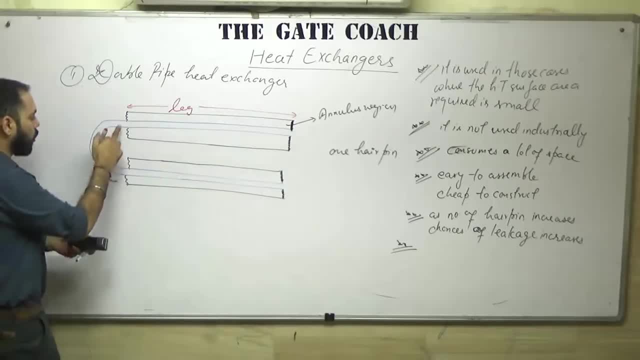 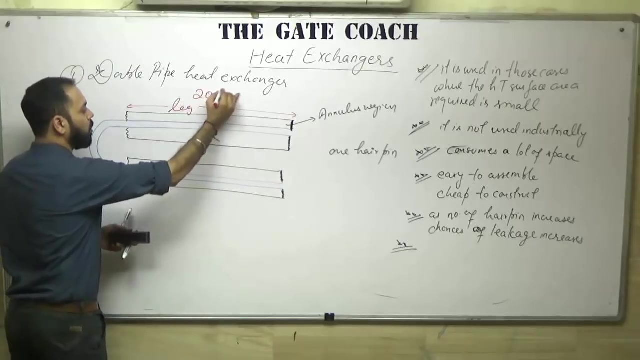 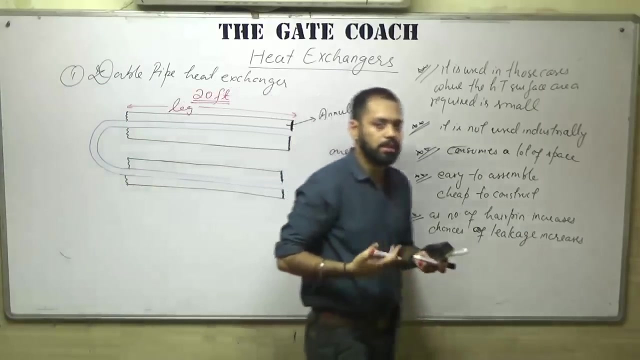 called the effective length. why effective length? because no heat transfer takes place in this particular area. because there is no hot fluid. the two fluids will remain in contact, in this case also in this region. only, right, so the length of this leg cannot be greater than 20 feet. usually the length of one leg is less than 20 feet, 15 feet, 16 feet or maximum. 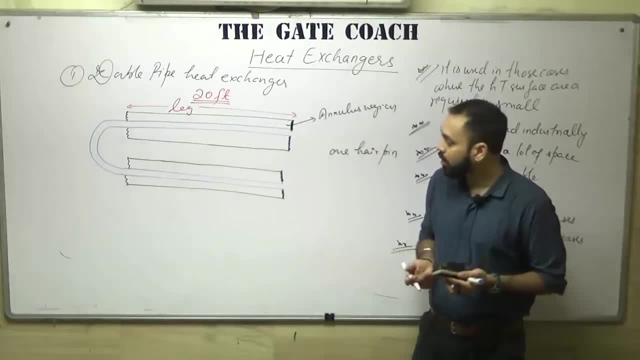 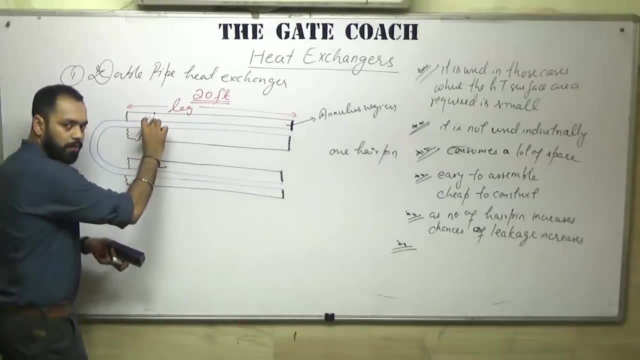 20 feet. it cannot be greater than 20 feet. why? the reason is, if you increase the length of the leg of this hairpin, in that case this inner tube, this inner tube, will start touching the outer tube, Because if you increase the length, the weight of this inner tube will be very high. 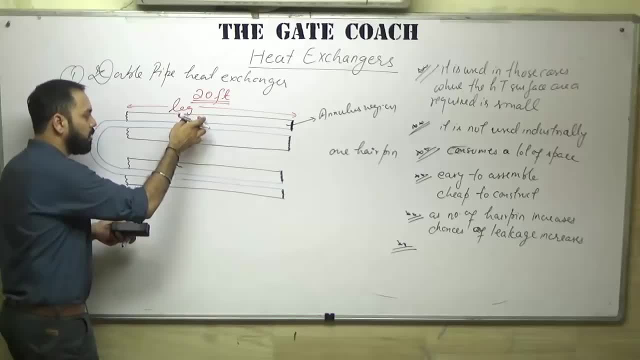 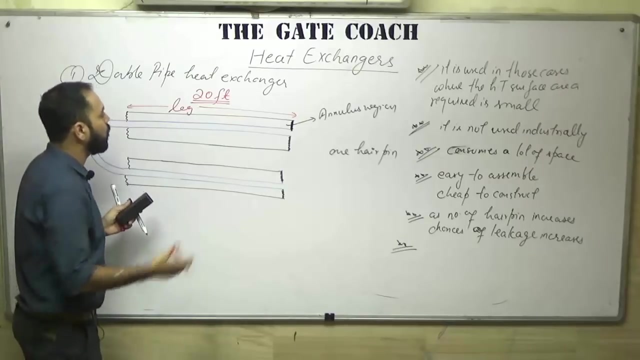 In that case it may touch the annulus tube, this outer tube. that will disturb the flow pattern and that will decrease the efficiency of heat transfer. So that is why we cannot construct- we do not construct usually- double pipe heat exchanger which is having one leg of length greater than 20 feet. 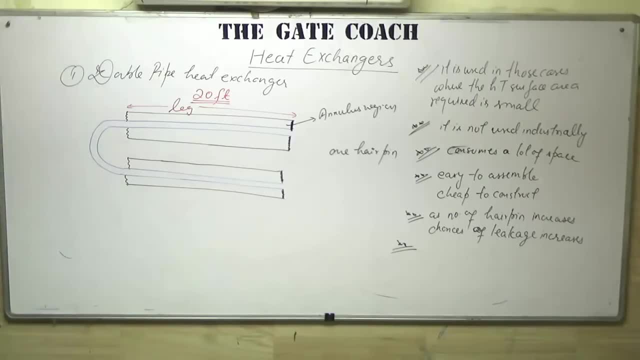 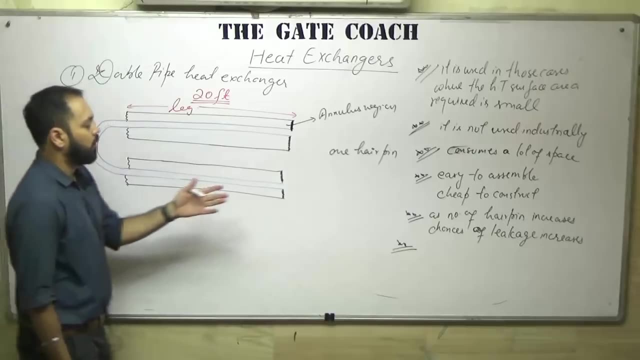 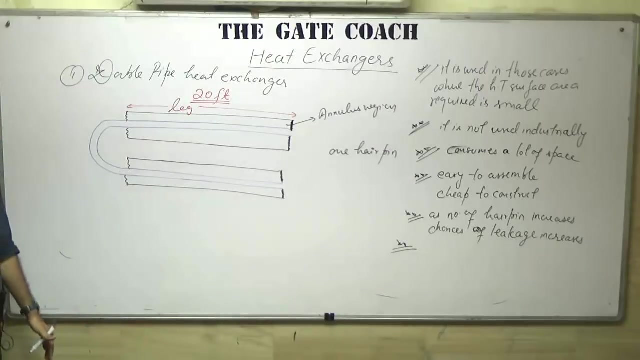 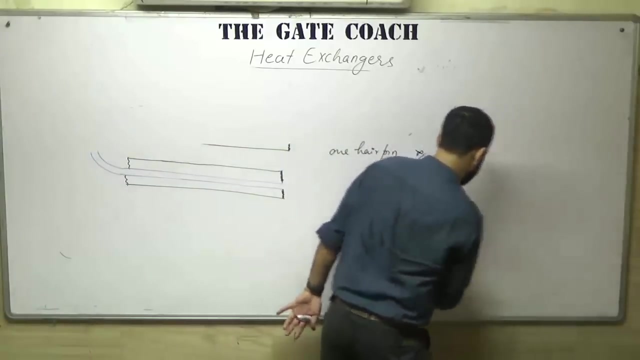 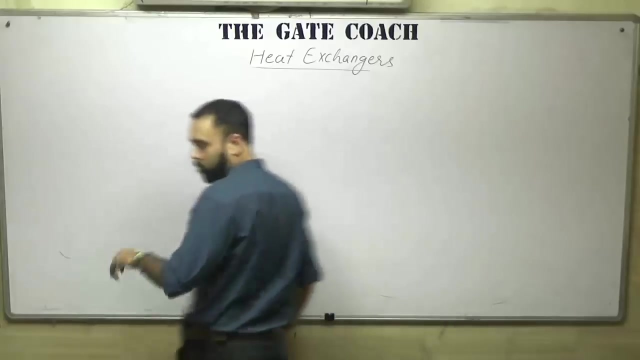 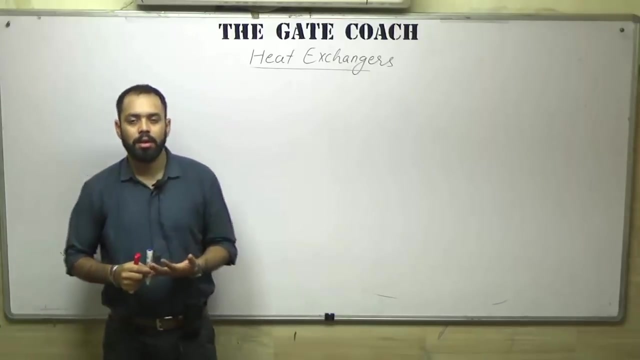 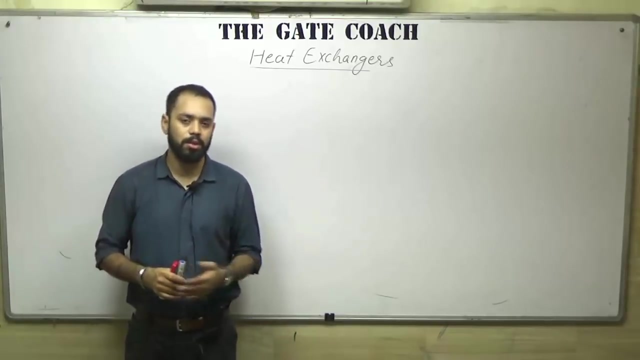 So this was about when double pipe heat exchangers will be used and in which case they cannot be used. what are the advantages and what are the disadvantages of this double pipe heat exchangers? So when you appear for this PSU interviews, please remember one thing that they are not going to ask: what are the different correlations used for finding the value of heat transfer coefficients, like C.8 correlations or other correlations? 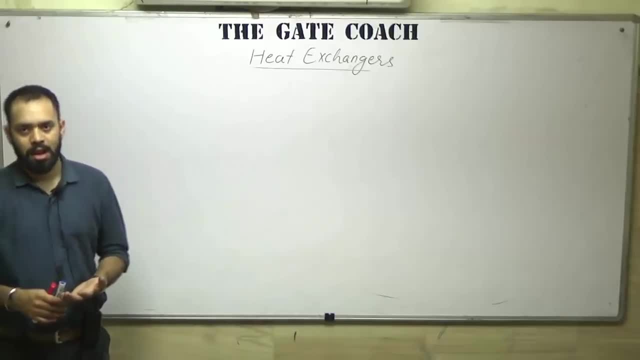 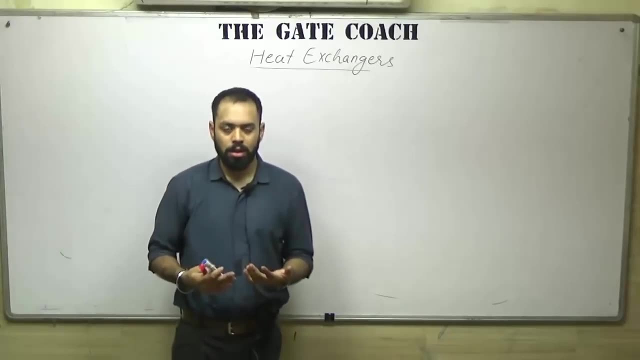 They are not going to ask you to derive to calculate the area, but they will ask these kind of practical questions. Of course you should have the basic knowledge of Kern's method. Kern's method is a method used for designing the heat exchanger. 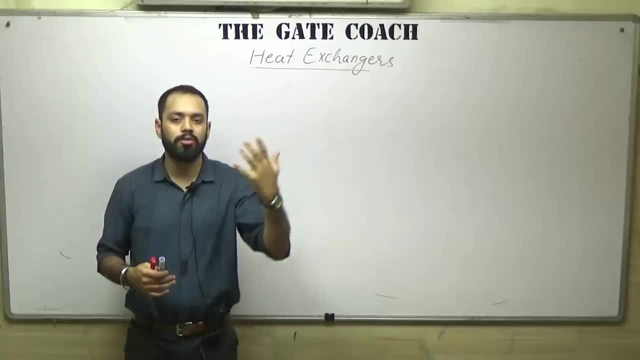 You should have the knowledge of step by step knowledge that what we follow, what is the method which is followed to construct, to calculate the area of a heat exchanger. When we say that we are chemical engineers and we have to design a heat exchanger, what is the meaning of design for us? 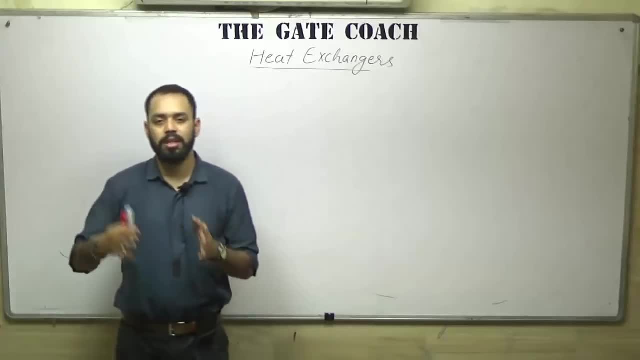 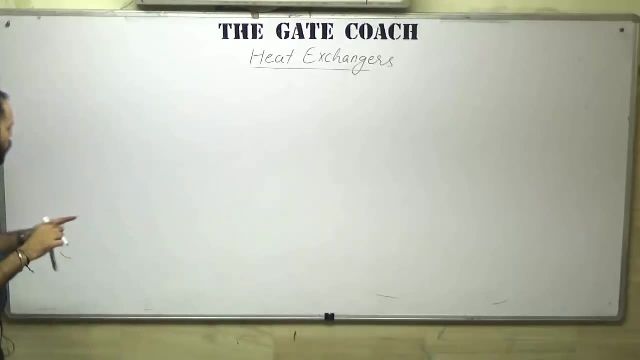 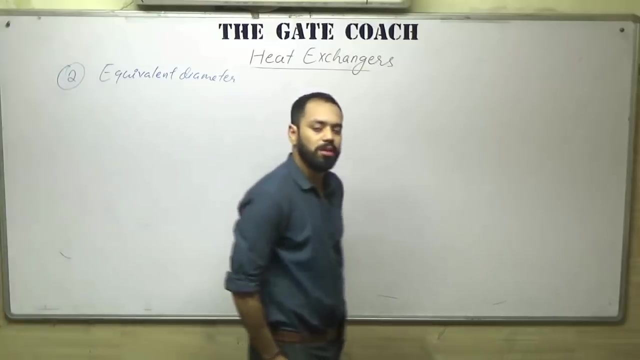 For us, designing a heat exchanger means calculation of the area which is required to complete that heat duty. One more parameter which is asked in the interview In the interviews is the equivalent diameter. Let us suppose that we are using a double pipe heat exchanger and a fluid is flowing inside the tube, other fluid is flowing inside the annulus. 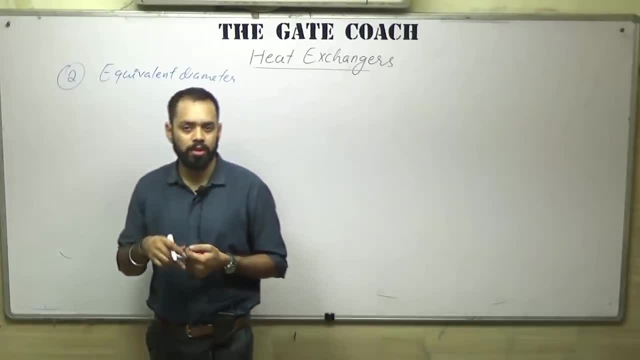 So, for the fluid which is flowing inside the tube, when you have to calculate, let us say, the Reynolds number, the rho Vd by mu, the diameter that you are going to use will be the diameter of the inner tube. Okay, For the fluid which is flowing inside the annulus, we have to use the equivalent diameter. 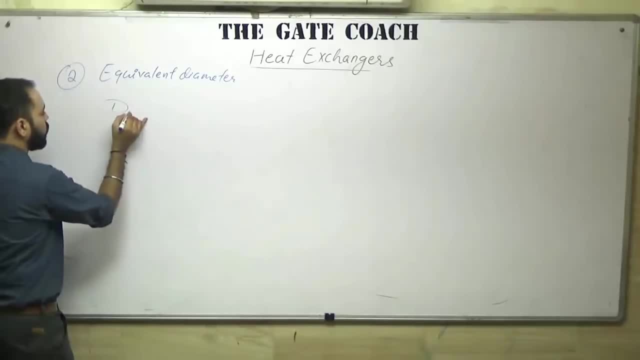 Okay Now what is equivalent diameter? Most of the students are confused. They say that sometimes we use this particular formula, some other times we are using another formula. So let me explain what is equivalent diameter. It is 4 times of hydraulic radius. 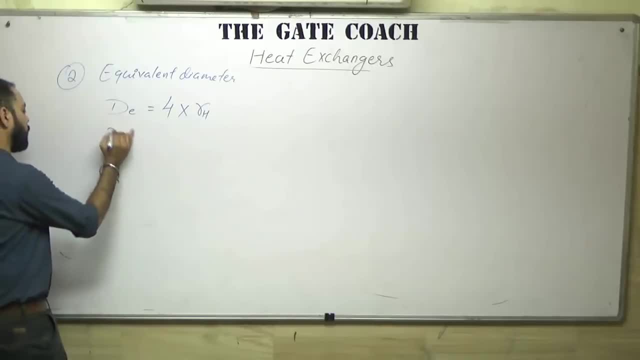 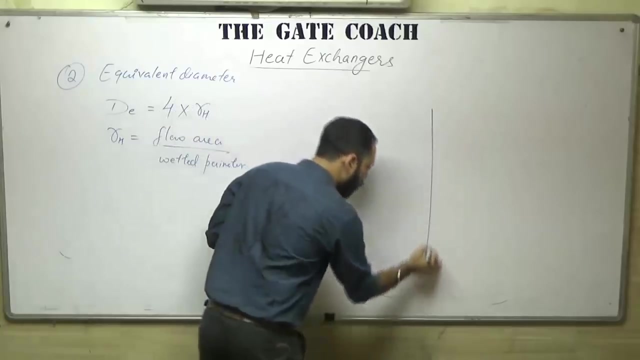 So Rh is hydraulic radius. Now what is hydraulic radius? Hydraulic radius is defined Flow Area divided by wetted perimeter. Okay, So we calculate equivalent diameter in two cases actually: One for the calculation of heat transfer and the other for the calculation of pressure drop. 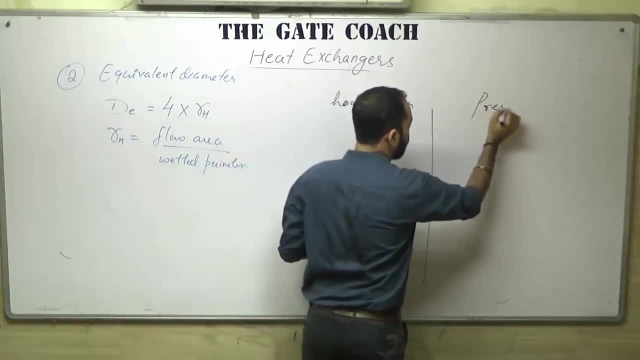 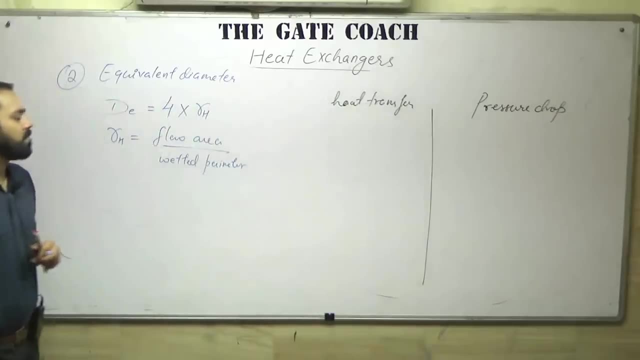 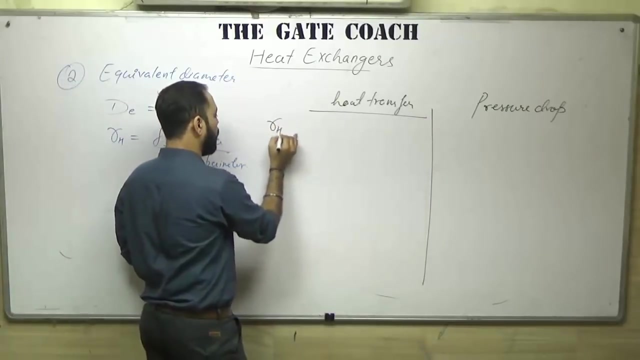 Heat transfer and the other one is for pressure drop. So that is the difference that you have to understand. Okay, If the question is: what is the equivalent diameter for the calculation of heat transfer? so the formula is same, Right, What will be the hydraulic radius here? 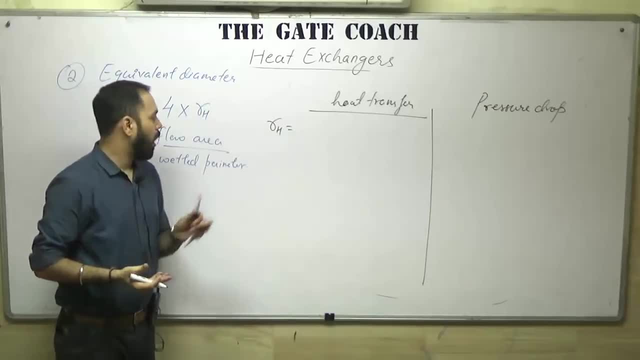 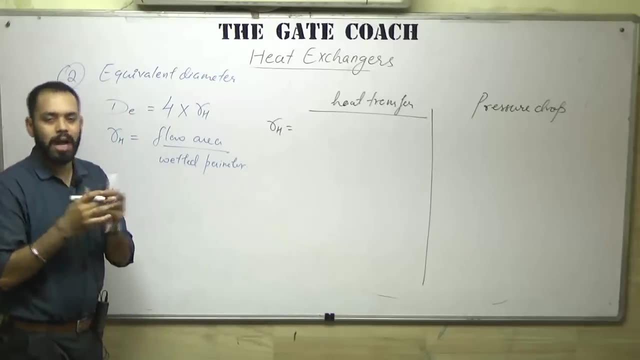 The flow area. So for the annulus fluid I am not doing this calculation for the tube fluid, because for the tube fluid, whatever is the diameter of the inner tube, that will be the diameter used for calculation. But for annulus fluid, what is hydraulic radius? 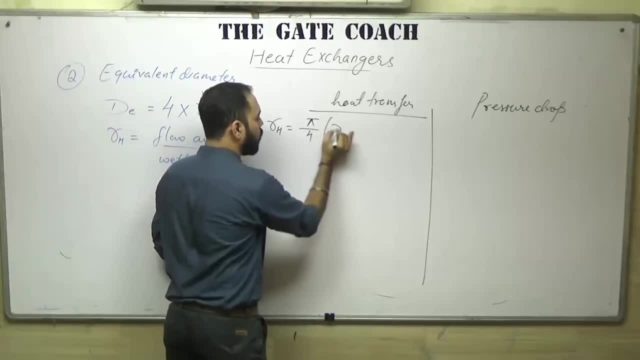 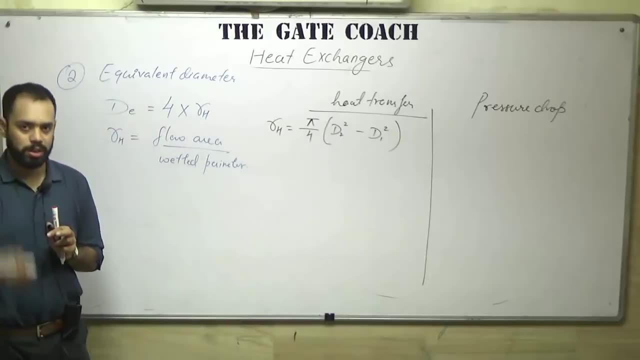 Flow area available. What is flow area available? Pi by 4 d2 square Minus d1 square. What is d2 square? d2 square is the diameter of the outer tube. Okay, Actually this is the inner diameter of the outer tube. 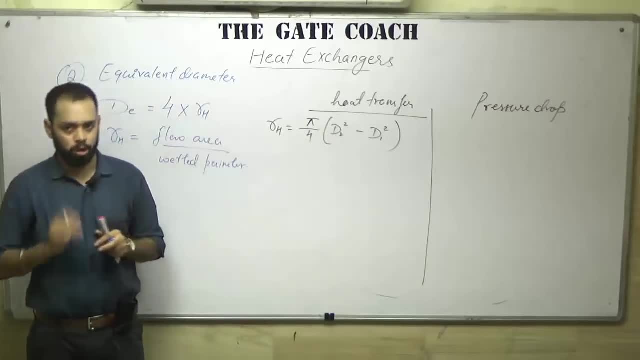 What is d1 square? d1 square is the outer diameter of the inner tube, Assuming that there is some thickness of these tubes. Therefore, I am saying like this: So this is the flow area. What is the wetted perimeter? 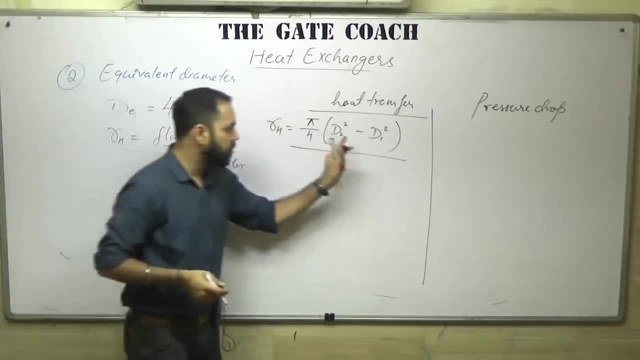 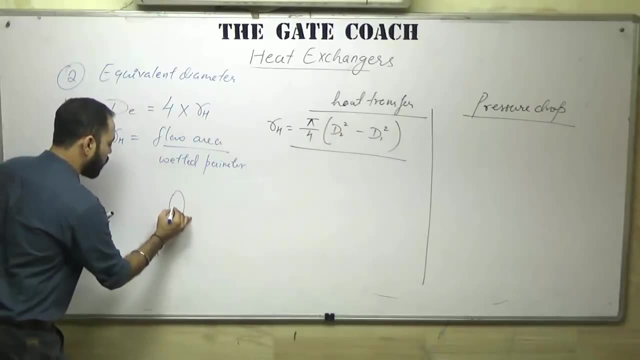 Now there is a difference in the wetted perimeter for heat transfer and for pressure drop. Okay, Because, Because, Because, if this is the annulus for heat transfer, heat transfer will be taking place only on the outer surface of the inner tube. 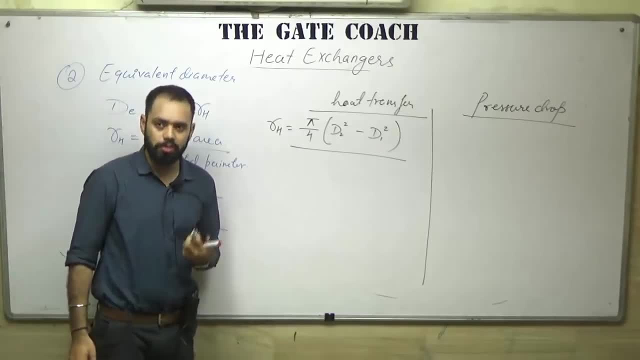 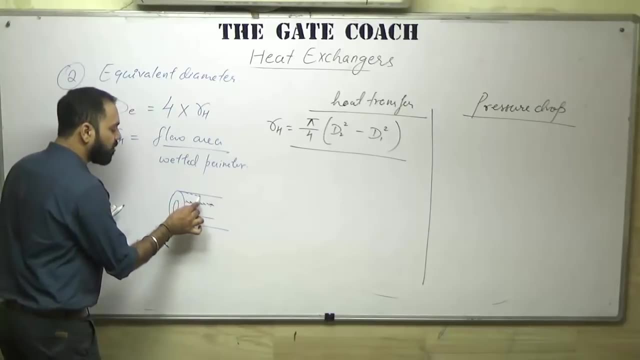 While for pressure drop calculation, which is due to frictional forces, the frictional forces are offered by the outer surface of the inner tube as well as by the inner tube, By the inner surface of the outer tube. So that is the difference, friends. 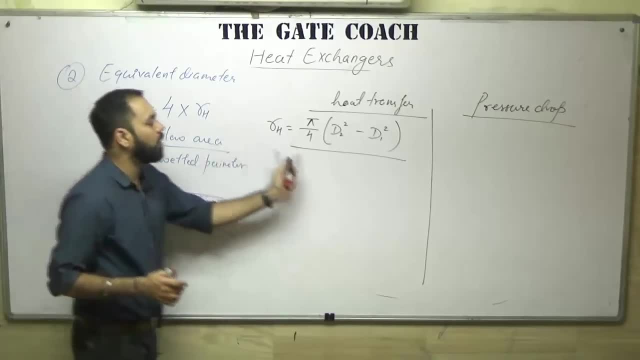 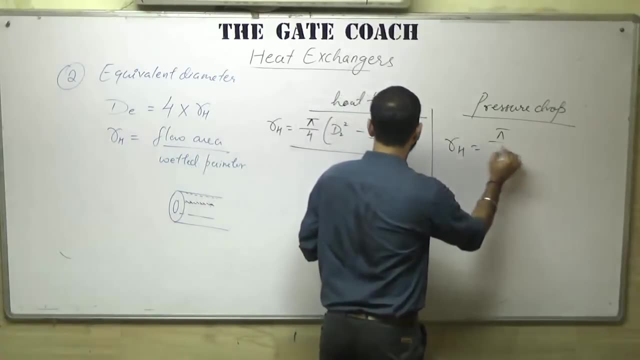 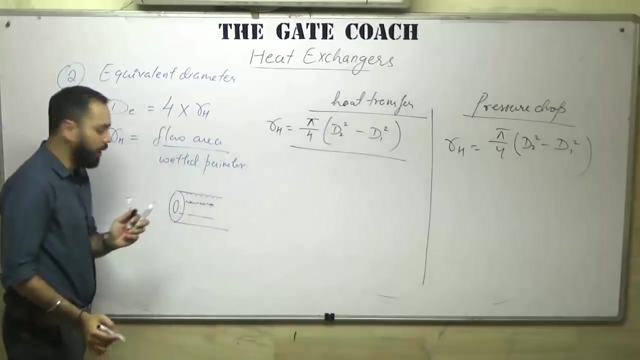 That is the basic difference. That is, the wetted perimeter for heat transfer and for pressure drop. The cross-sectional flow area will be same for pressure drop calculation as well as for heat transfer calculation. So what is the wetted perimeter here? In this case, for heat transfer, the wetted perimeter will be the perimeter of this inner. 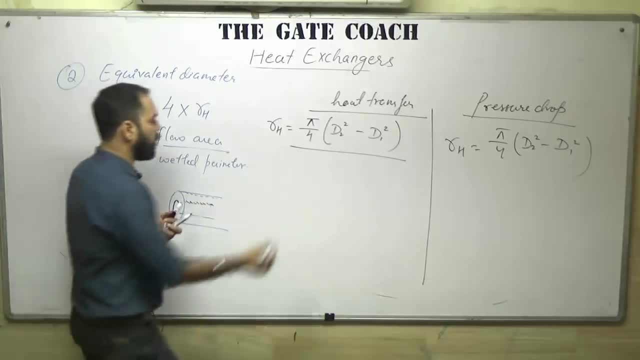 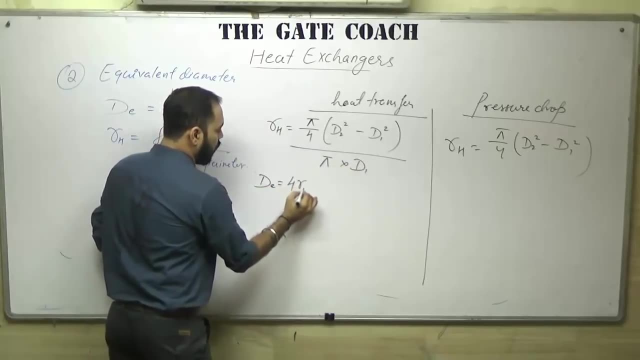 tube. What is the perimeter? 2 pi r, or you can say pi d1, pi into diameter, So that will be pi multiplied by d1.. So therefore, equivalent diameter will be equal to 4 times rh and you will find that. 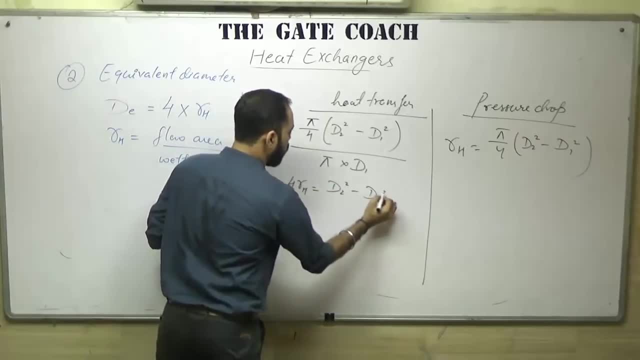 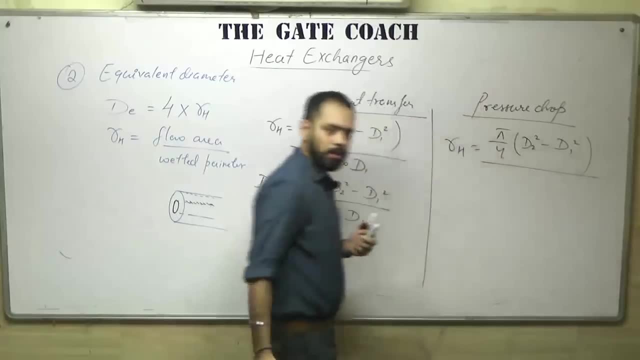 this will be d2 square minus d1 square divided by d1.. Okay, Now for the second case. what is the wetted perimeter? Here, the wetted perimeter will be the perimeter of the inner tube as well as the perimeter of the outer tube. 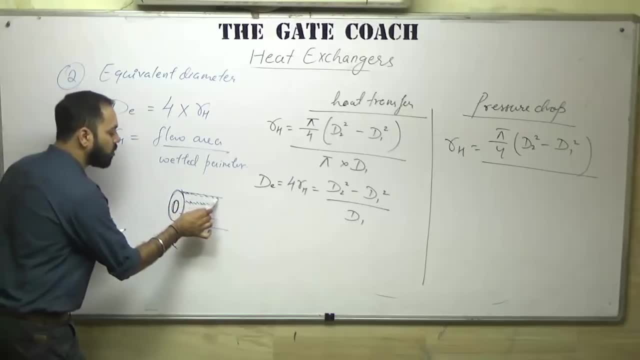 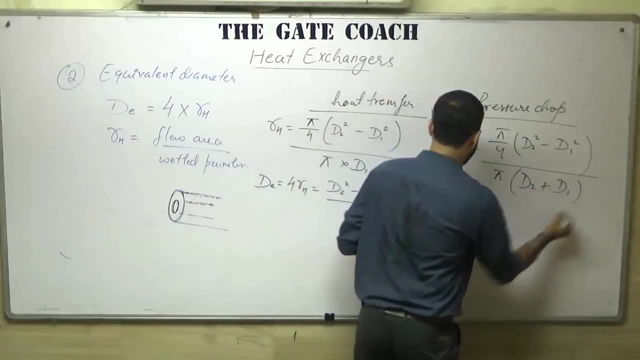 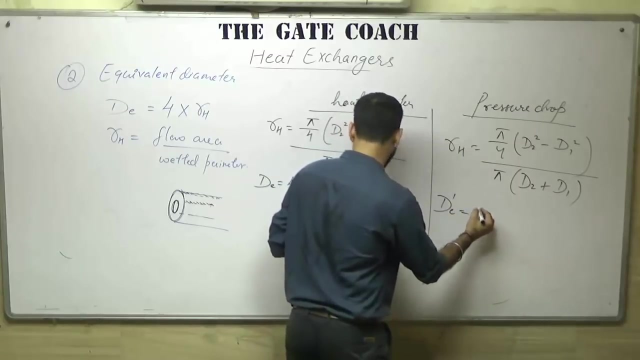 Why? Because frictional forces are offered by the outer tube also. Okay, So therefore this will be pi d2 plus d1 and therefore the equivalent diameter, dE dash in this case, because this is different from the heat transfer equivalent diameter. that. 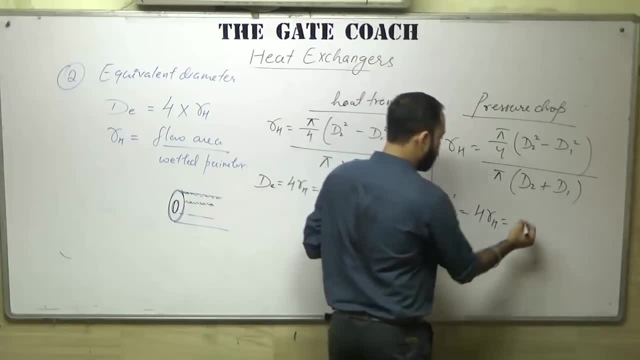 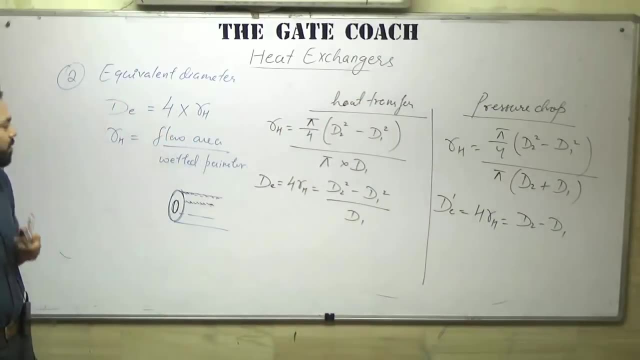 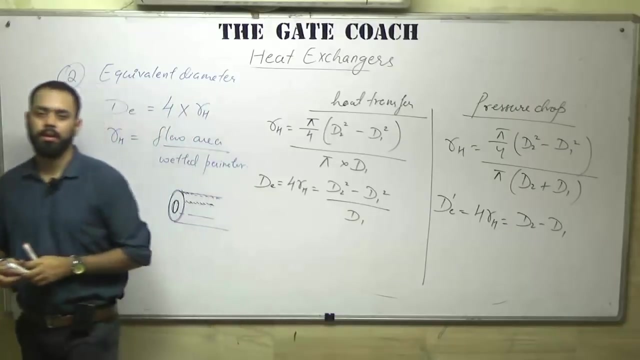 is 4 times rh and that will be equal to. you will see this is d2 minus d1.. So that is the difference between the calculation of equivalent diameter for calculation of heat transfer and for calculation of Okay Pressure draw. Why this equivalent diameter is used? 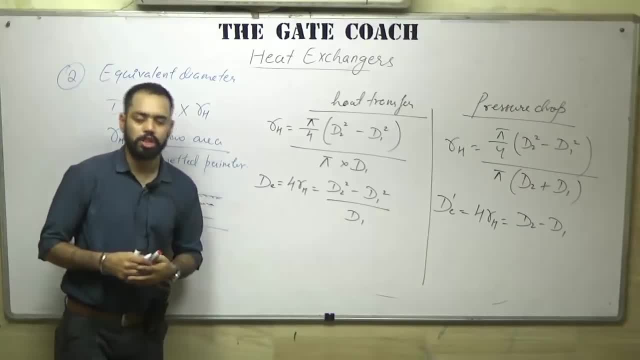 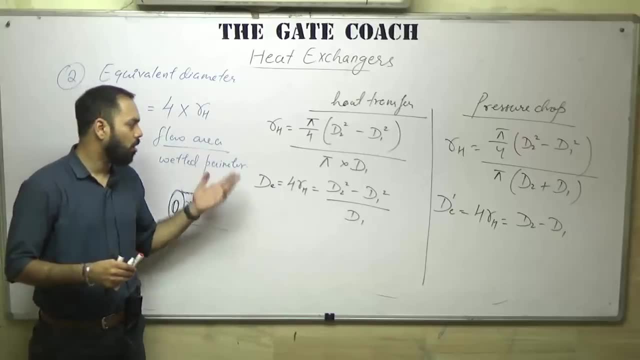 If you see the steps involved in designing of a heat exchanger, that is, in the Kern's method, you will see that we have to check the Reynolds number of the annulus fluid or of the tube fluid. So there, we have to use this equivalent diameter. 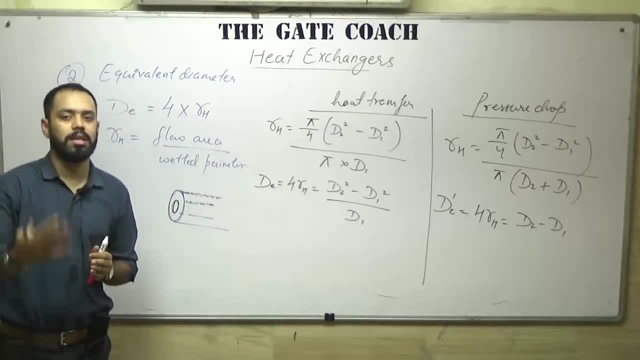 So please go through the steps. We should have the knowledge of only steps, not the detailed calculation, because in PSC interviews they are not academics, they are not professors, they are not going to ask you to derive these relationships. They are industrialist, they have industry experience. they are going to ask you problems. 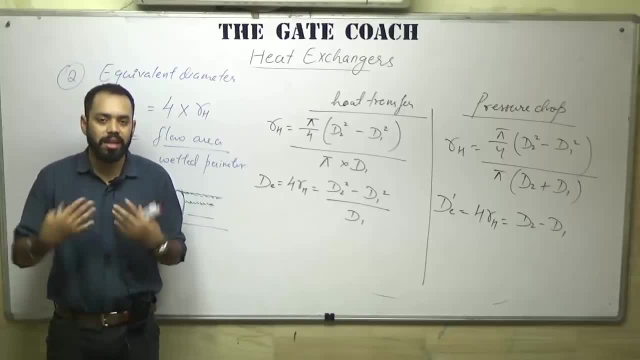 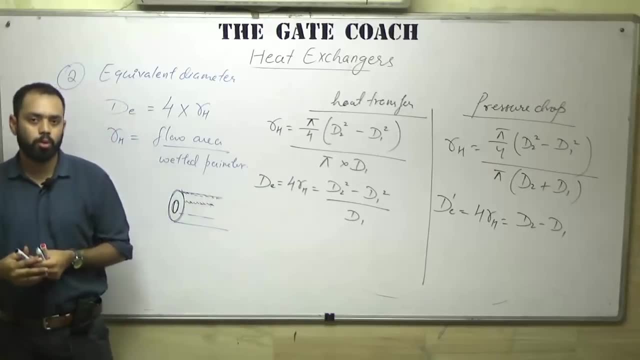 related with the heat exchanger. what are the different problems? what are the how to select the heat exchangers right? For which purpose we are going to use which kind of heat exchanger? So these will be the questions. So do not worry about the correlations, do not remember them. 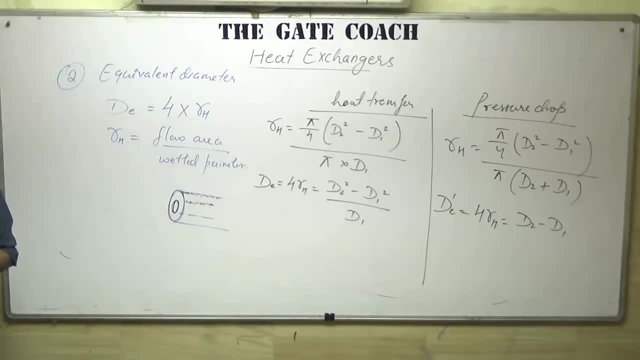 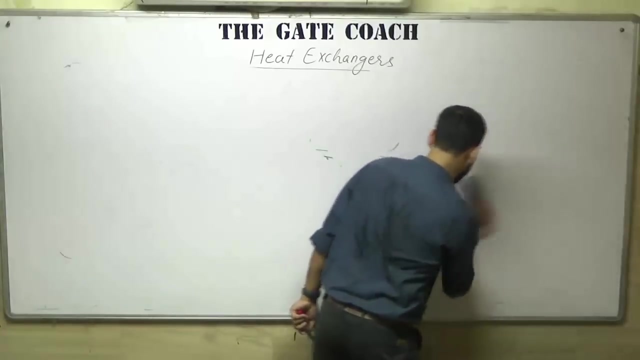 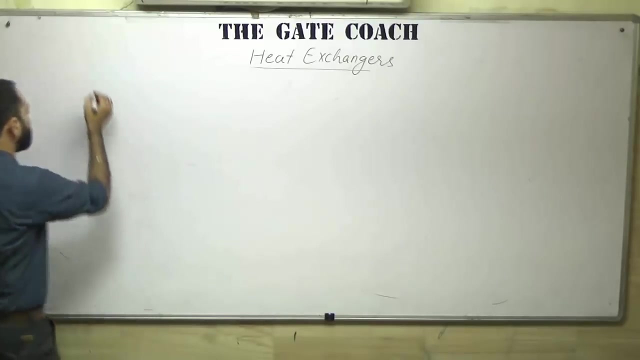 They will not ask the value, the expression of these correlations, right? So, friends, that was about double pipe heat exchangers. Now the next type of heat exchanger is very important and it is usually used in process industries and chemical industries, that is, shell and tube heat exchangers. 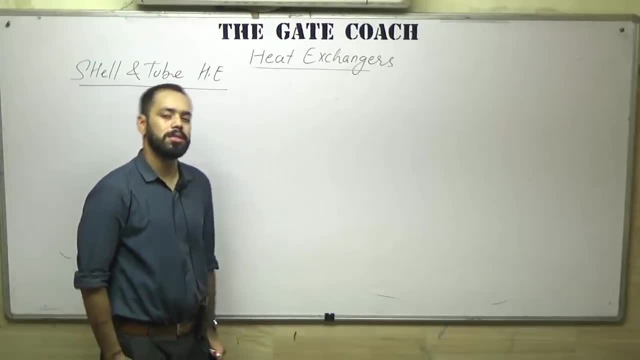 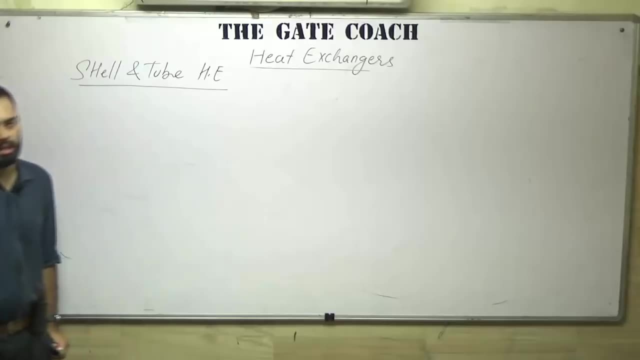 So during your training or during your visits to any plant plant, you must have seen any type of heat exchanger, and most of the time that heat exchanger is a shell and tube heat exchanger. So what is the advantage here of using shell and tube? heat exchanger. The basic advantage is very high heat transfer surface area in a comparatively smaller space. So comparatively means I am comparing the double pipe heat exchanger and shell and tube heat exchanger For the same heat transfer area: the shell and tube heat. 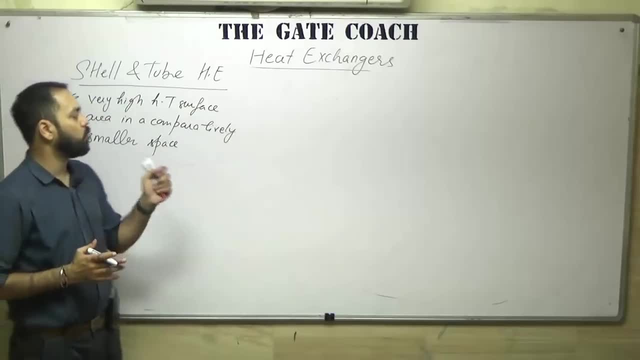 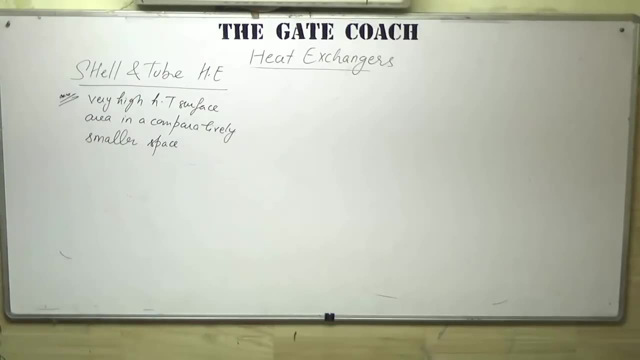 exchanger is going to consume very less space as compared to the double pipe heat exchangers. So we are going to discuss the different components of a shell and tube heat exchanger here. So, first of all, First of all, we are going to discuss the tubes that are used in the case of shell and tube. 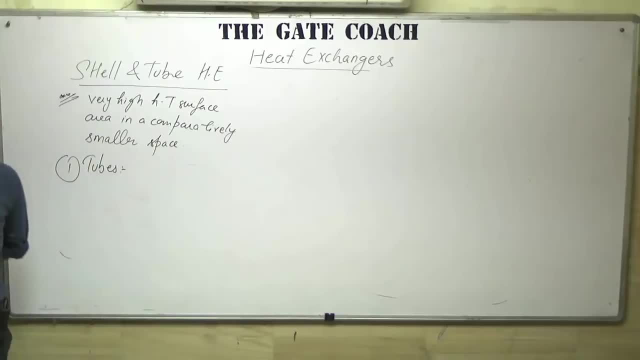 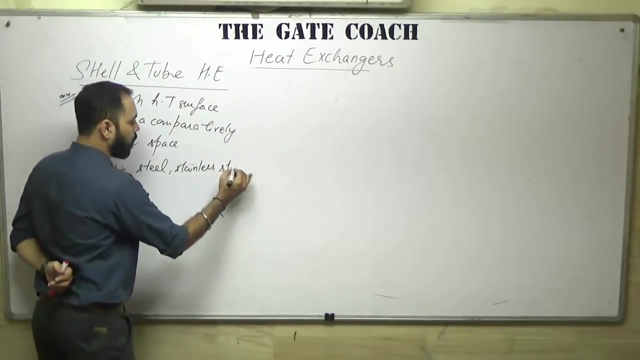 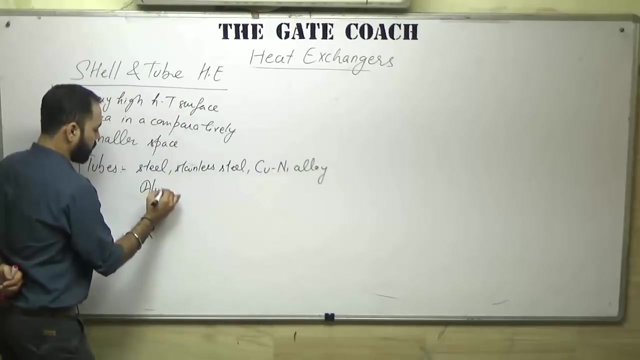 heat exchangers. So the tubes which are used here are usually made up of steel or stainless steel. These kind of questions are asked, that what is the material of construction used for this tube? stainless steel, or you can say copper, nickel alloy, or may be aluminum, copper brass. 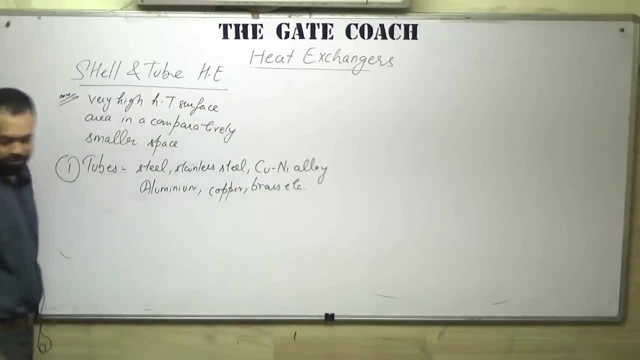 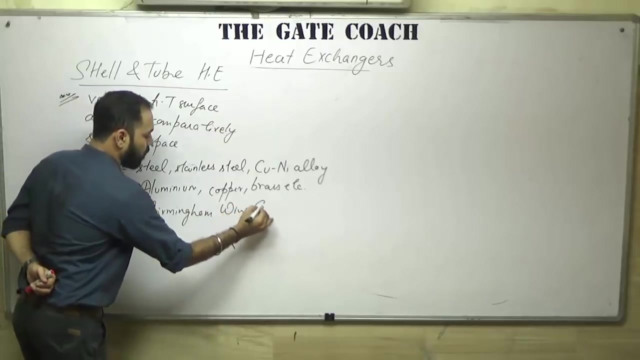 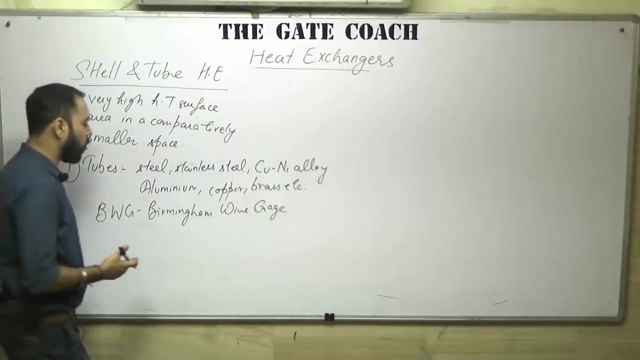 etc. Then there is a term which is called BWG, which is known as Birmingham wire gauge. Okay, So if the interviewer asks you that what is BWG, you should know why it is used, This BWG or Birmingham wire gauge, or sometime it is simply called gauge of the tube. 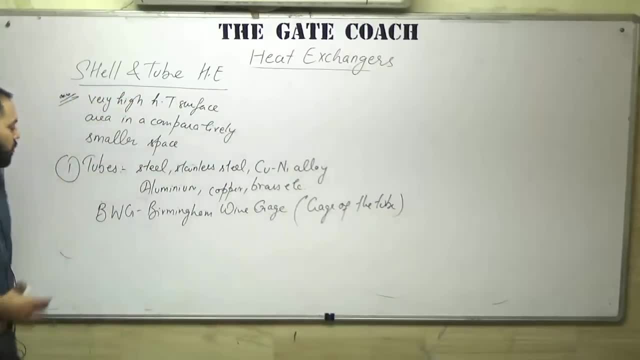 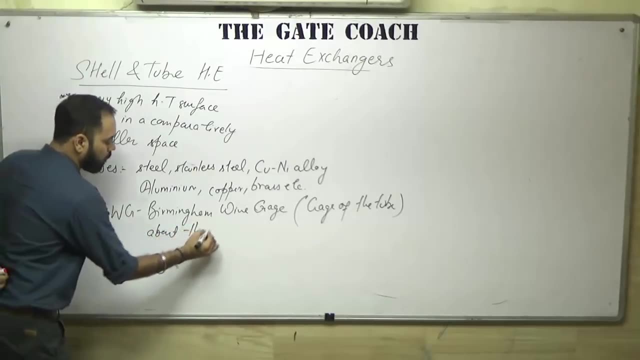 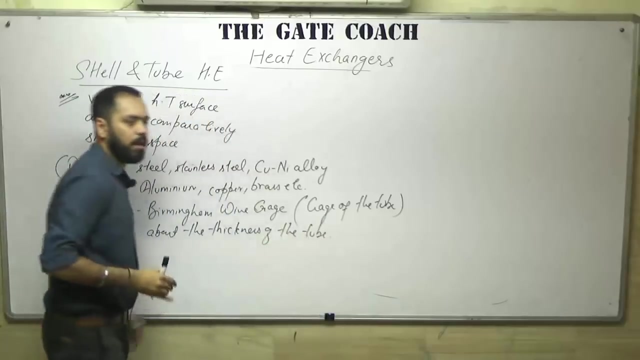 So what information this gauge of the tube gives us? This gauge, or BWG, of any tube gives us information about the thickness of the tube. Thickness of the tube. Thickness of the tube. Let us suppose that the outer diameter, the external diameter of the tube is fixed. 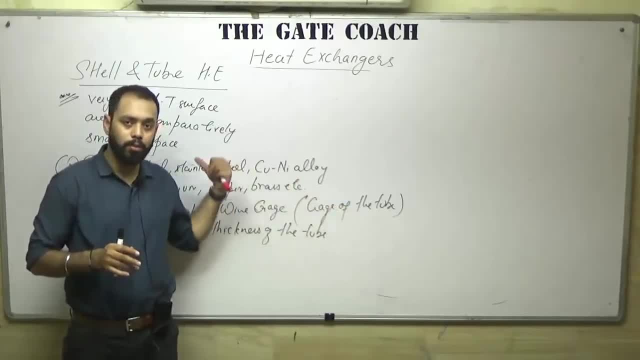 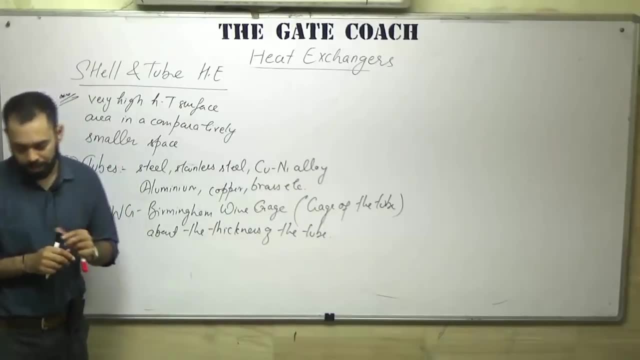 In that case, if the gauge of the tube or if the BWG number of the tube increases, the thickness of the tube will increase. right, Fixing the outer diameter. okay, So generally the outer diameter of the tube is fixed, Okay. 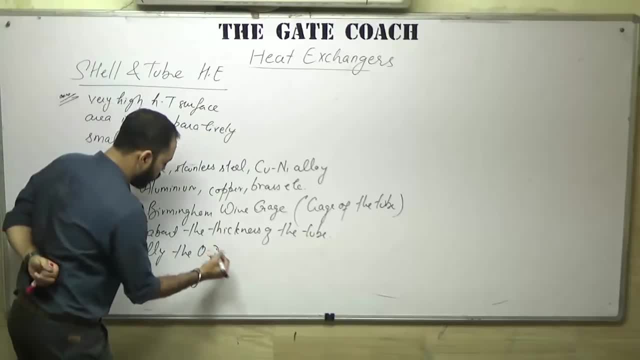 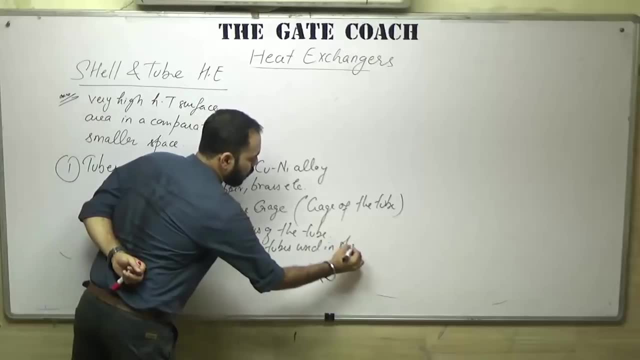 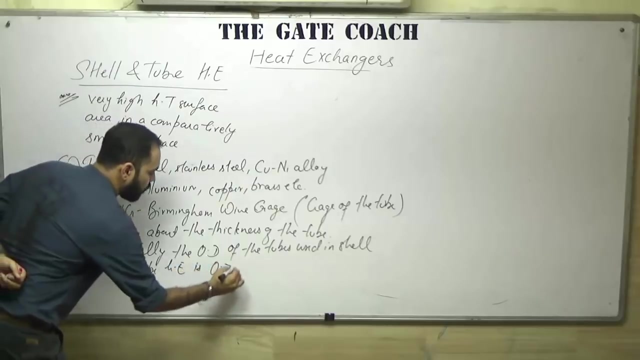 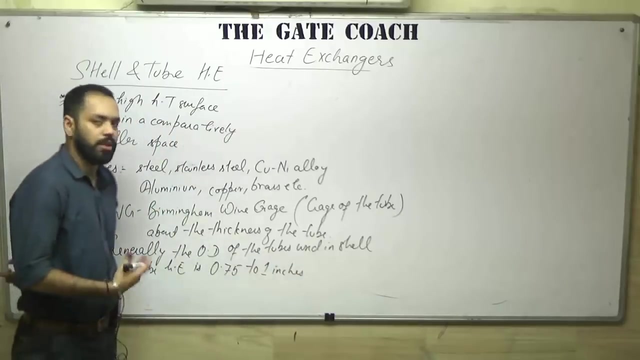 And of the tubes which are used in heat exchanger: shell and tube heat exchanger. of the tubes used in shell and tube heat exchanger is 0.75 to 1 inches. Why I am writing these data? See, I am not saying to memorize everything, but sometimes the interviewer will ask you. 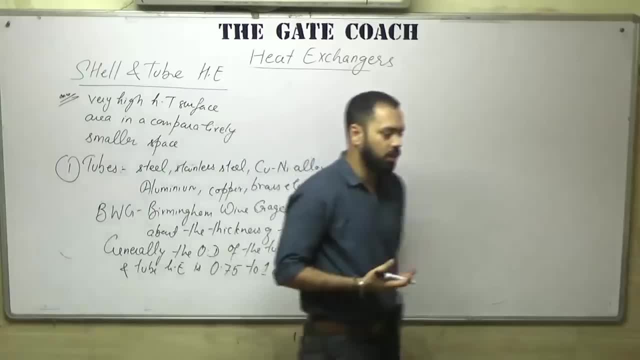 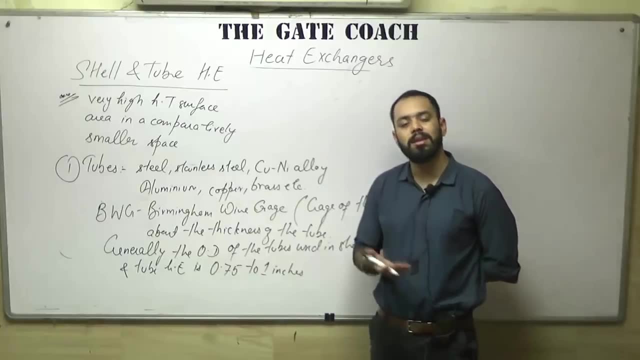 have you seen any heat exchanger? Yes, So you are going to say, yes, we have seen the heat exchanger during our training or during our, let us say, lab experiments. also, we have seen some heat exchanger. Then he may ask that what was the material of construction of the heat exchanger? 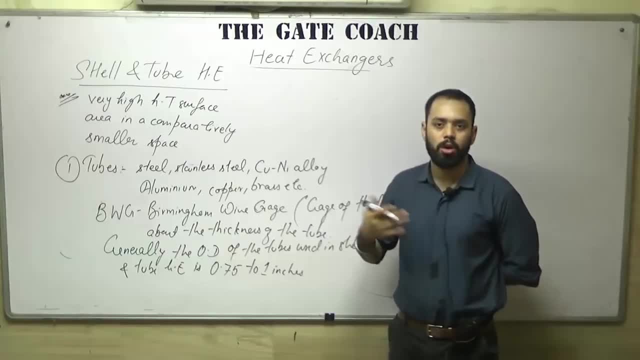 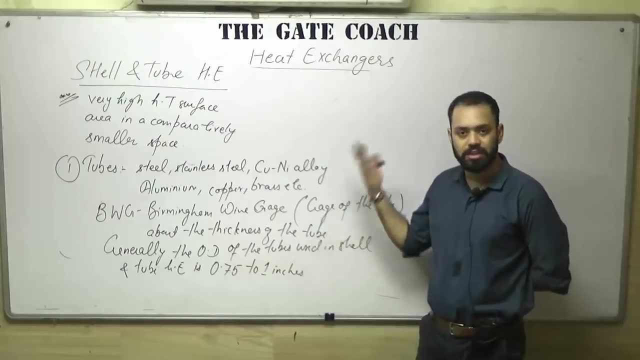 So, being a chemical engineer, you should not say something which is very awkward, which is not possible. If he asks you that what is the diameter of the tube which is used in the heat exchanger, you should not say, sir, 5 inches or 10 inches, okay, 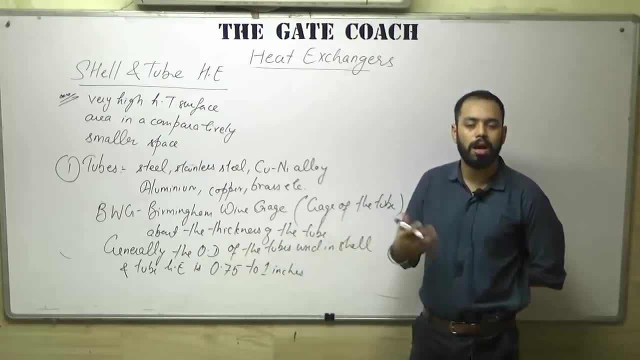 You can say 1.5 inches or 1.15 inches. that is acceptable. your answer should look like you have the basic knowledge of a heat exchanger, So that is why I am writing this data. no need to memorize this, but you should have. 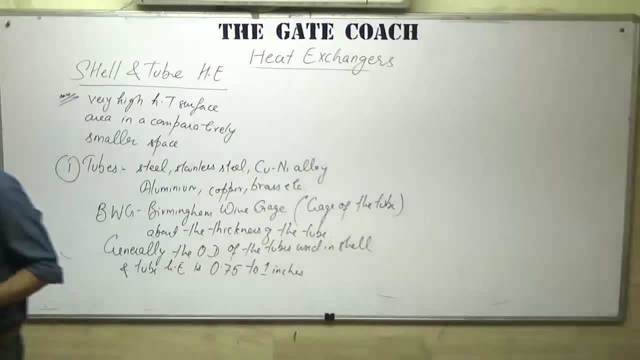 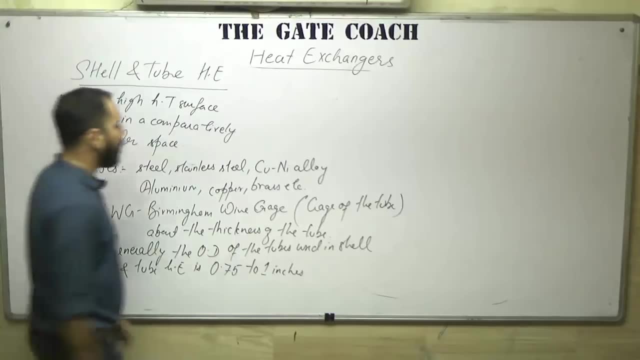 an idea. okay, So this is about the tube and the BWG, or the gauge of the tube which is used for a shell and tube heat exchanger. Then there is a term which is associated with shell and tube heat exchanger that is called 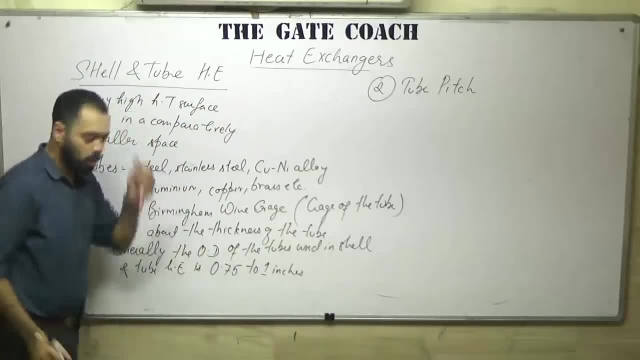 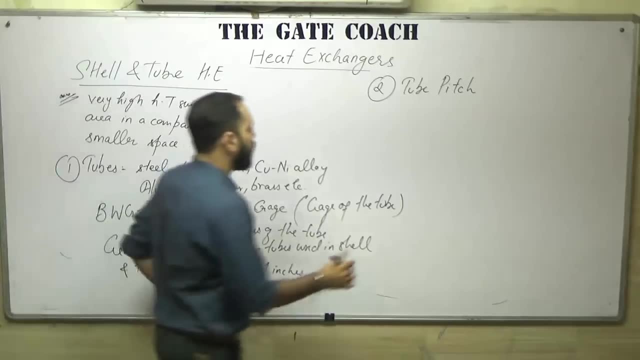 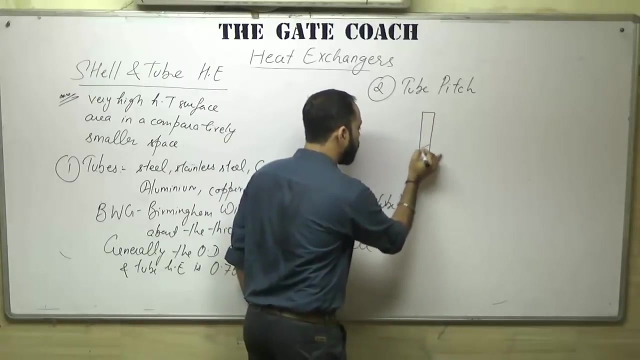 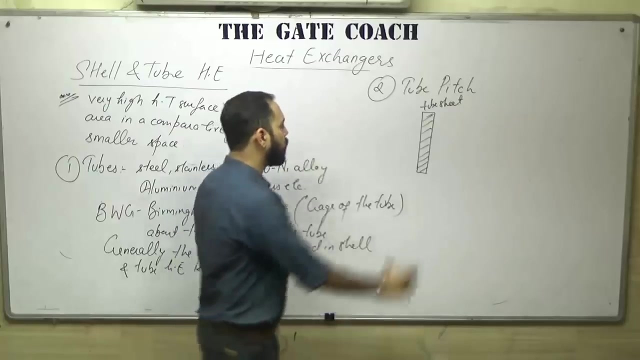 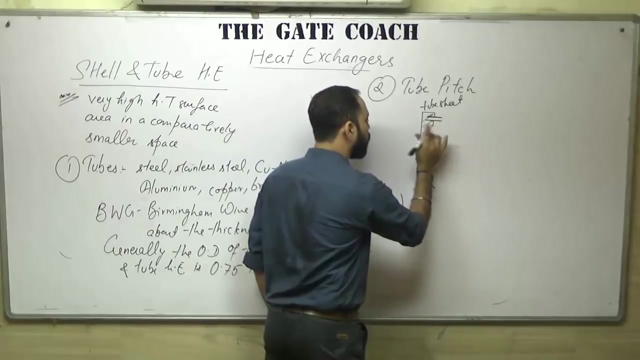 tube pitch. okay, What is the meaning of tube pitch? Okay, In heat exchanger there is a plate which is called tube sheet. right, This plate is called tube sheet. In this plate there are small holes which are made in which the tubes are fixed. okay, 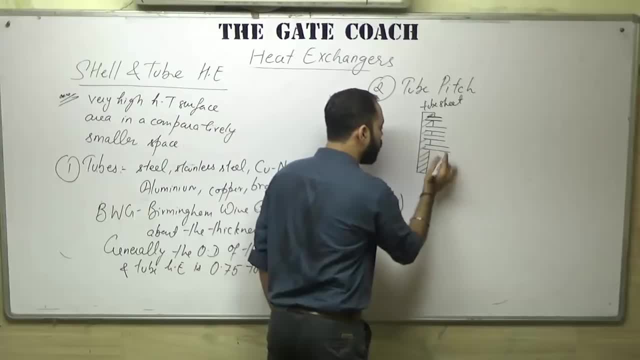 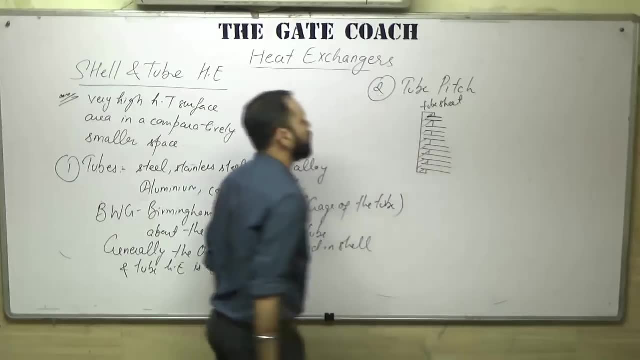 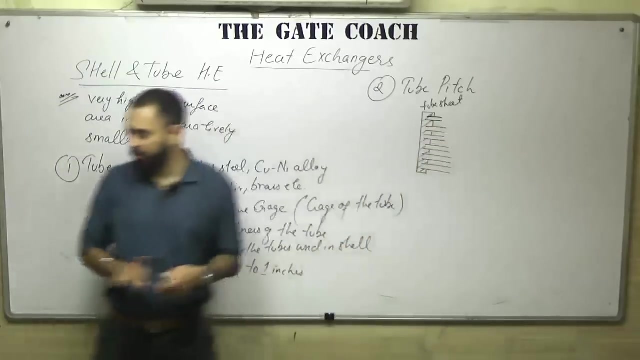 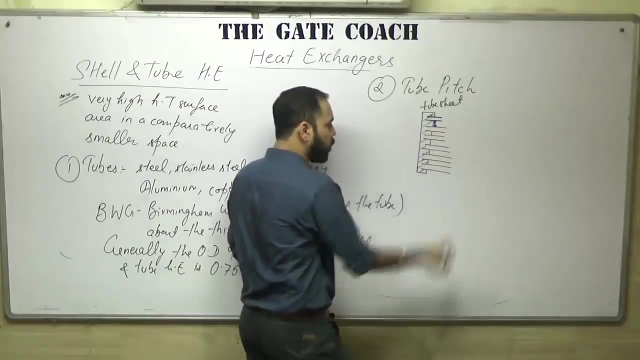 The tubes are fixed in this, so they help us to support the tubes, okay, Otherwise the tubes will not remain at their fixed place. So, like this, the tubes are fixed in this tube sheet, okay. The closest space, the smallest space between two adjacent tubes in a tube sheet is called 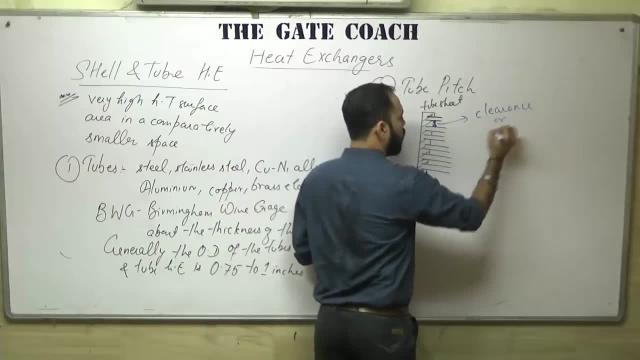 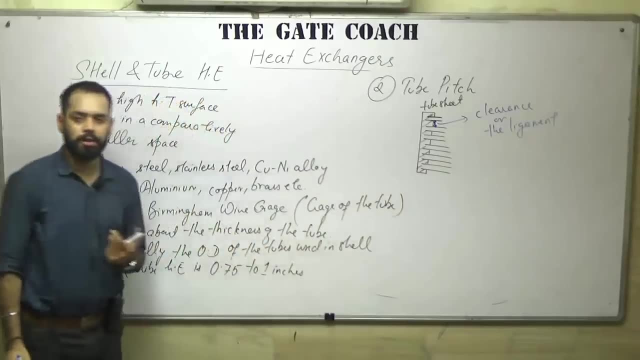 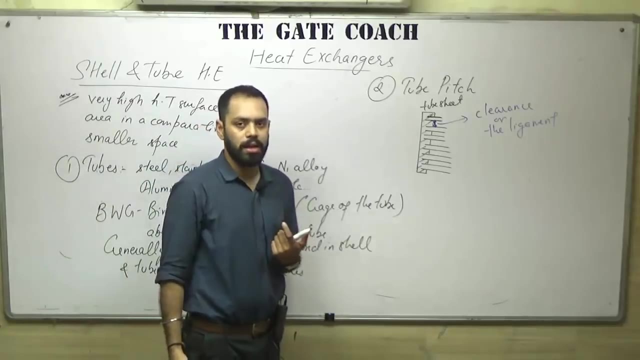 clearance Okay, Clearance, Okay. And then we have the diopter and the ligament. I hope all of you are aware with the definition of ligament efficiency. So there is a definition which is called as ligament efficiency. Okay, You can go through standard text and you can find what is ligament efficiency. 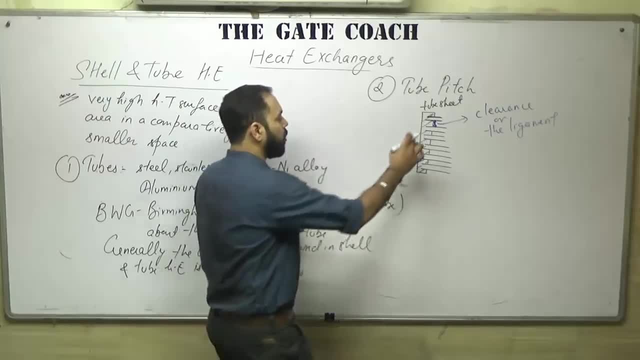 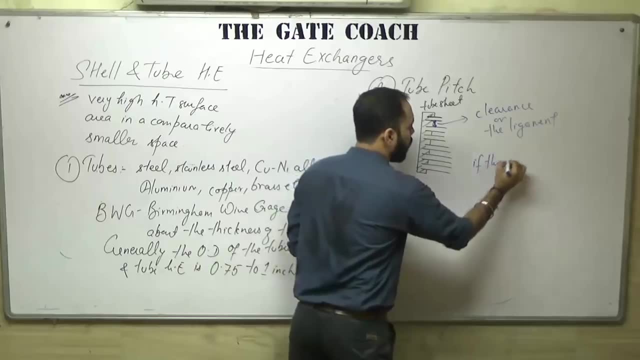 So that definition is associated with this. What happens is that if you drill these holes very close, then it will. if the holes are…if the holes are…if the holes are…there are holes for this because of the two different holes. These holes are for the sum of the holes. 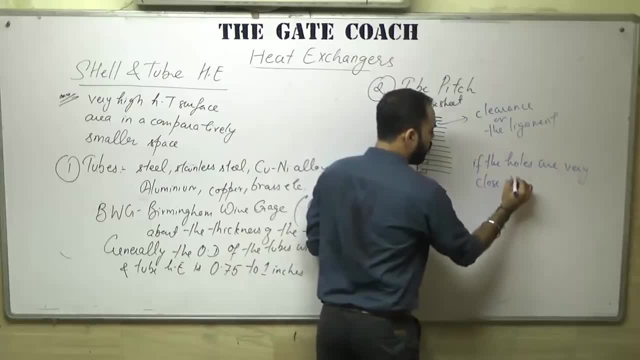 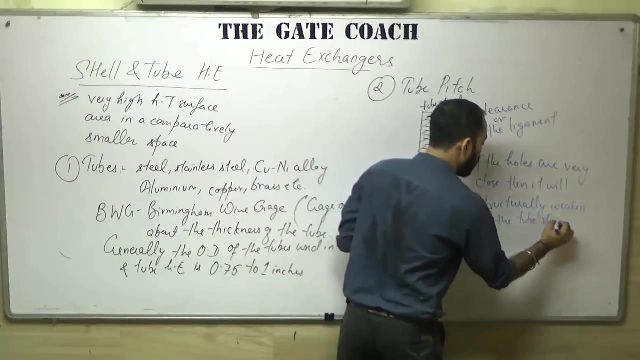 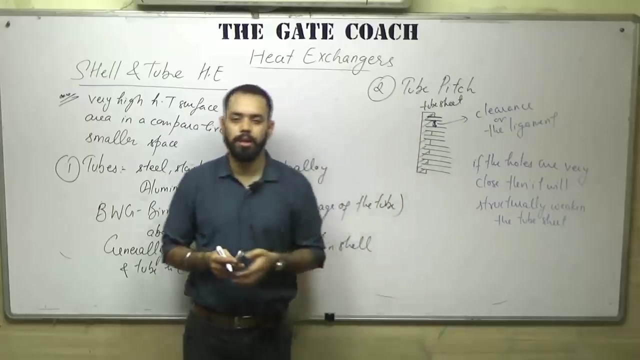 very close, then it will structurally weaken the tube sheet, because the tube sheet is a metal right? if you are drilling these holes very close, in that case the structural strength of the tube sheet will become very low. okay, so this is the parameter which should be considered. 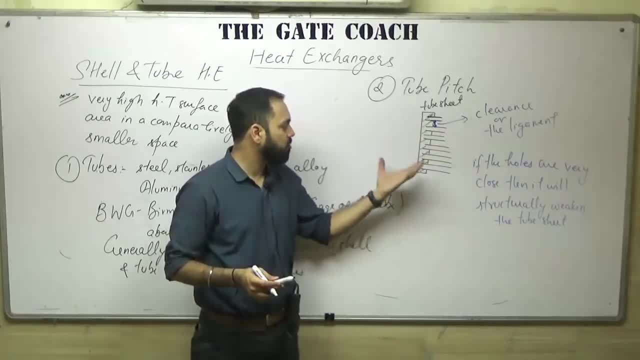 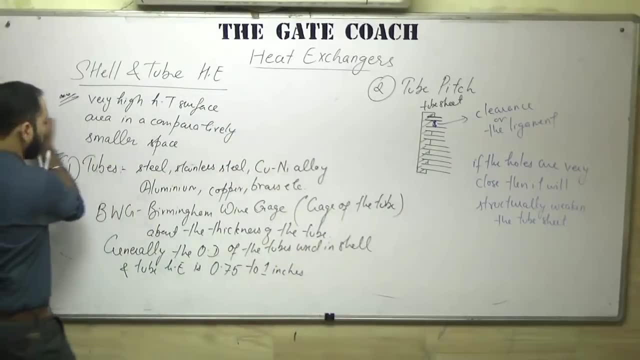 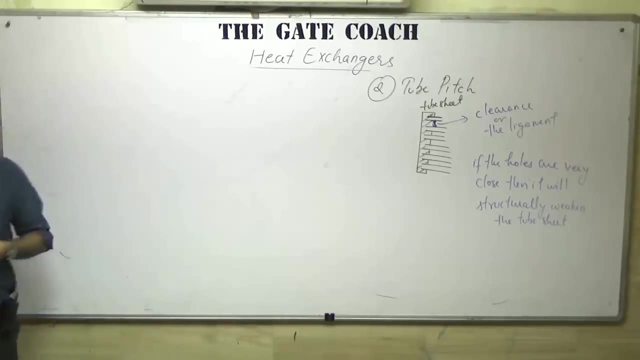 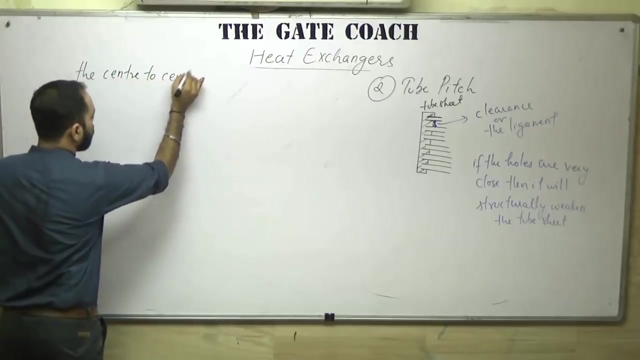 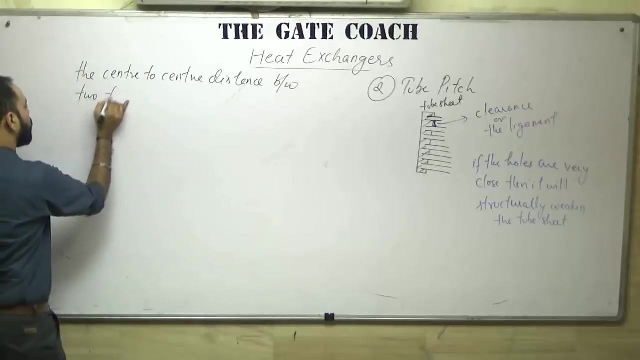 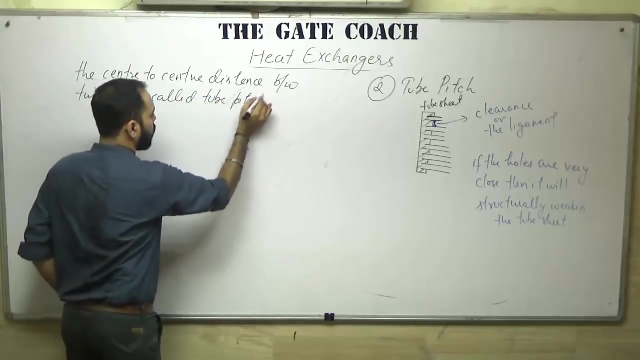 the space is called clearance or the ligament, and there is a definition associated with this that is called ligament efficiency. so please go through the definition of ligament efficiency. okay, now we were discussing the tube pitch. what is tube pitch? the center to center, distance between two tubes is called tube pitch, the center to center. 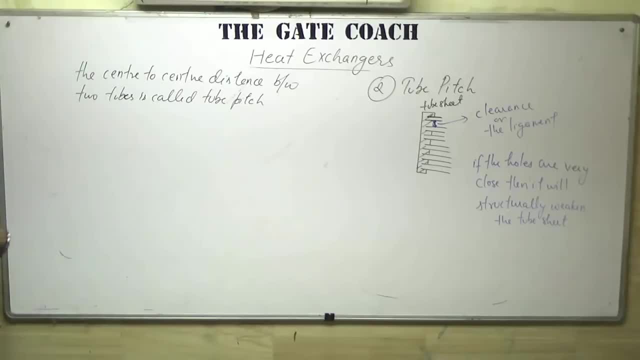 distance between two tubes is called tube pitch, and there are different types of pitch which can be used in a heat exchanger. so let us consider that this is the cross section of a tube. okay, so the tubes can be arranged like this. okay, so this distance, the center to center distance, here is known as the pitch. so if 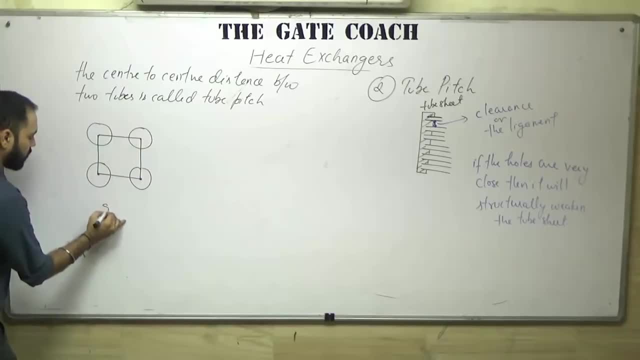 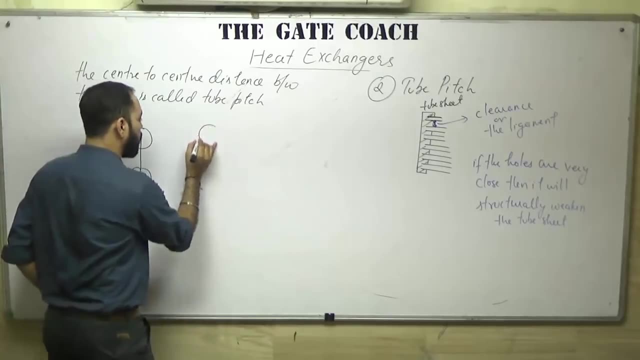 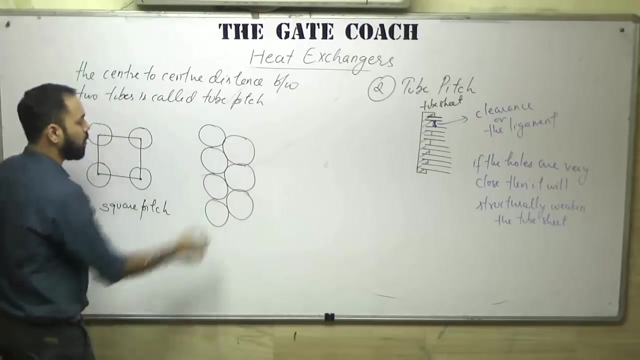 the tubes are arranged like this. this kind of pitch is known as square pitch. okay, also, the tubes can be arranged like this: okay, okay, okay, okay, okay, okay, okay. so let this. the tubes can be arranged. in that case. the center to center distance will be known as the pitch, and this kind of pitch is known as the triangular pitch. these are: 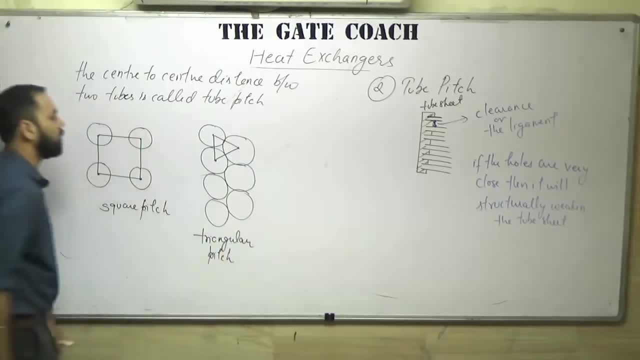 the two most common tube pitches in a heat exchanger. there is a rotated square pitch also and there are some other pitches, but this two are the most common pitch. now for this particular type, for the square pitch and a heat exchanger, there are two types of. 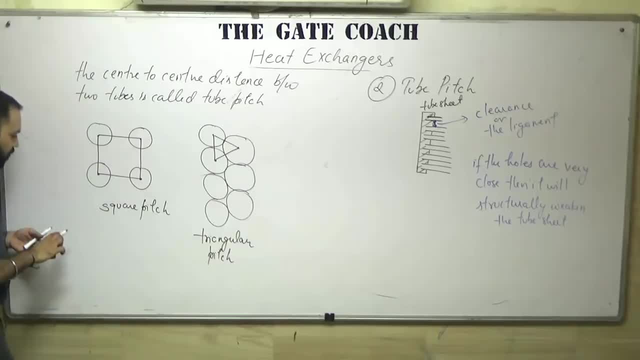 pitch the two most common委igar peacefully in a हά sabes dye, air自由 in a heat. there are some benefits. What are the benefits? That if the tubes are arranged in a square pitch, then external cleaning becomes easier. External cleaning of the tubes is easier. 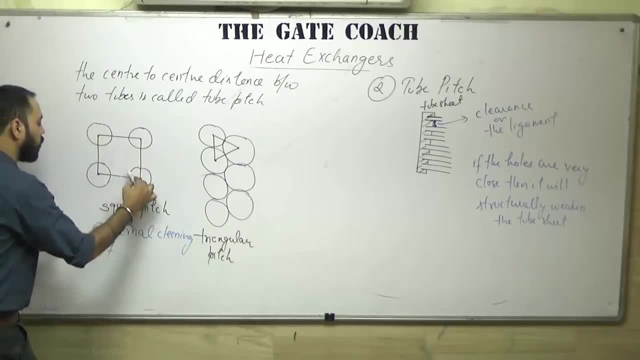 What is the external cleaning? If these are the tubes like this, this external surface of the tubes can be cleaned easily because there is a lot of space between these two tubes, So external cleaning of the tubes becomes easier. This is not the case with 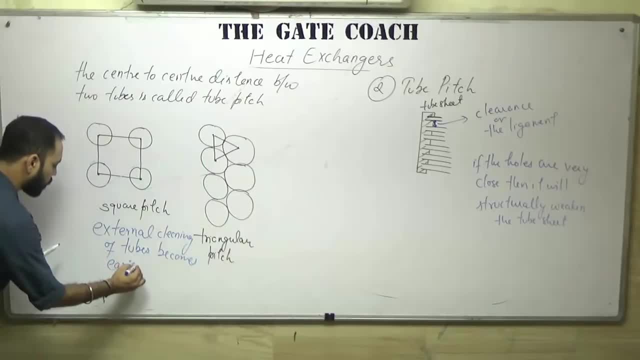 the triangular pitch. Also, in case of this square pitch of the tubes, the pressure drop will be small because you can see there is a lot of space between the tubes So that the external fluid can flow easily between the tubes. So the pressure drop offered. well, It will be small, while it will be higher in the case of triangular pitch tubes. So usually the value of pitch: in case of square pitch it is different. in case of triangular pitch it is different, But usually pitch varies from 1 inches to 1.25 inches. 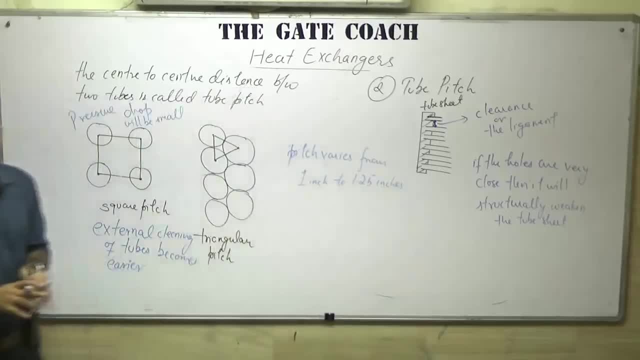 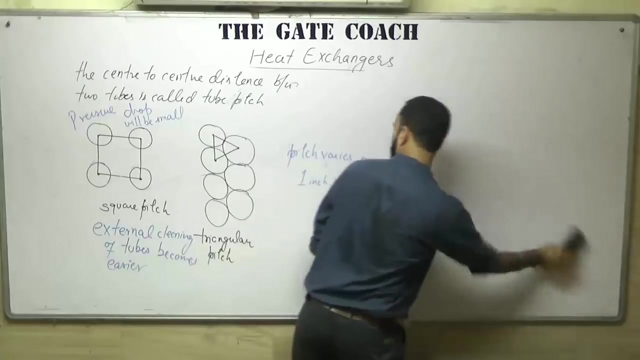 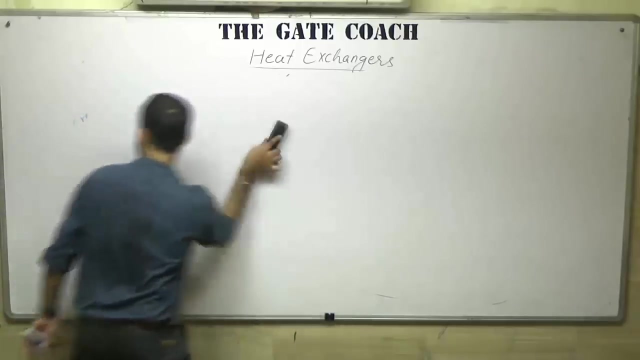 So we will use only runter pitch here. So that was about the pitch. Outer cross area- CMYR. inner cross area- CMYR plus V. Outer cross area- CMYR equal to 아니야. distance is enough, because matching is necessary. Next is the shared function. I have삭 the shell, So usually shells are made from steel, and internal diameter of the shell varies from 12 inches to 24 inches. The standard wall thickness of the shell is 3 by 8 inches. which is sufficient for. sufficient for a pressure drop up to 300 PSI. Okay, So we should have an idea that what is the pressure drop. So we should have an idea that what is the internal or external diameter of the shell, What is the approximate thickness of? 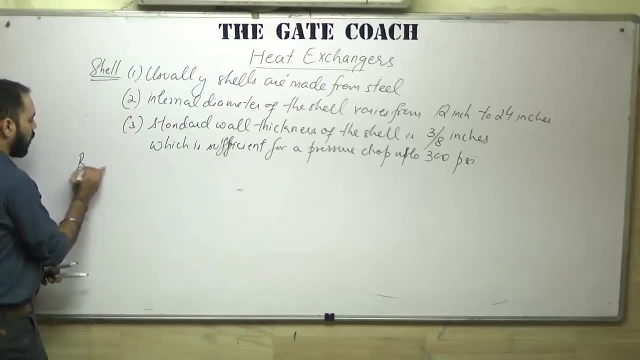 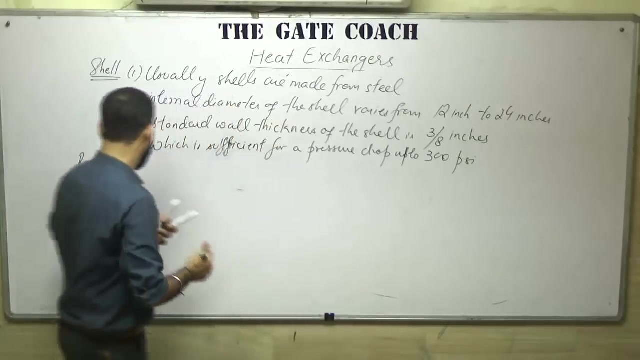 a shell. Okay, Now another term, another thing used in the heat exchanger is baffles. So it is very important that why baffles are used in the heat exchanger. Okay, What is the function of baffles? So the function of baffles is to increase the turbulence. 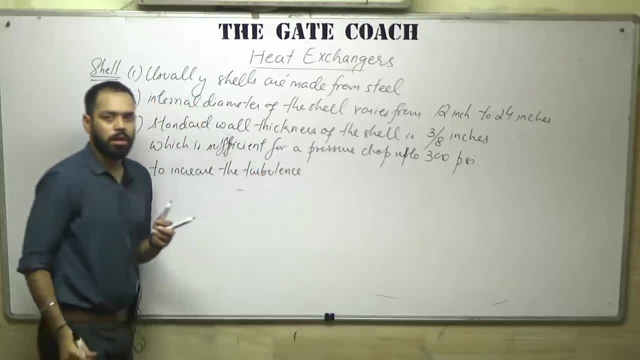 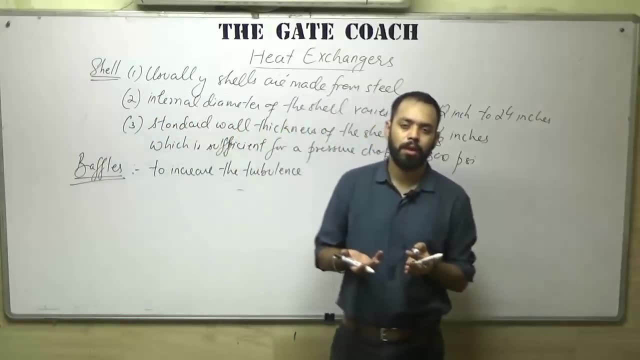 Okay, So the function of baffles is to increase the turbulence. How they increase the turbulence? Because what happens in a heat exchanger? if there is baffles, So the baffles will reduce the flow area and if you follow the equation of continuity, for the same volumetric flow. rate. the flow area is reduced, the velocity will increase The velocity of the fluid which is flowing in the shell side. Okay, to increase the turbulence on the shell side, the velocity of the fluid is going to increase. And to increase the turbulence, the velocity of the fluid is going to increase. 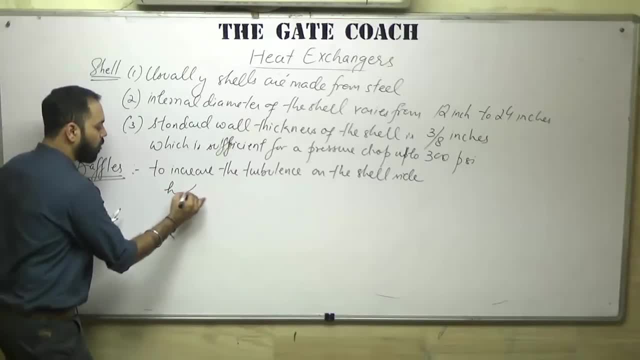 And we know that the heat transfer coefficient is always directly proportional to velocity raised, to the power, some constant, let us say 0.8.. So as the velocity of the fluid increases, the heat transfer coefficient increases, and which is always beneficial for us, okay. 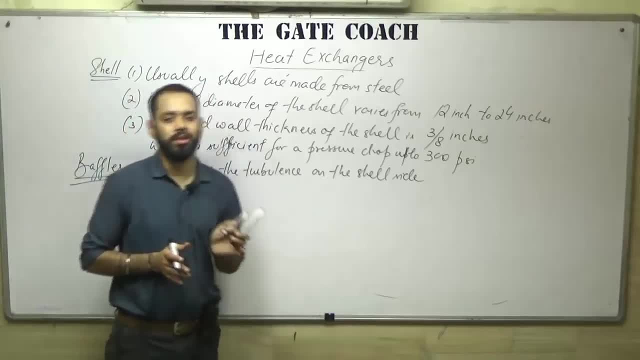 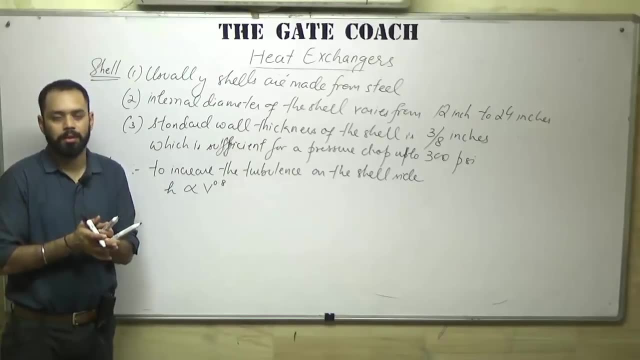 So that is the main function of the baffles: they increase the turbulence right. Also, baffles provide support to the tube bundle because the tube is a length. the length of the tube is not very small, so they have to be supported in between the exchanges. 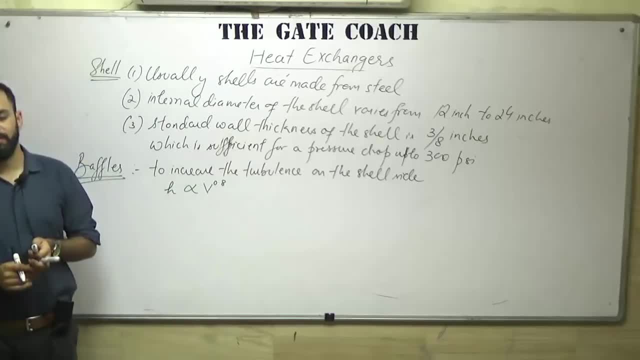 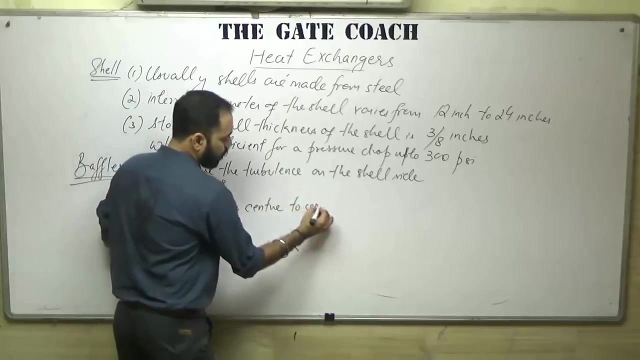 So the baffles also provide the support to the tube bundles. right Now there is a term which is called baffle pitch. What is the meaning of baffle pitch? It is the center to center distance, distance between two baffles. 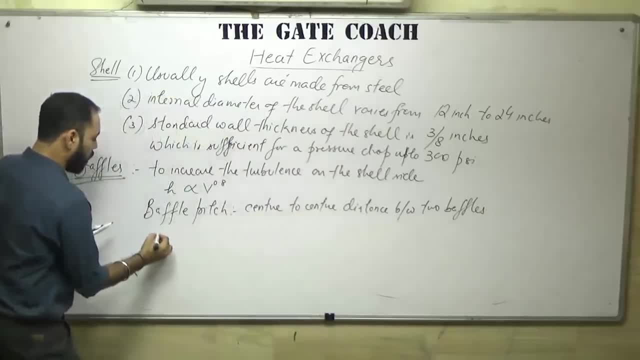 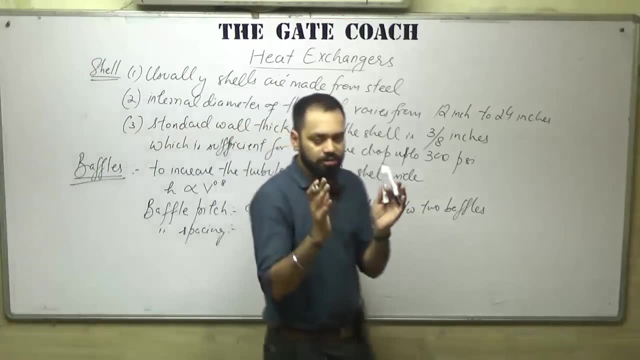 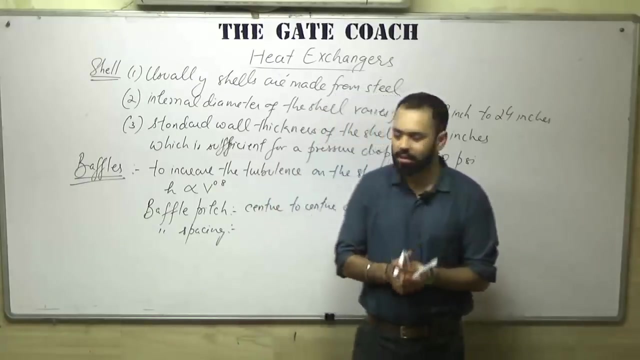 Baffle pitch is also called baffle spacing. So why the baffle spacing matters? Because if the baffle spacing is very small it is going to increase the value of pressure drop. So we cannot have very small baffle spacing. we cannot have very high baffle spacing, okay, 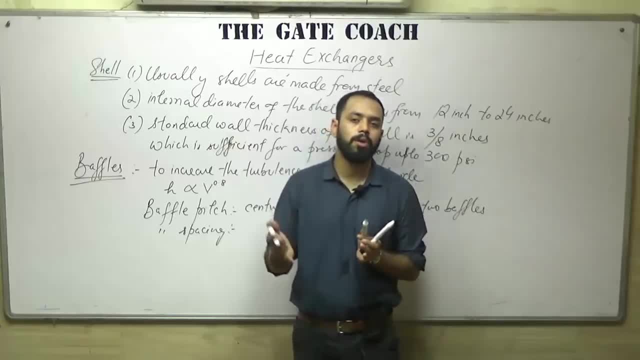 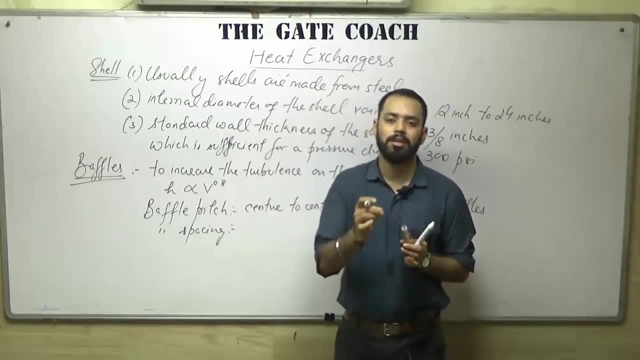 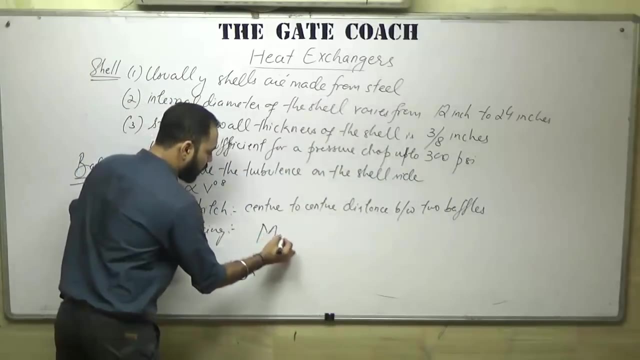 In a heat exchanger, the maximum baffle spacing is equal to the internal diameter of the shell and the minimum baffle spacing is equal to the 150.. So that we should remember that, what is the maximum baffle spacing? That is, maximum spacing is equal to the internal diameter of shell and minimum spacing is equal. 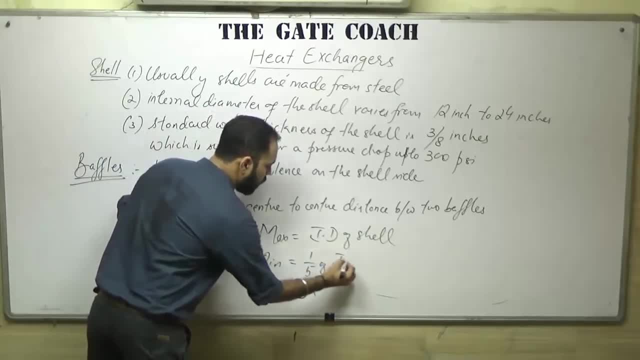 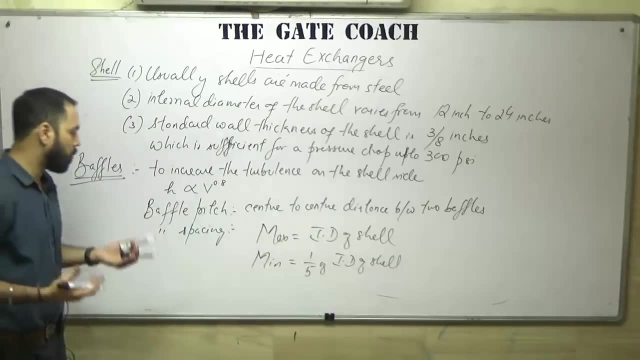 to the one-fifth of internal diameter of shell. What happens if you decrease the baffle spacing? The pressure drop increases. Again the pressure drop increases. but yes, there is a positive effect also if you are decreasing the baffle spacing. 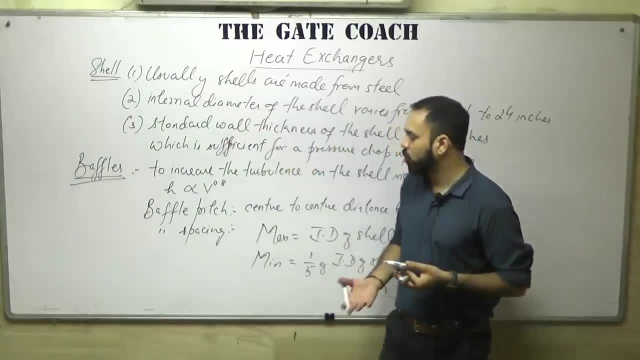 In that case the velocity will increase, which will lead to increase in the heat transfer coefficient also. okay, So there is a positive effect, there is a negative effect. okay, So that is our role, the role of the chemical engineer, that we have to optimize the process. 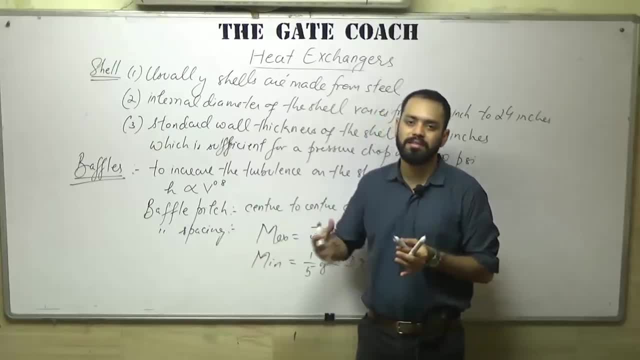 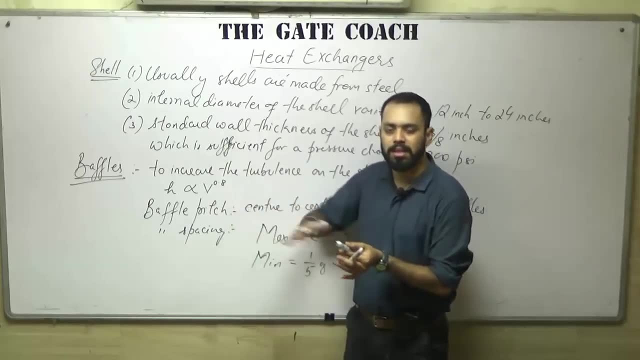 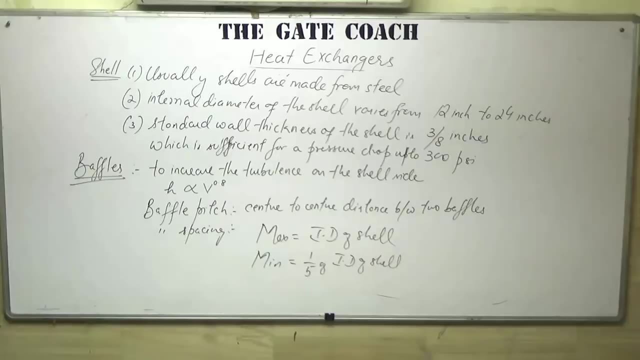 The final decision is only taken on the basis of the total cost, So that we cannot explain theoretically. okay, But we can say that if you increase baffle pitch, these are the positive effects, these are the negative effects. okay, Now, sometimes there is a question, very basic question, based on heat exchanger. that 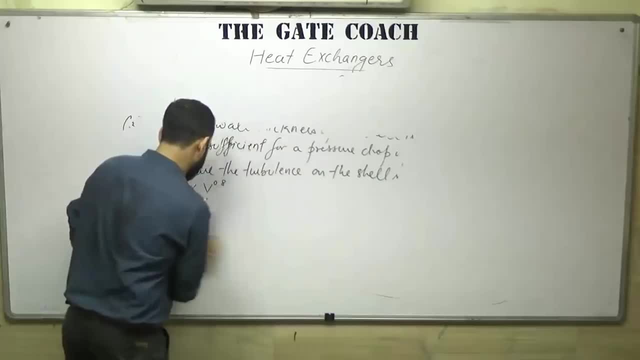 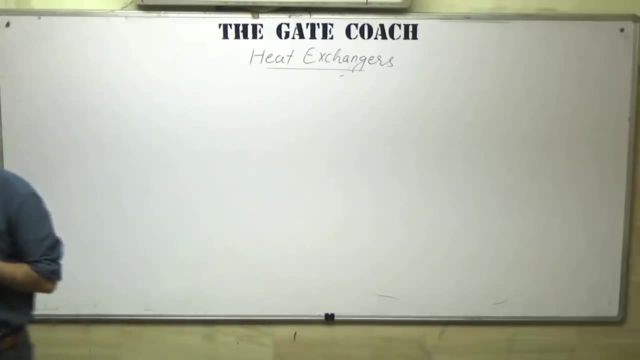 what is the advantage of using counter current heat exchangers instead of co-current heat exchanger? So the advantage is: in case of counter current, the value of delta T lm, that is, logarithmic mean of the temperature difference, is higher, which leads to reduction in the total area. 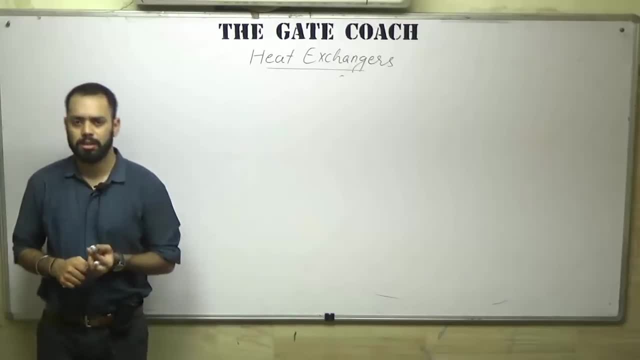 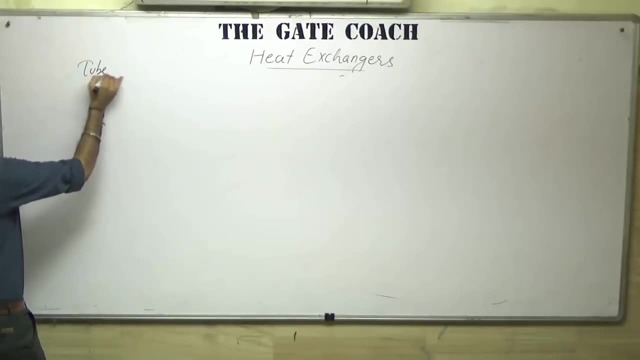 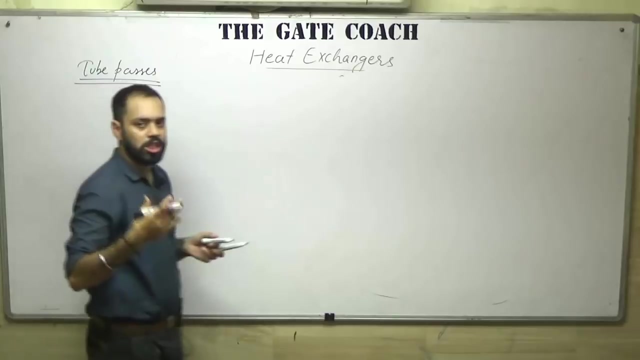 right. So that is why counter current exchangers are used. They are always beneficial, okay, economical for us, okay. Now there is another parameter, which is the tube passes. If you have heard about 1-2 shell and tube heat exchangers, so what is the meaning of? 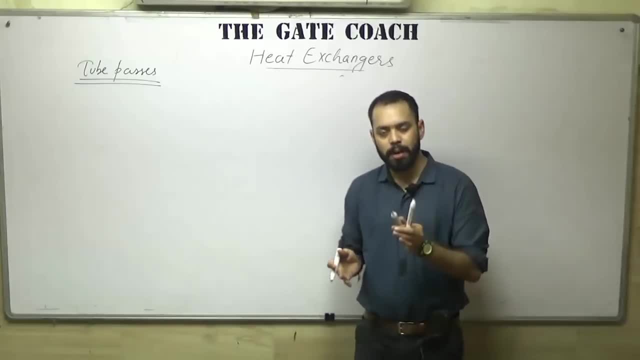 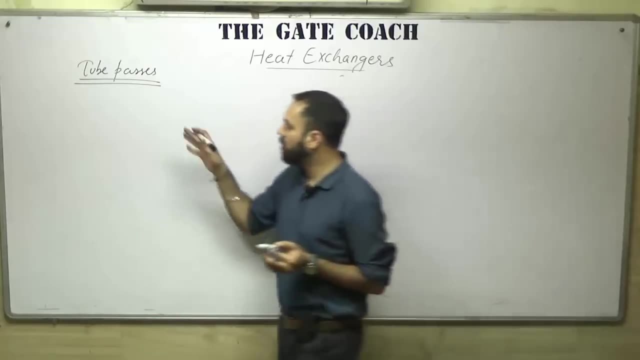 1-2 shell and tube heat exchanger. 1-2 means 1 shell pass and 2 tube passes. 2-4 means 2 shell pass and 4 tubes passes, So how this number of tube passes is increased. 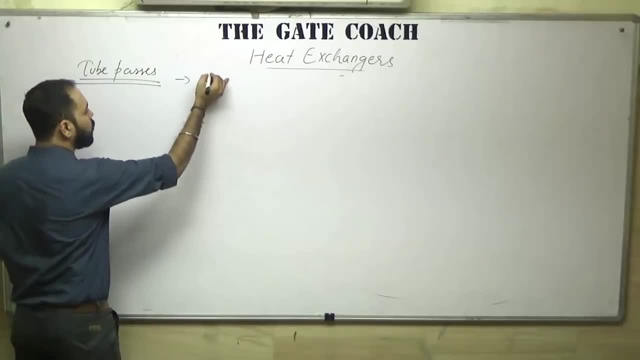 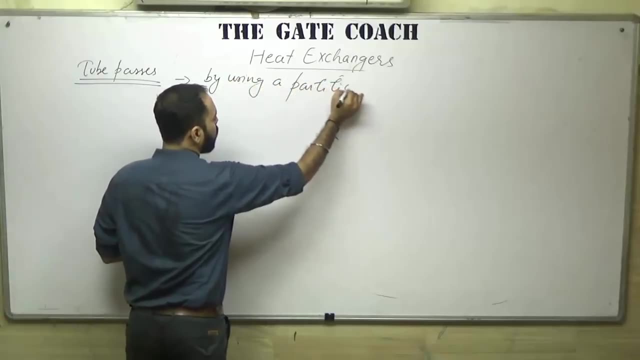 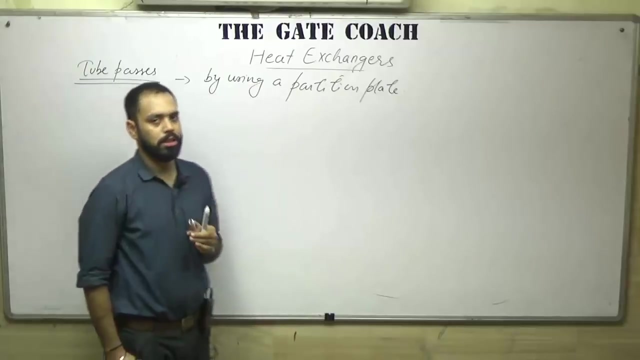 Or decreased in a heat exchanger. So that is by using- by using a partition plate, a partition plate. okay, So you can go through the detailed diagram of a heat exchanger and you can see where this partition plate is used. 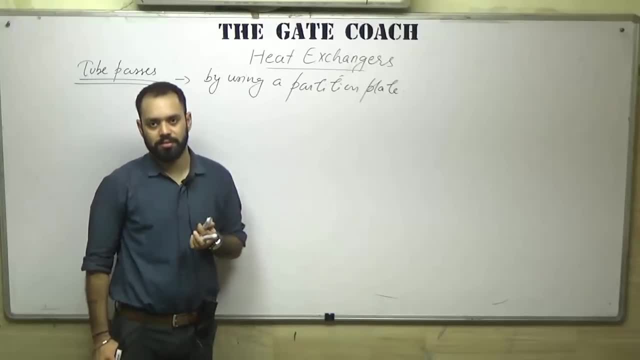 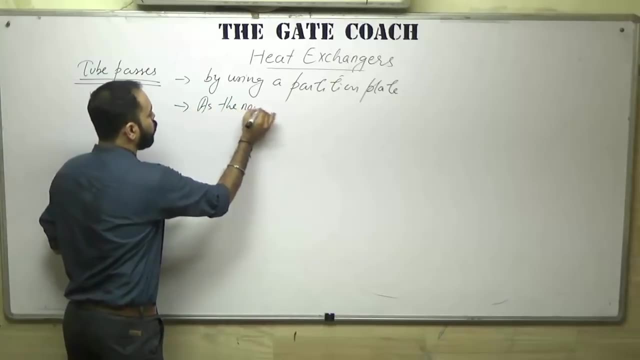 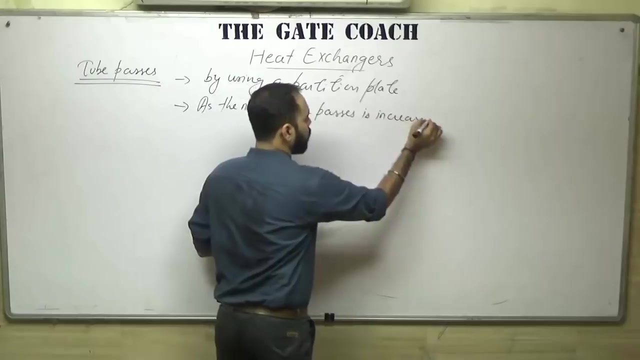 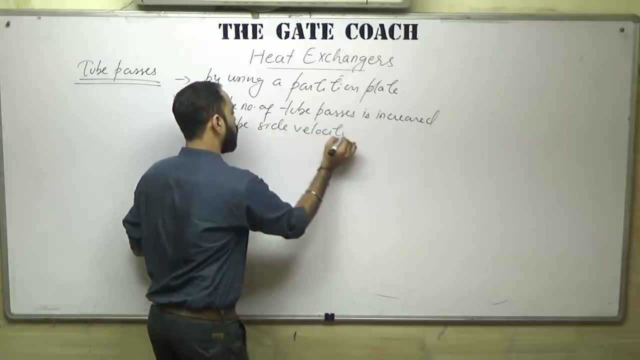 So this partition plate will increase the number of tube passes. What happens as the number of tube passes is increased? So as The number of tube passes is increased, the tube side velocity also increases. So please remember, this is a very important parameter. 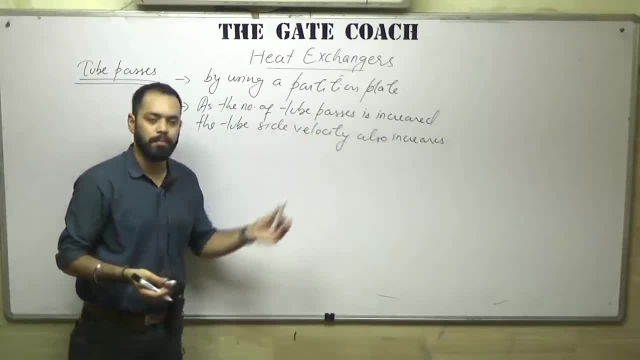 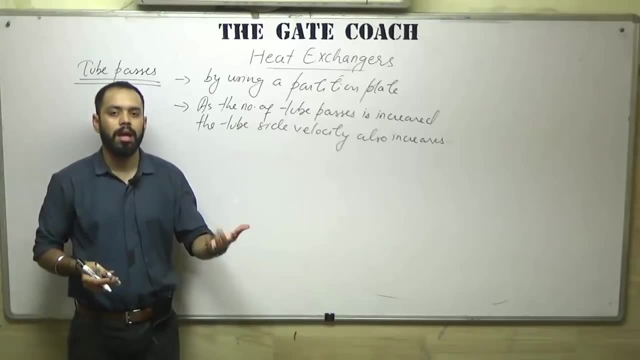 If the interviewer ask you that what is the parameter which decides the number of tube passes, So you should answer: that is the velocity of the fluid inside the tube that we have to maintain. Okay, let us suppose that we want to maintain a velocity of 1.3 meter per second. 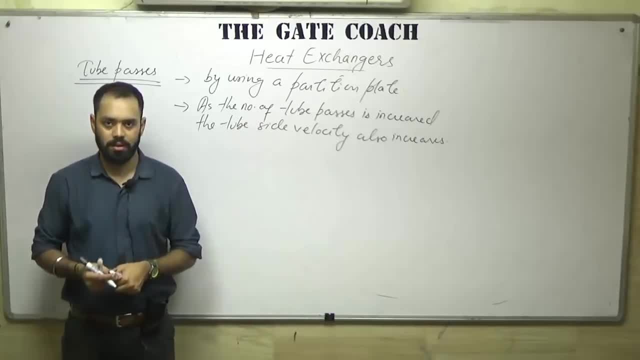 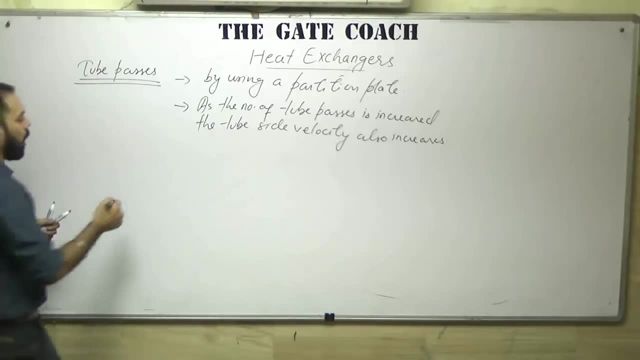 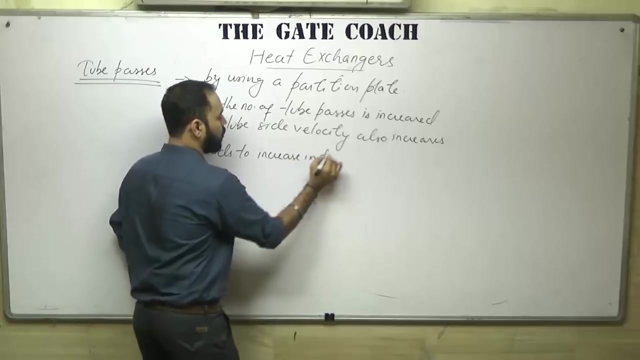 So based on that velocity we will decide the number of tube passes. okay. So as the number of tube passes is increased, the tube side velocity also increases. okay, And if the velocity increases it leads to increase in the heat transfer coefficient. 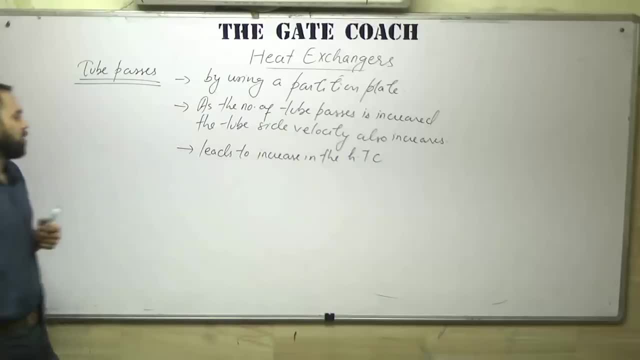 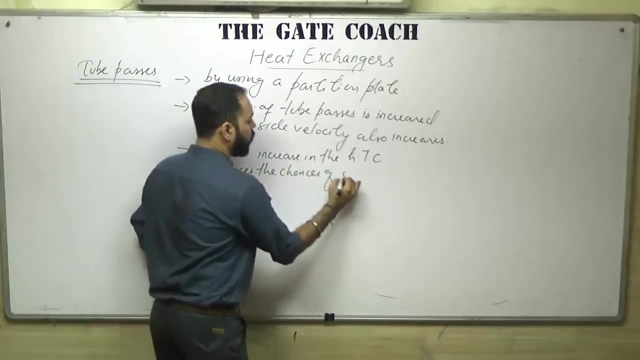 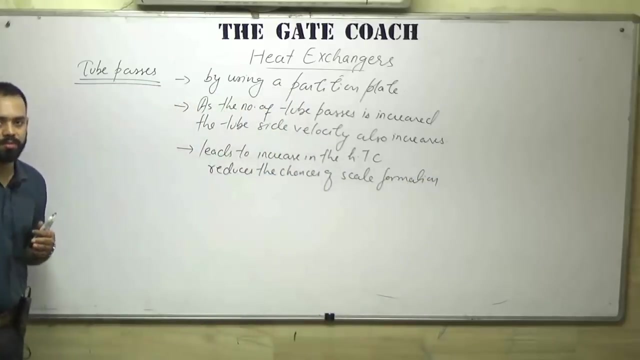 okay. And also, if the velocity increases, it reduces. So that means the chances of scale formation. if the fluid is passing at a very high speed inside the tubes, the chances of forming a scale will be reduced, okay. So this was a brief introduction about the tube passes, how it is decided, what is the 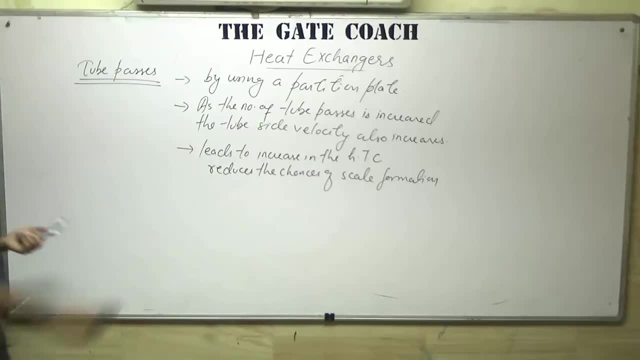 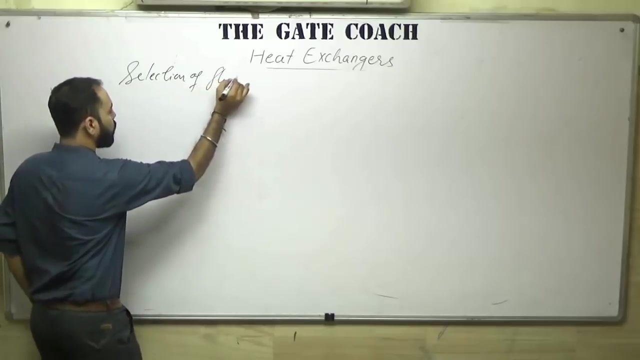 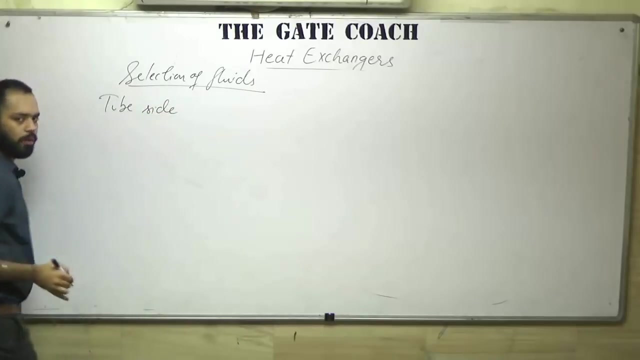 effect of increasing or decreasing. the tube passes. okay, Next is, Next is, Next is First one selection of fluids. okay, So in a tube shell and tube heat exchanger, two fluids will be there, one will be the. 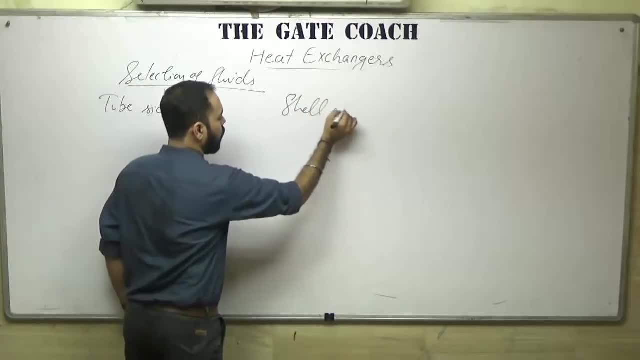 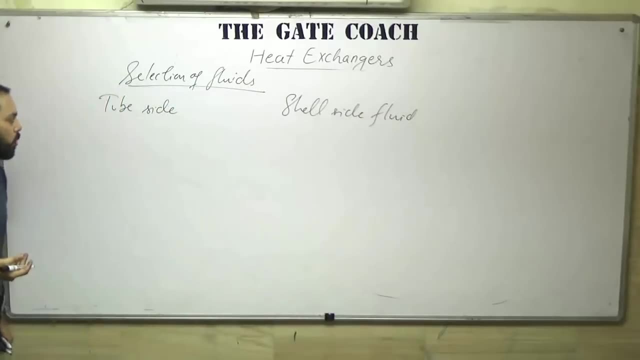 tube side fluid, other will be the shell side fluid. So there are some criterias. okay, these are the thumb rules. okay, based on the experience, that which fluid we should feed in the tube, which fluid should be present on the shell side, What are the criteria On the? 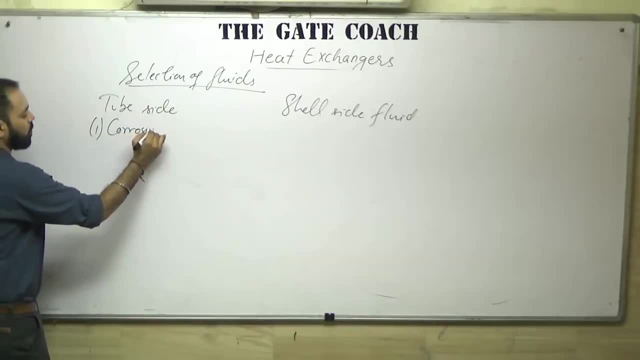 tube side, we will be using corrosive fluids. Why? Because if the fluid is corrosive, the cleaning of the tube is easier than cleaning of the shell. Also, the material of construction of shell is usually expensive. Therefore, we do not want the shell to be corroded Then after corrosive. 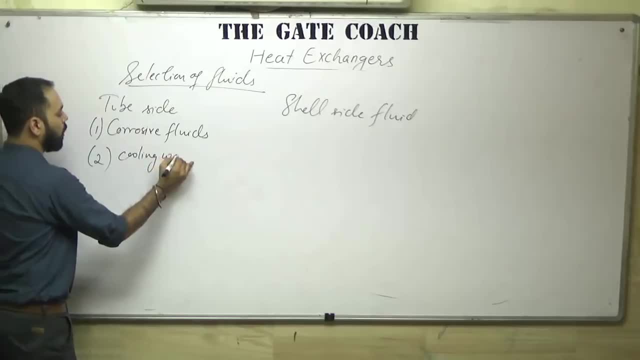 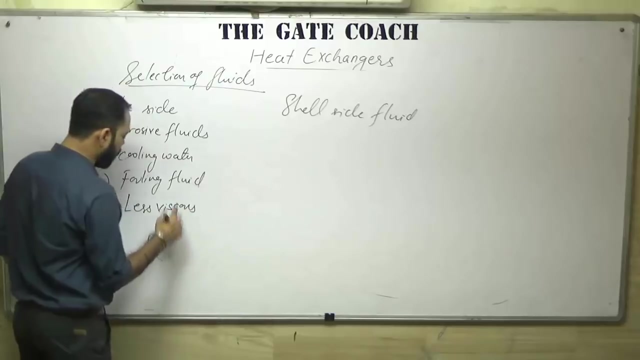 fluid. if it is cooling water, it is generally sent in the tubes. Third is fouling fluid. Fourth, the less viscous fluid, Because if it is viscosity, it will be very high. It will be difficult for the fluid to flow inside the less diameter of. 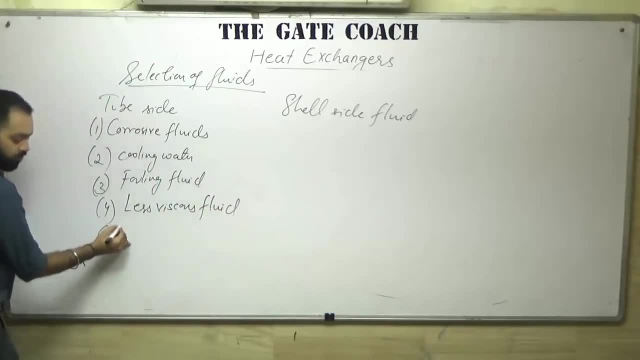 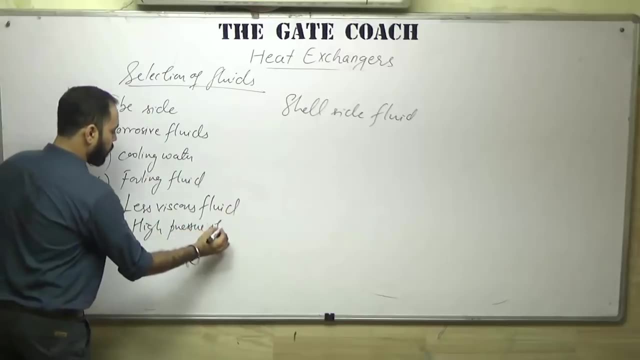 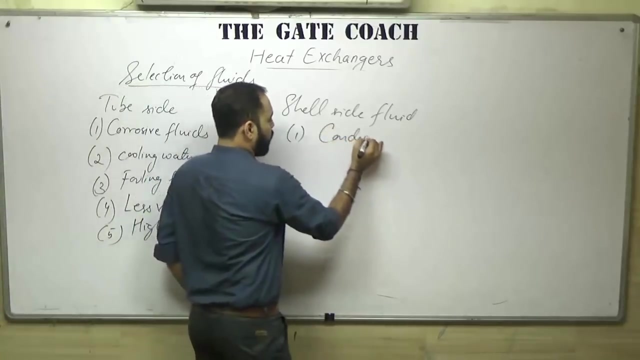 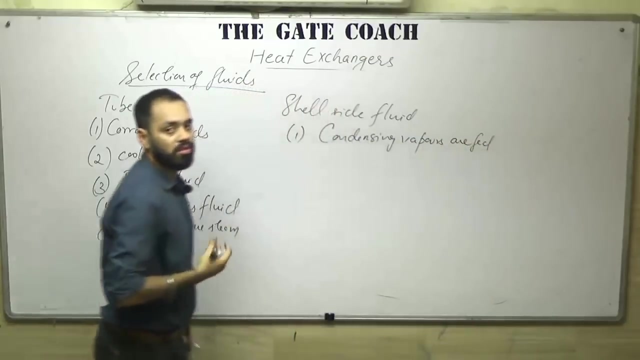 the tube. Less viscous fluid. And fifth is high pressure steam On the shell side, usually condensing vapors, are fed. Vapors are fed unless they are corrosive. If they are corrosive then it is difficult for the fluid to flow inside the tube. So less viscous fluid. 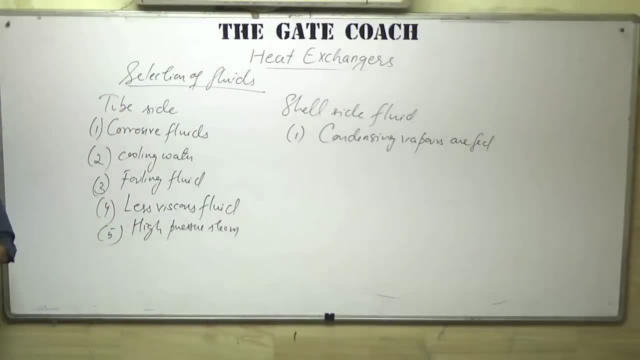 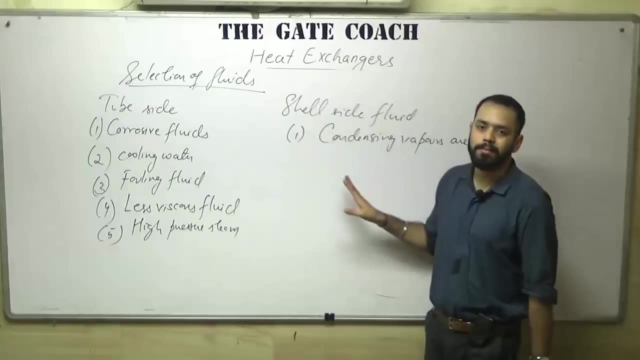 then they will be fed in the tube side. So that is about the selection of fluid. So, students, that was all from my side about the various parameters, various terms associated with the heat exchanger. that is important as far as the PSU interviews are concerned. 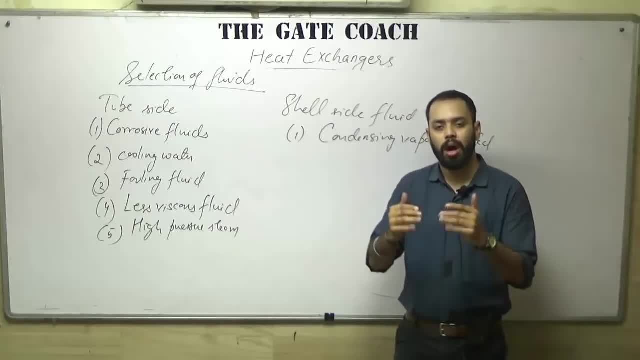 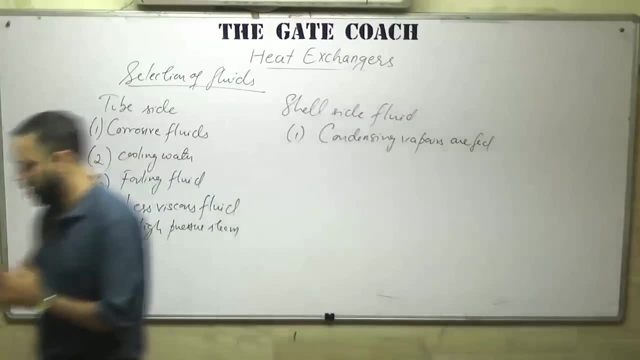 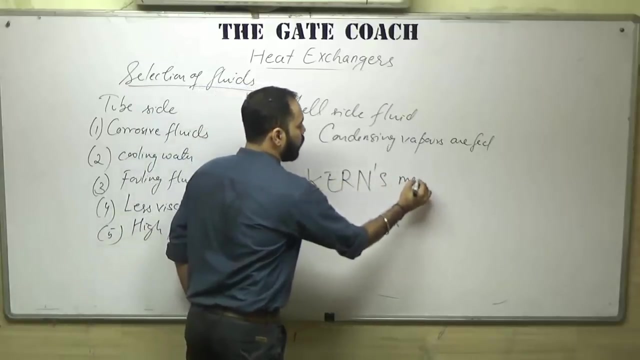 I am not discussing the formulas, the steps, how to design a heat exchanger. If you want to know, you should have a basic idea- go through the CONS method. What is CONS method? CONS method is the basic design method of heat exchangers. You can find this method in any 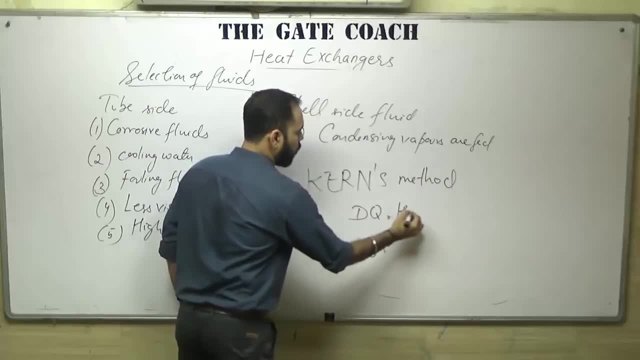 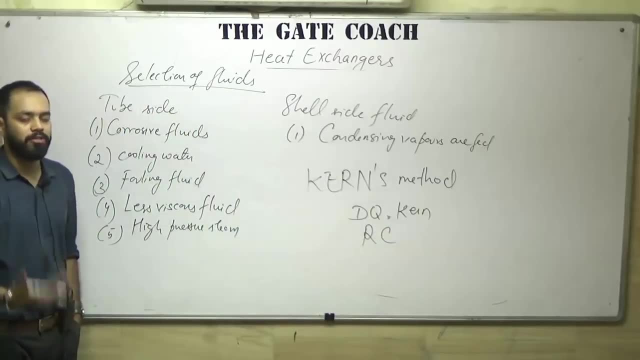 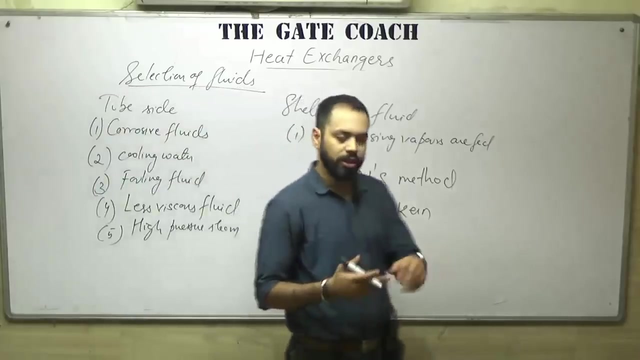 book, either in Dequecon or in Richardson-Coulson or any other book of heat transfer, You should have only little bit of idea What we do before designing the heat exchanger. the first step is calculate the heat duty: how much amount of heat has to be transferred from the hot? 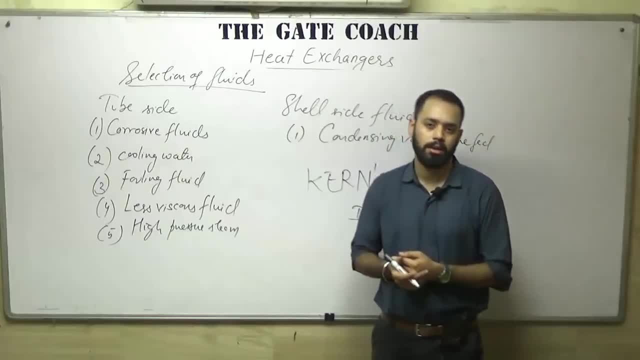 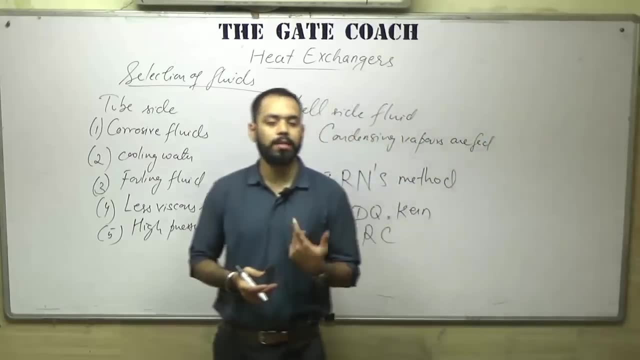 fluid to the cold fluid, or how much amount of heat has to be extracted. Okay, Right, So if you know the heat duty, the next step is calculate the delta TLM, the logarithmic mean of temperature difference. delta T, Once you calculate Q, once you calculate D, the 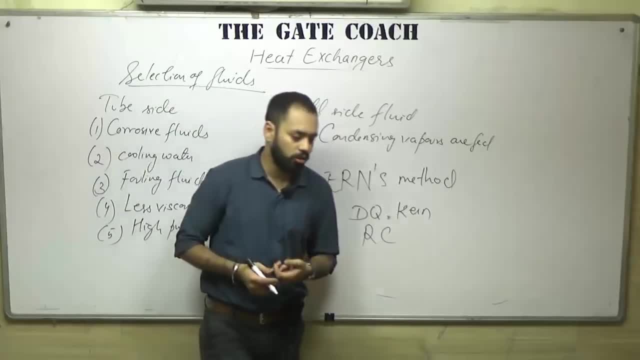 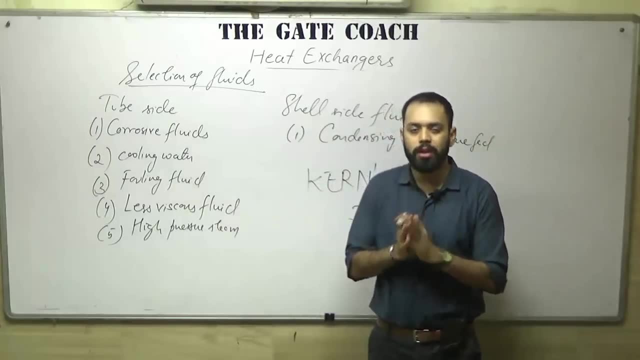 next step is: what is U, the overall heat transfer coefficient? Now the calculation of U is a hidden trial method. That is why I am not explaining these things here. You have to assume the value of U from the literature Based on that U by using the formula Q is. 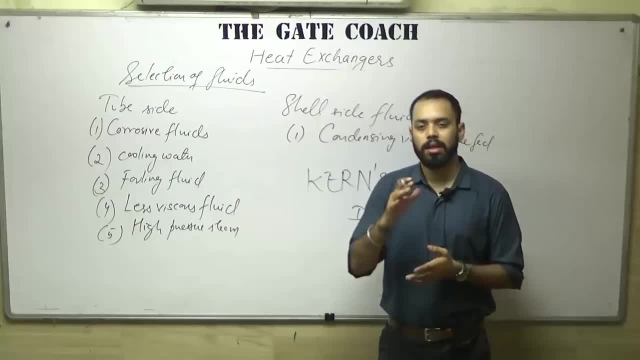 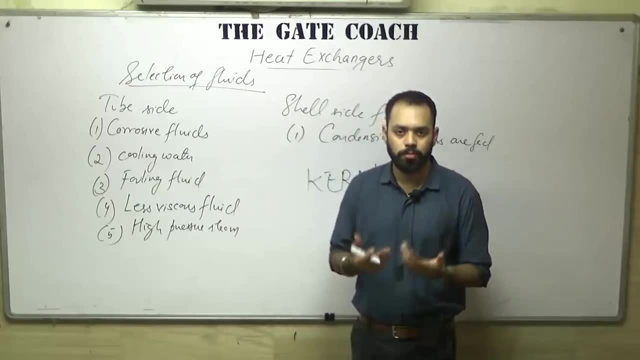 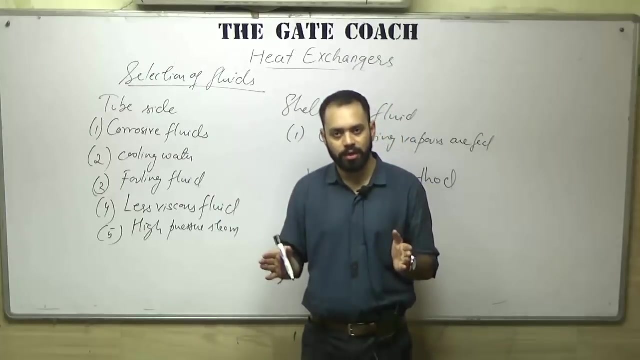 equal to UA delta TLM. You are going to calculate the area which is required for heat transfer Once you know the area. now we will assume that what is the standard tubes I am using for heat transfer? The length of the tube is fixed. The diameter of the tube is fixed. Now we know that how?